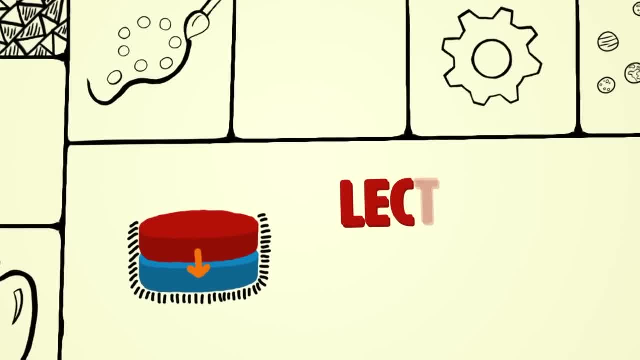 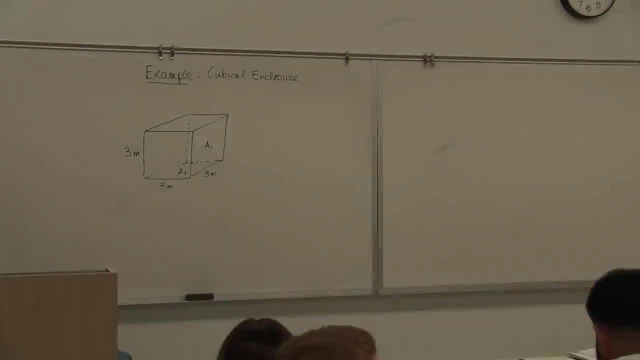 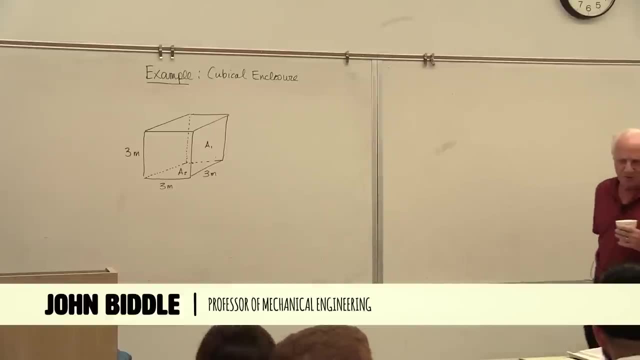 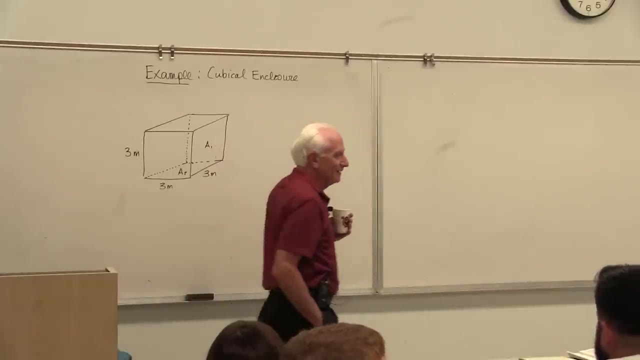 Okay, so, just so you know. oh yeah, okay, Blackboard. Blackboard website. it's got the notes for chapters 12 and 13 right now on there, but it will also have two practice exams Sunday night, 1159, you know. So two practice midterms, for the second midterm will be on there. 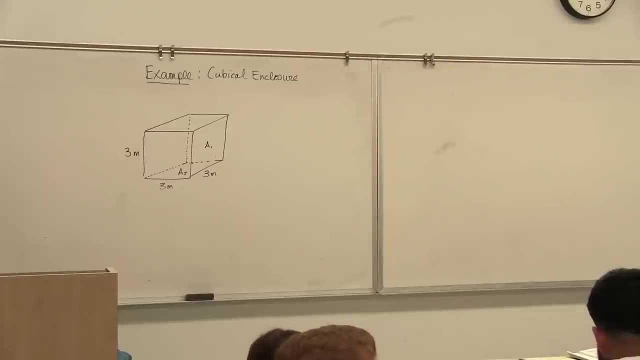 They were ones given last year, the second midterm given last year, So that'll be on there Sunday night late. Okay, now a quick review where we were in chapter 13. We had finished the first part of chapter 13, which allowed us to calculate the view factors in a radiation- thermal radiation. 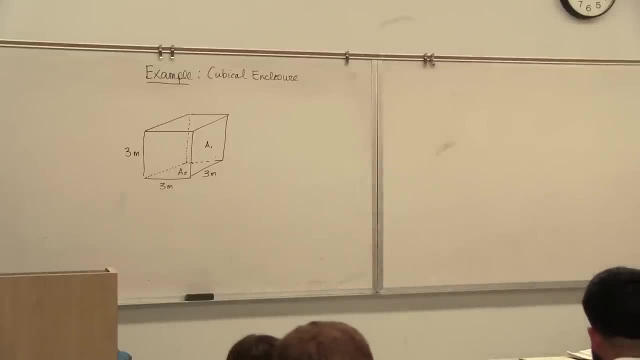 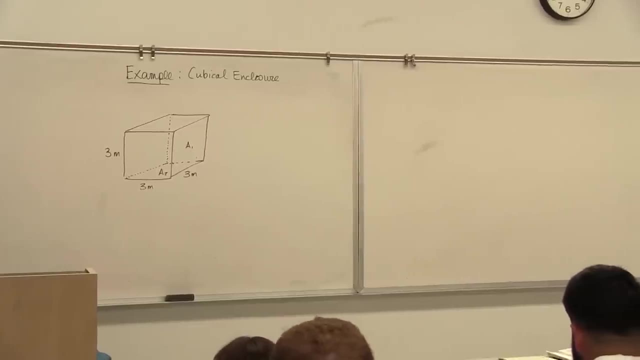 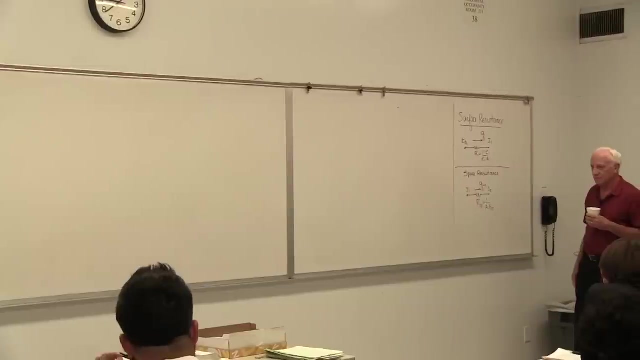 problem the view factors. The second part of chapter 13 talks about how we actually do some heat transfer calculations in an enclosure with thermal radiation And we went through the derivation for two kinds of resistances in these problems. One is called a surface resistance. 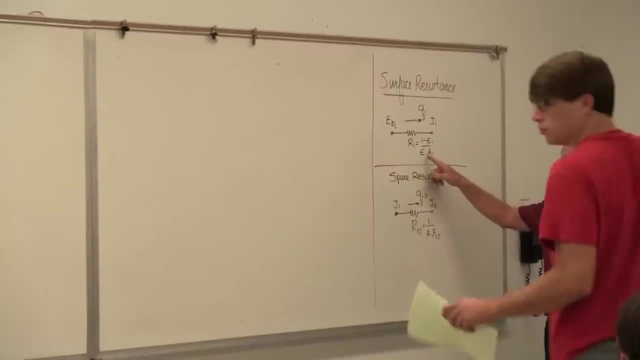 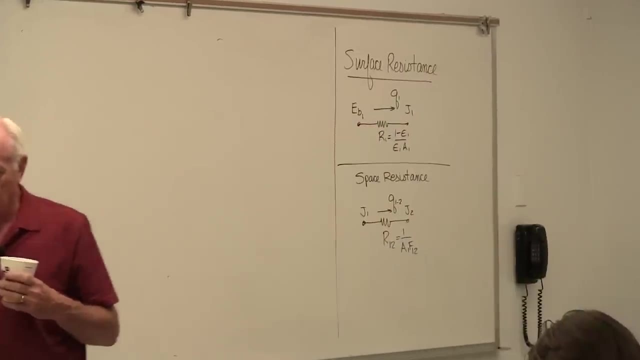 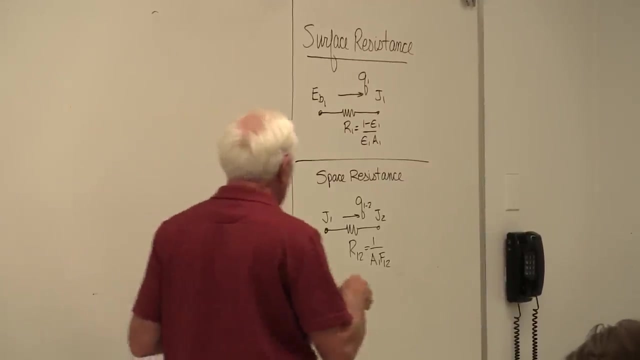 Its value is one minus the emissivity of the surface divided by the emissivity times the area of the surface, And there's a little model of it right there. Every surface in an enclosure has a surface. Then there's a second kind of resistance, called a space resistance, because it depends on the 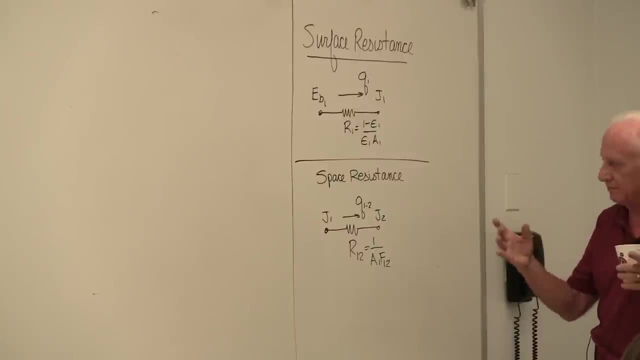 space between two surfaces and their orientation and their geometry. Its value is one over A1F12.. And here's the picture that shows where that resistance is located: between nodes J1 and J2.. J is the radiosity of the surface. The radiosity J is what leaves the surface, The emitted radiation plus the 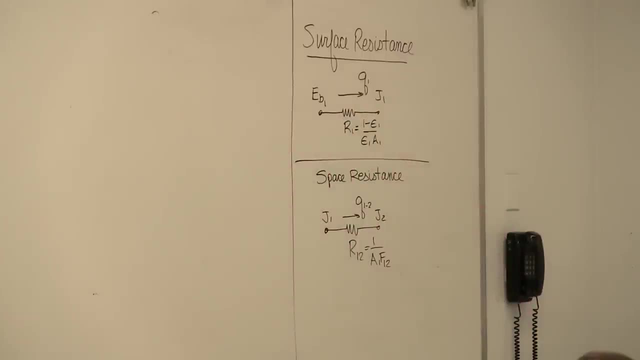 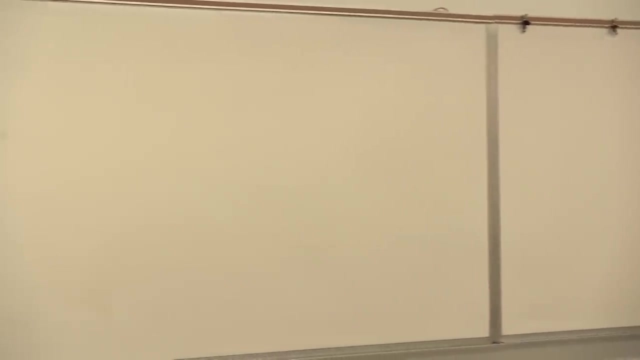 reflected radiation. Okay, So we're looking at enclosures And we're trying to find the heat exchange between surfaces in an enclosure. We're going to look at a specific example. It's a cubicle enclosure. Surface A1 is the right-hand side, right-hand wall, the bottom. 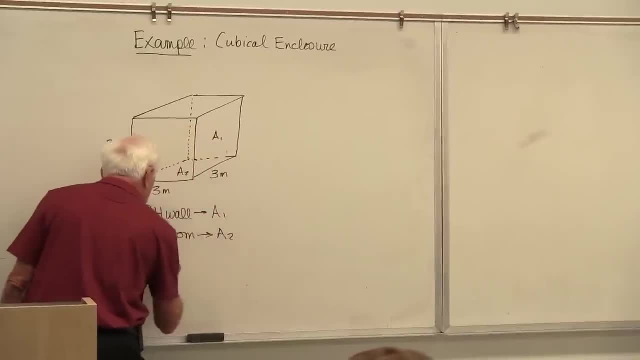 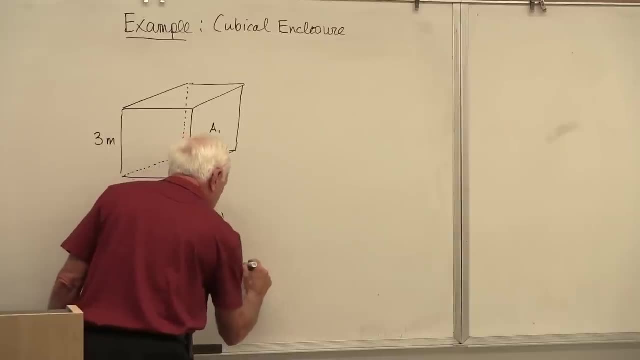 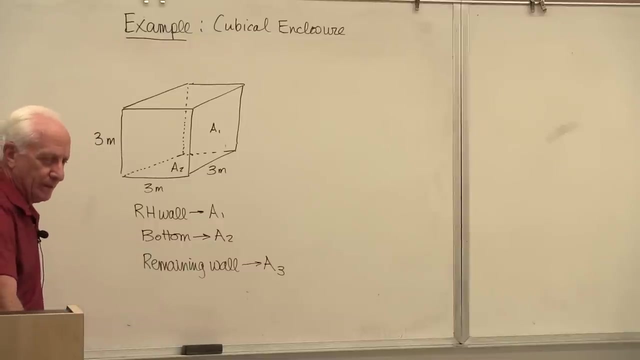 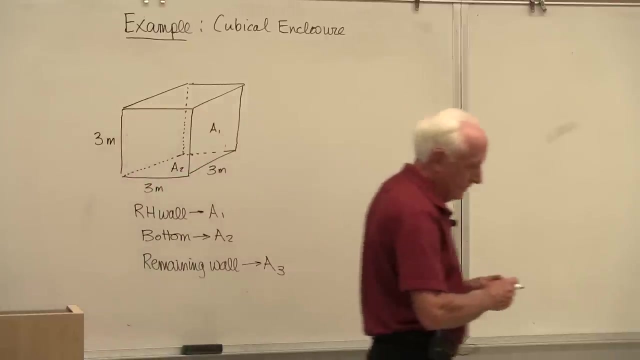 Surface A2 is A2. And the remaining walls are A3. So we call that a three-surface enclosure because we're going to say the temperature of wall three is constant, It's given. So I'll put down what those temperatures are. 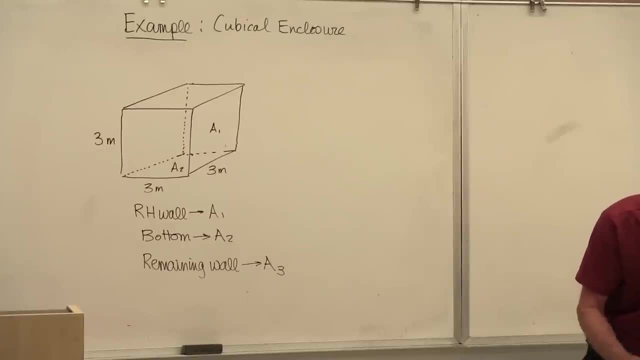 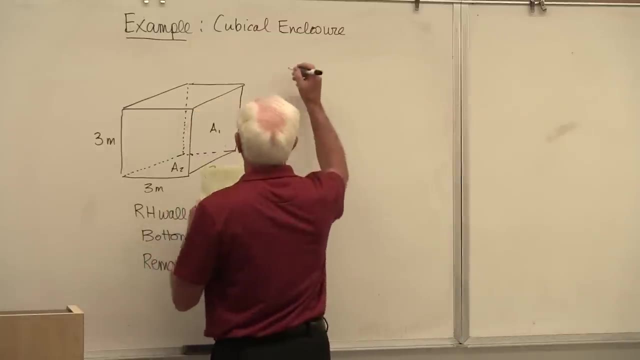 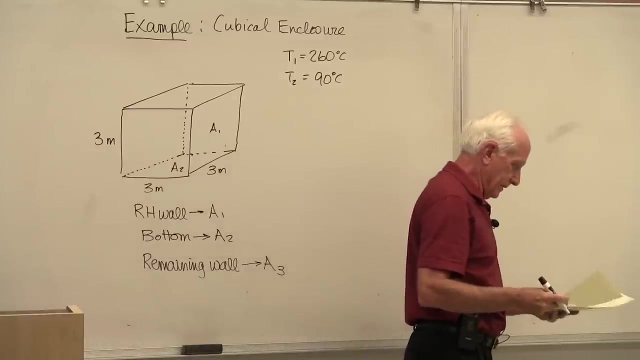 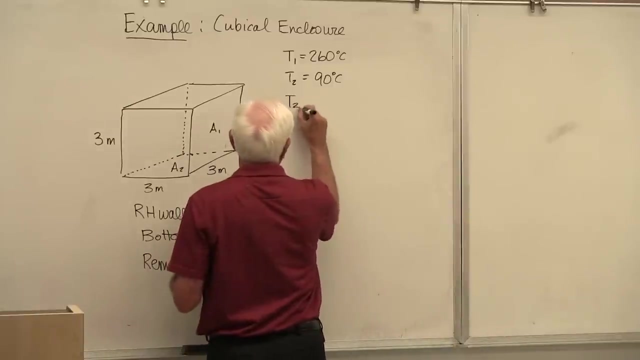 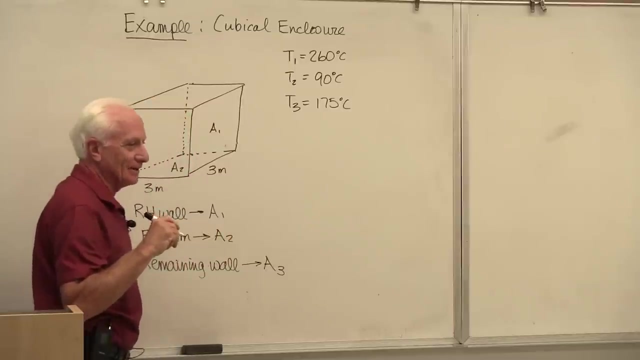 So assume that we're given the temperatures In the enclosure. let's put down what we have here: T1 is 260 C, T2, 90 degrees C And T3 is 175 degrees C. Okay, We're going to go from the simple to the complex. So we're going to say to start off with: let's let all those 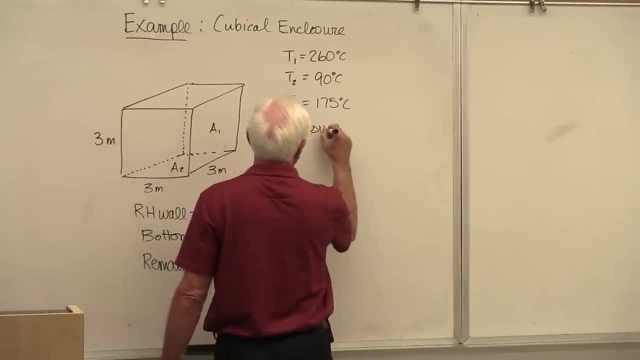 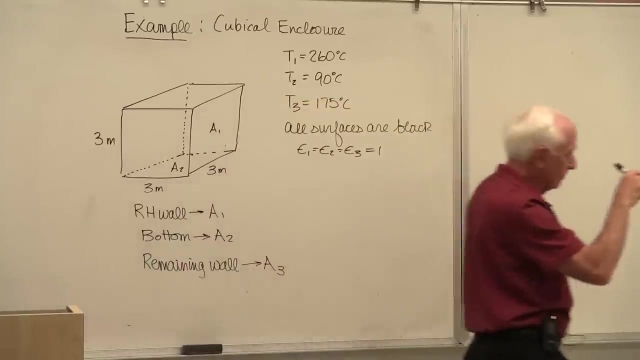 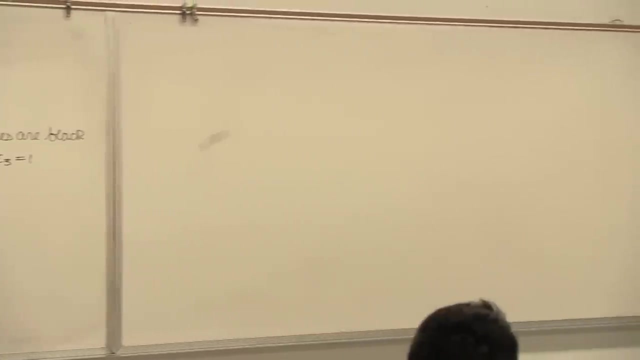 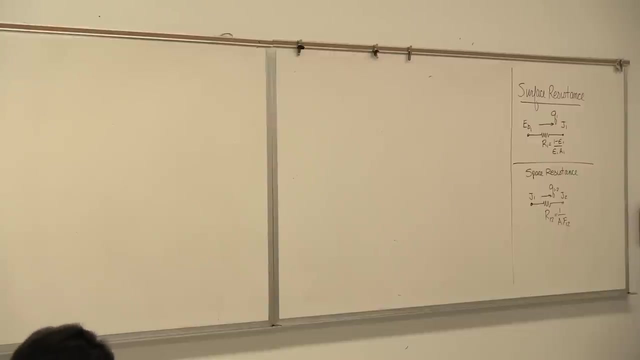 surfaces be black. So epsilon 1 equals, epsilon 2 equals, epsilon 3 equals 1.. If the surfaces are black, you go over here and you put epsilon equal to 1.. The resistance: The resistance is 1 minus 1, 0.. So now we know R1, R2, and R3, 0. 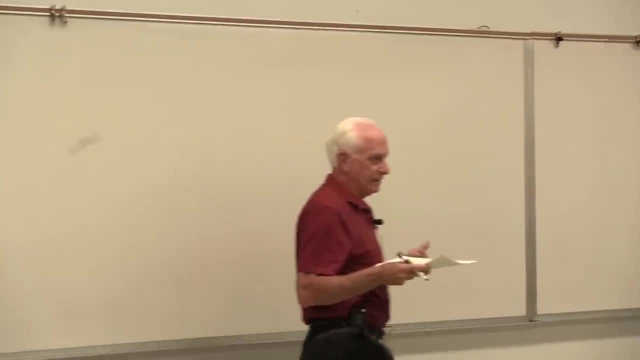 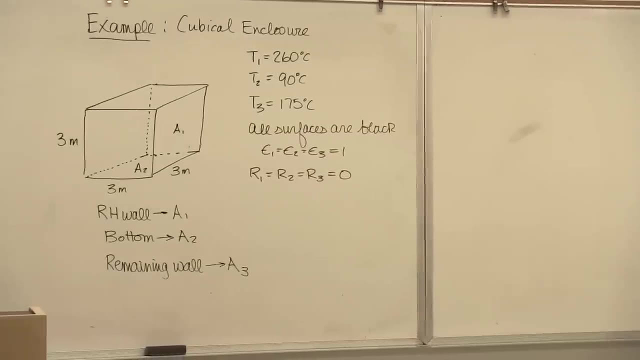 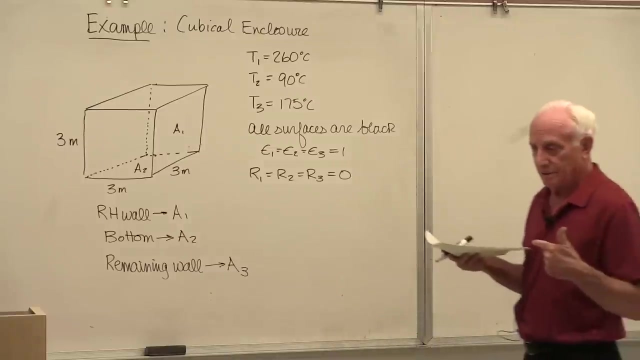 Don't forget that surface resistance tells you how easy it is for heat to escape from the surface by emission, How easy it is for heat to escape the surface by emission, And a black body or a black surface is the best possible emitter. So obviously a black surface has a low resistance because a lot of heat gets out. 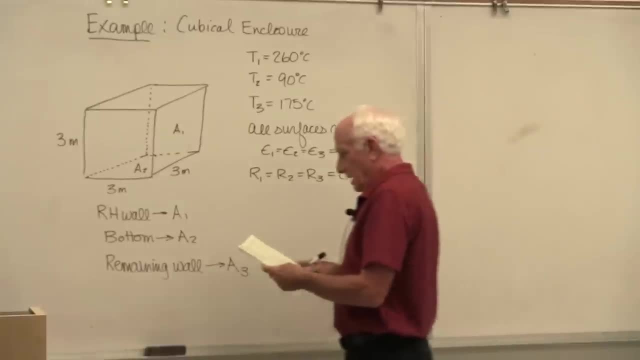 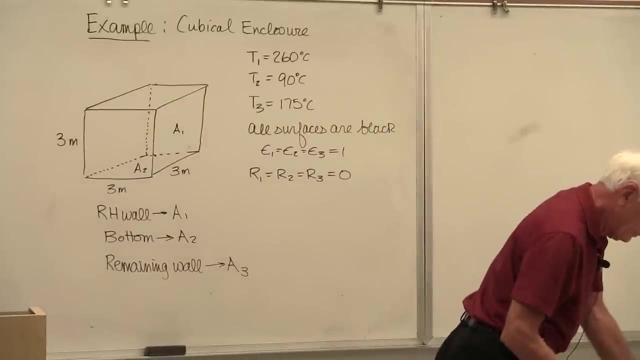 Okay, Back over here Let's see what else we might need. I think that pretty much covers that, So we're going to draw the circuit, But I'll just remind you first. the last time we met, we looked at this configuration. 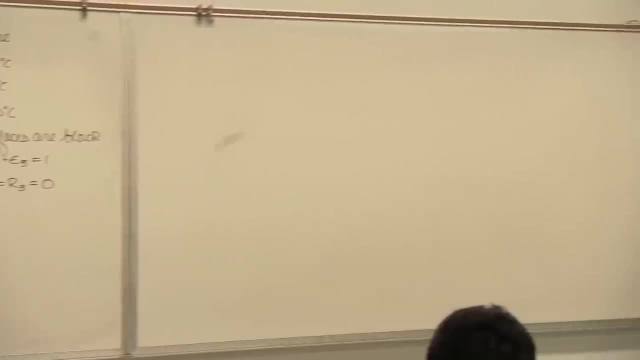 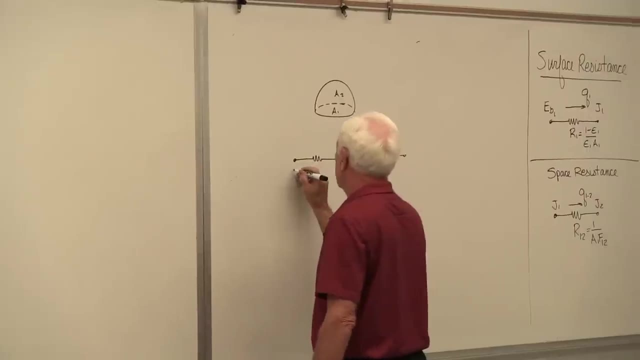 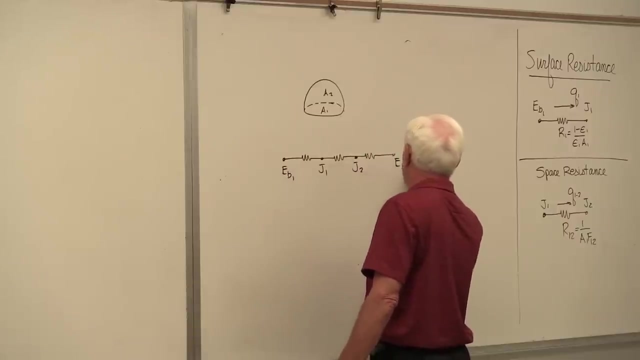 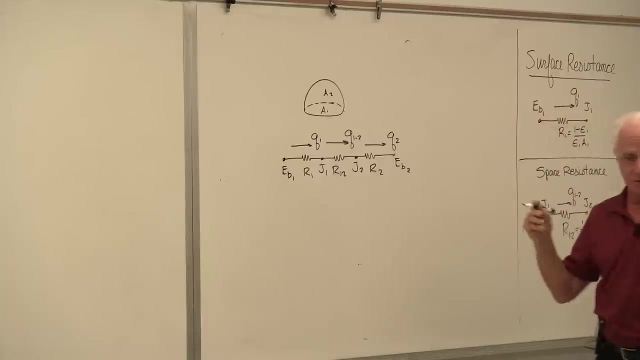 And this was A1 and this was A2, and the resistor model for that looked like this And we found it. It's a series. It's a series: Two surfaces in closure. They're all in series. 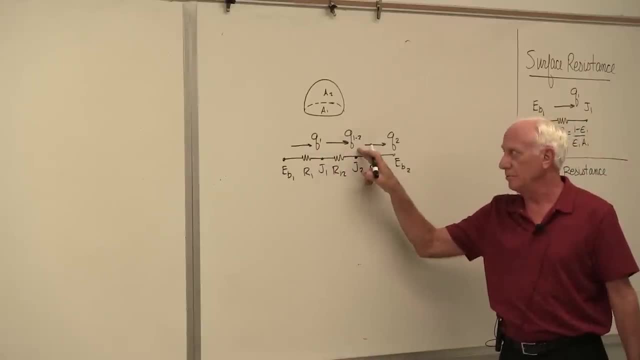 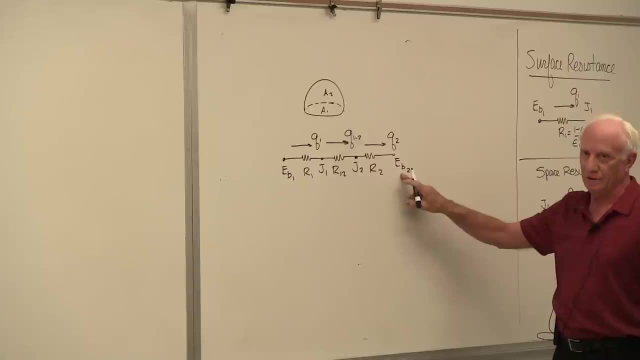 And if you want to find the Q, since all of the Qs are the same in series: Q1 equals Q12, equals Q2.. The way you find the Q is you take m minus e-B2, which you know the temperatures are given. 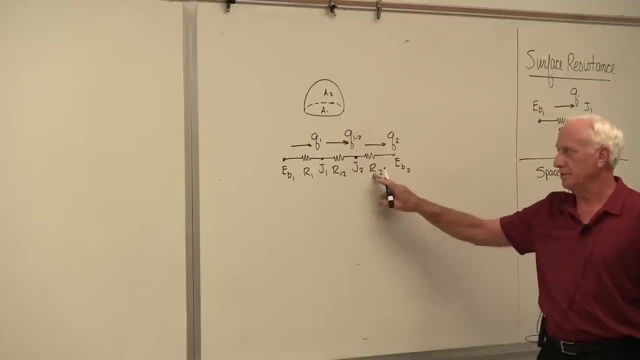 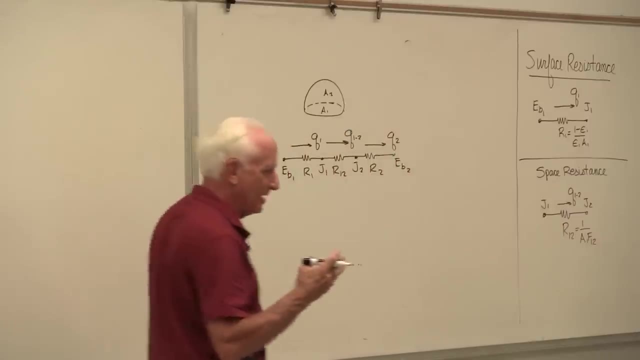 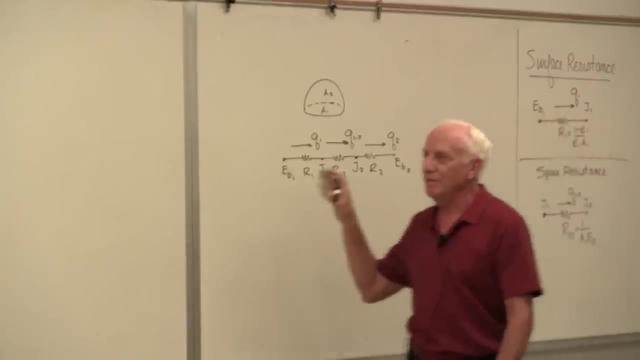 divided by R1 plus R12 plus R2.. And now you've got Q And a problem: you can find the Js. They're not important to find the Js Normally in thermal analysis. we want to find the Qs. So that's how you find the Qs. Now we make life a little more. 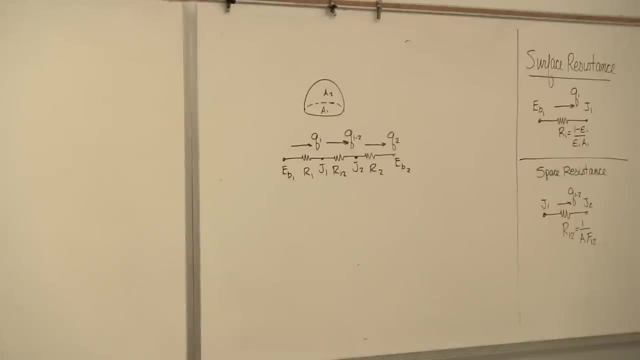 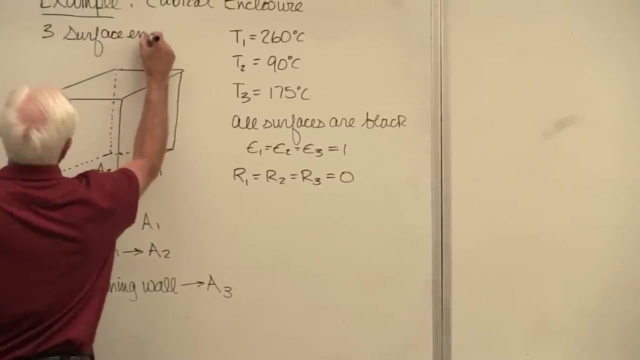 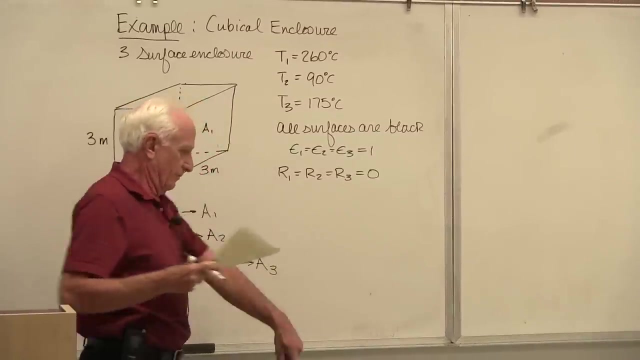 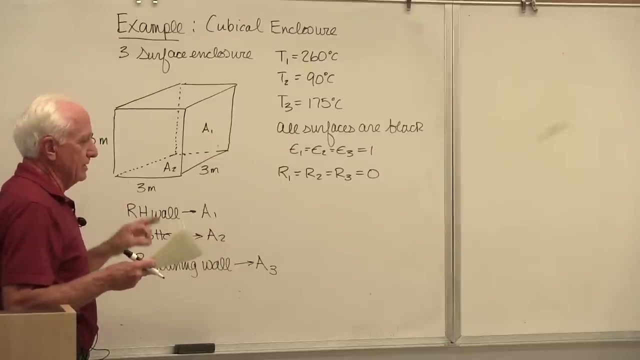 difficult. That's a two-surface enclosure. This is a three-surface enclosure. Okay, It could be this room, The front wall's area A1.. The floor is A2.. And the other walls and the ceiling are combined A3.. The reason why we can call them by one nodal designation: 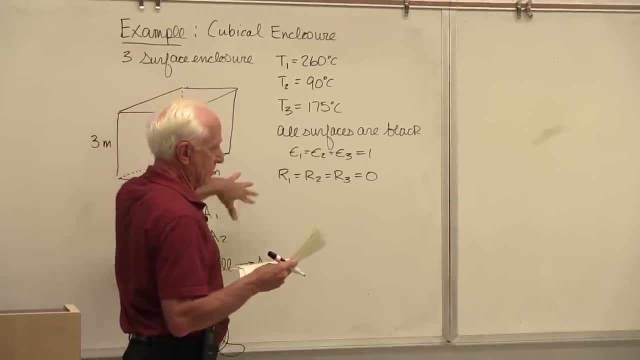 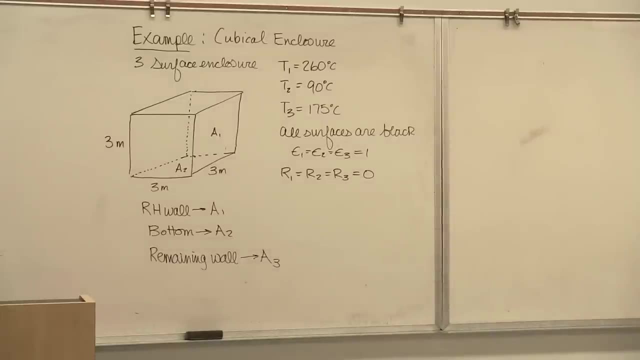 is because they all have the same temperature and they're touching each other. Okay, So draw a thermal circuit like this. But now, rather than two, you've got three nodes. They're all black. Okay, One, two, three, four, five, six, seven, eight, nine, 10,, 11,, 12,, 13,, 14,. 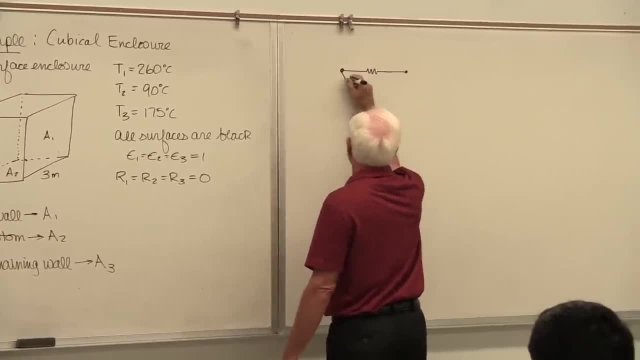 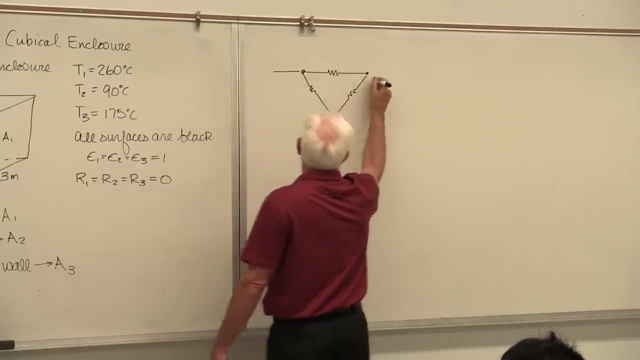 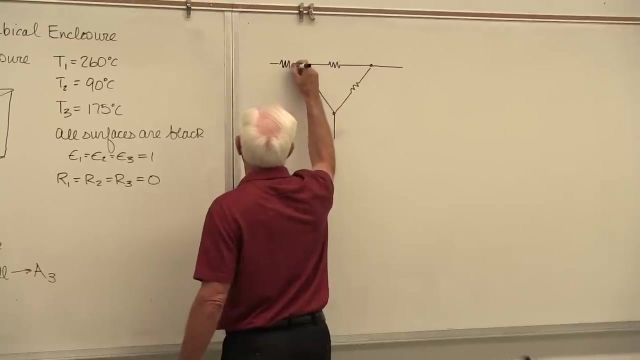 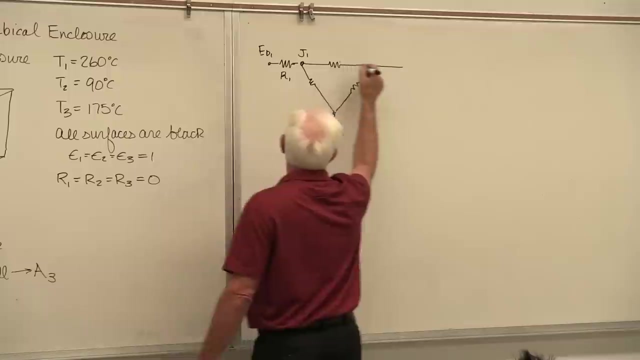 15,, 16,, 17,, 18,, 19,, 20,, 21,, 22, 23.. There are the three nodes. Now I'll put them here and I'll set them equal to zero, But for right now that's R1.. This is EB1, J1, J2, R2, R3,. 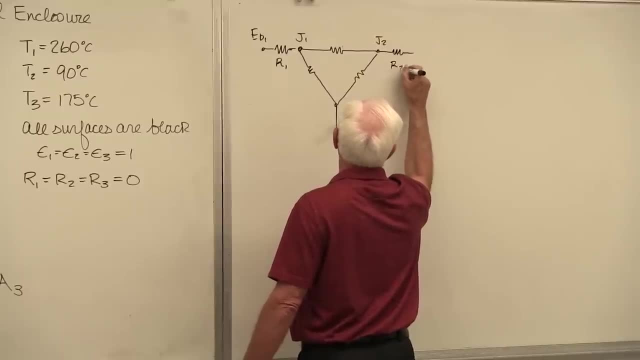 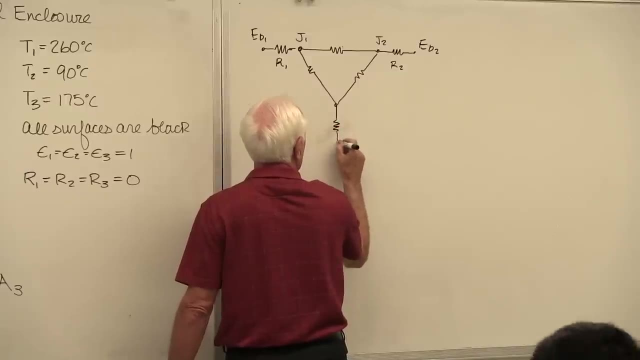 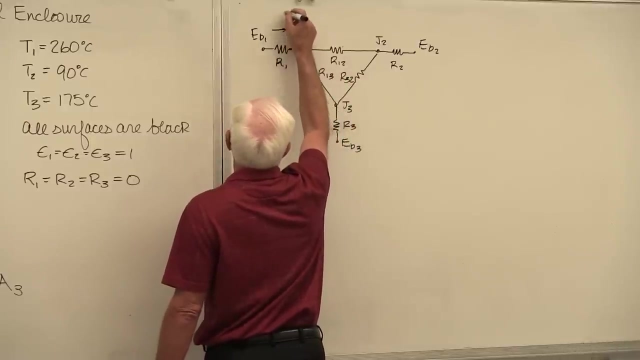 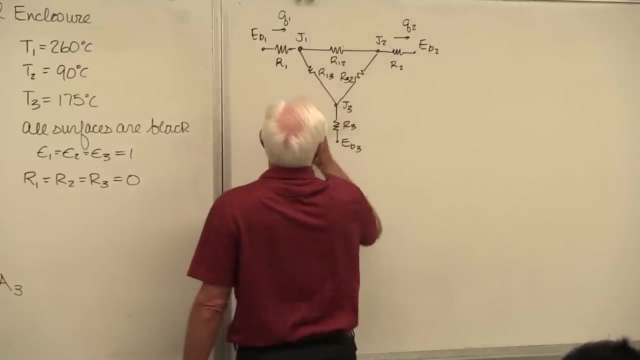 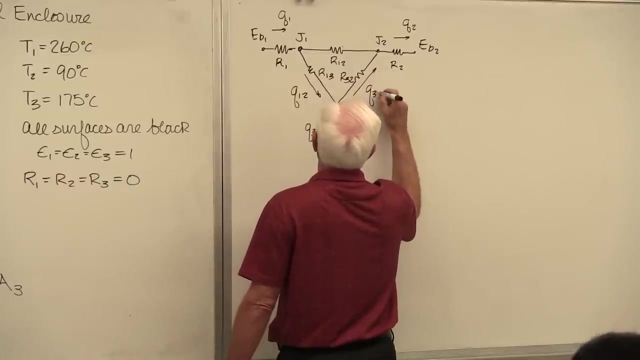 we'll make it the big problem and then we'll reduce it to a smaller problem: J3, R3, 1, 2, 1, 3,, 3, 2.. Q1, Q2,, Q3,, Q1, 2, Q3, 2, should be 1, 3, and this is Q1, 2.. 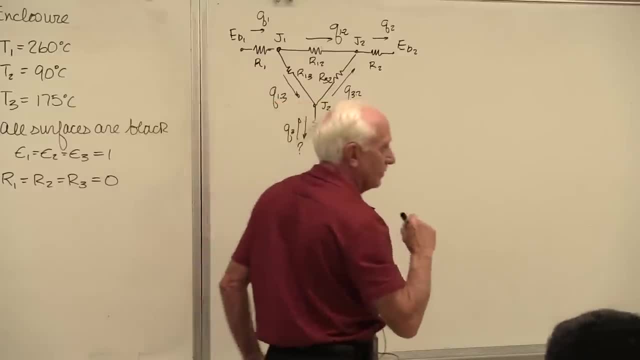 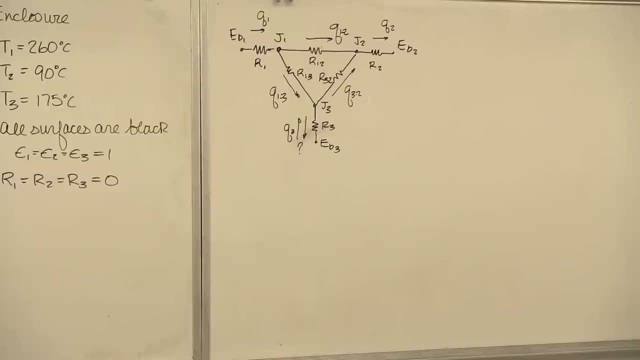 Q2, Q3, Q3, 2, 3, 2, 3, 2.. Okay, So there's the full-blown three surface enclosure. Anytime there's three surfaces. that's how the. that's how you set the little circuit up the thermal. 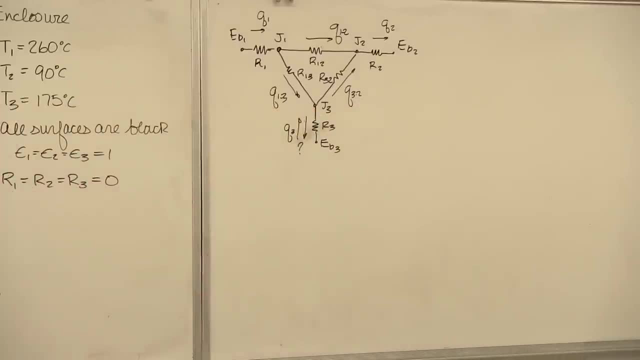 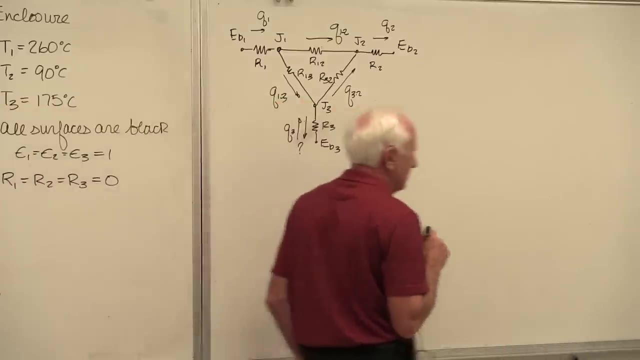 circuit up. Everything is labeled. Every node is labeled Js and EBs. Every resistor is labeled. Every heat flow is labeled. How many heat flows are there? Six, Unknown Js, three, Okay, Okay, Okay, Now we'll take the. we don't, I know, since surface one is the hottest and surface. 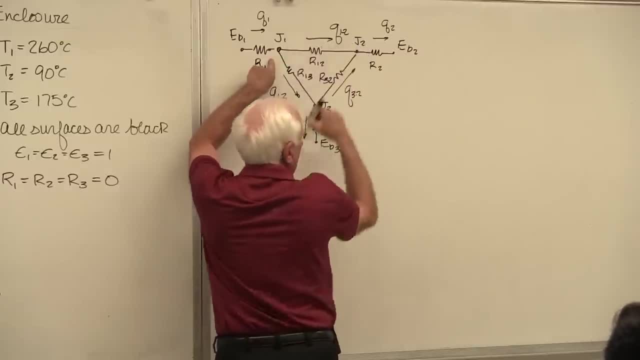 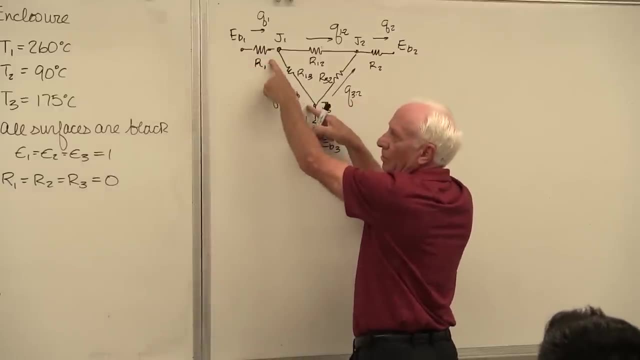 two is the coldest. I know heat goes from one to two, of course, going from hot to cold. I know that since one is hot and three is colder- 1,, 2,, 60,, 3,, 175, heat goes down. that. 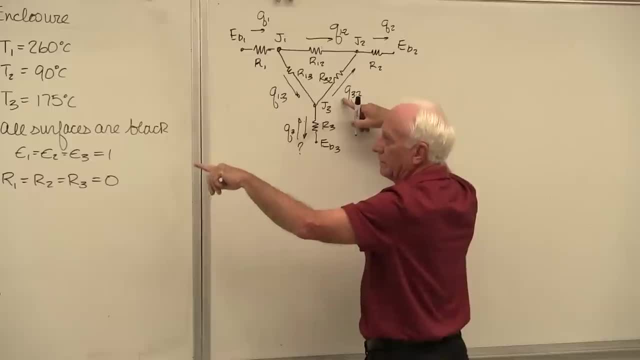 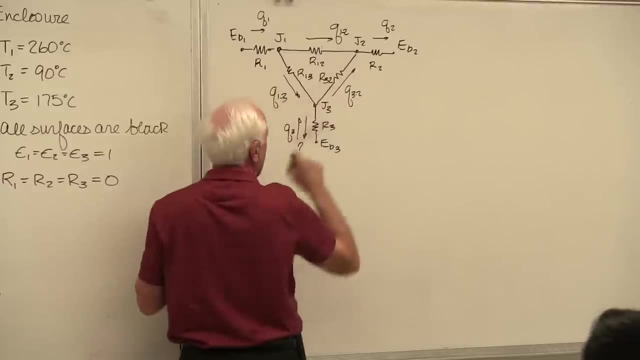 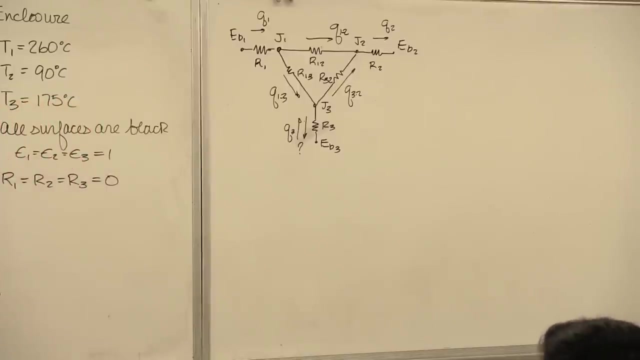 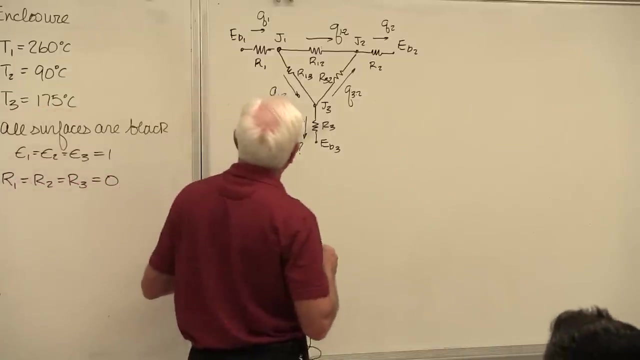 way, I know that Over here three is 175.. 2 is 90,. okay, it goes that way. I know that. What I don't know is which way that Q3 is. I won't know it until I solve the problem. which way it is going to go, Okay, So let's. 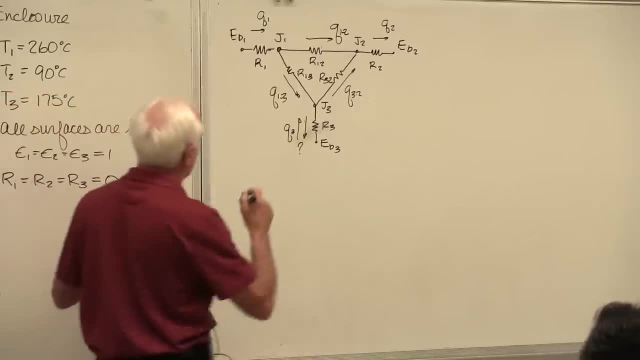 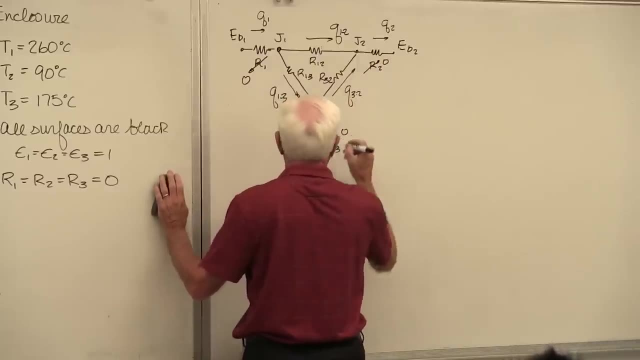 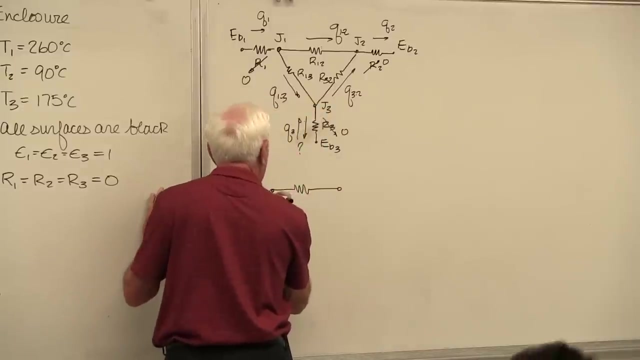 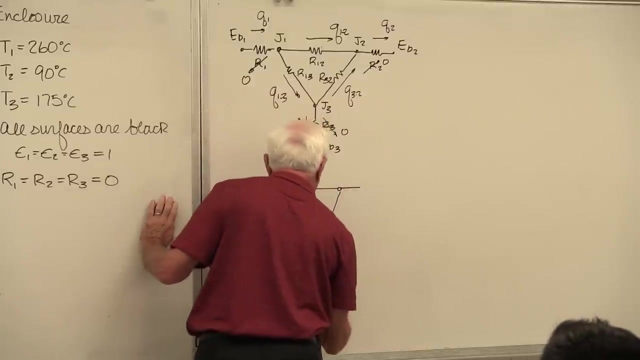 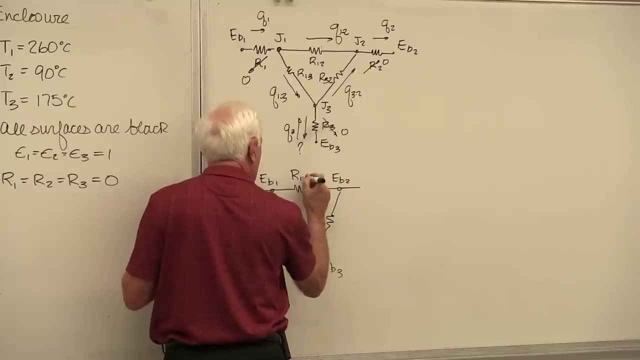 do first things first. This is all black surfaces. all the R1,, 2, and 3 are zero. Okay, gone, gone, gone. The new circuit, Look at, looks like this: EB1, EB2,, EB3,, EB4,, EB5,, EB6,, EB7,, EB8,, EB9,, EB10,, EB11,, EB12,, EB13,. 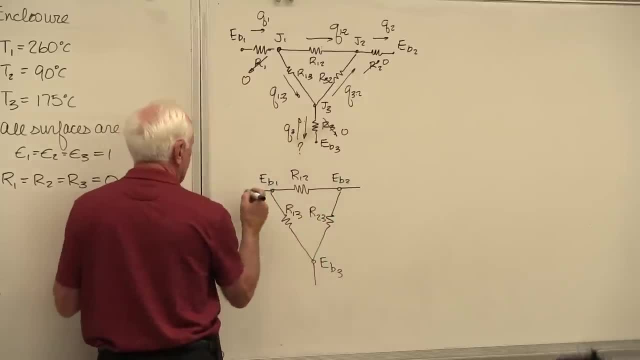 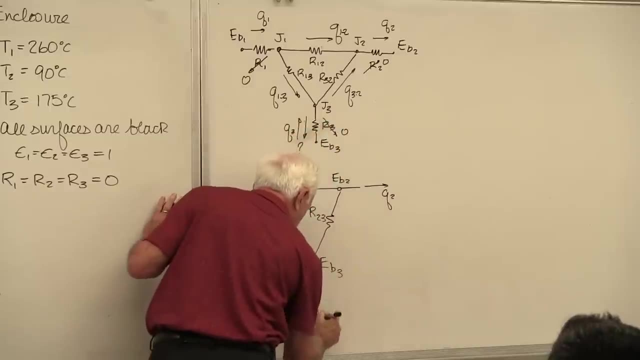 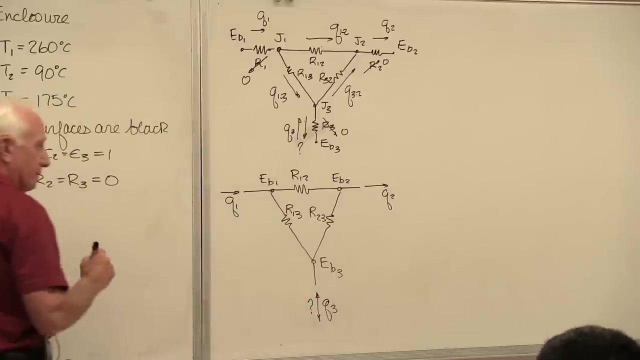 EB12, okay, Q1,, Q2,, I don't know which way yet, Q3. All right, but you know what I know, those EBs, Those are known. EB1 equals sigma T1 to the fourth black-body emissive power. 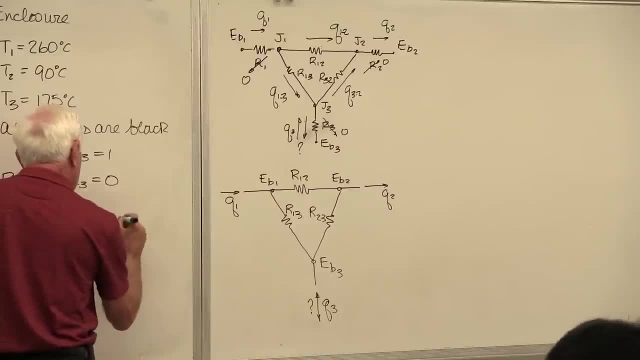 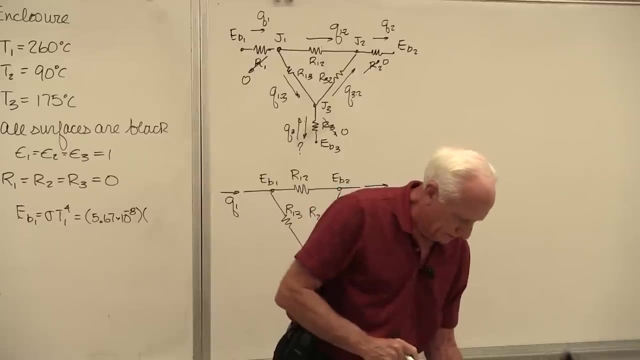 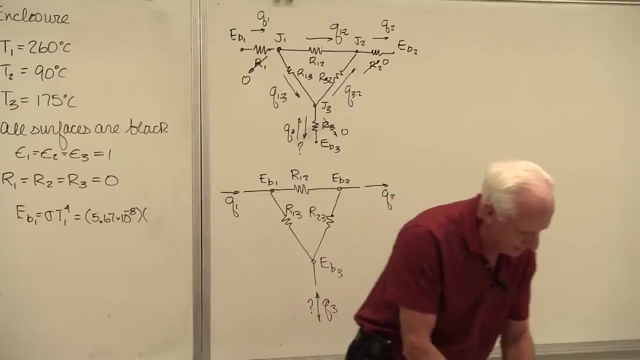 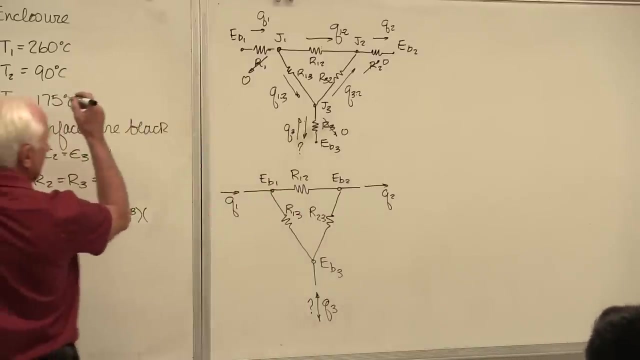 Sigma: 5.67 times 10 to the minus 8, multiplied by- let's see here, oh, there, it is okay- multiplied by my temperature Five. now, don't forget, we're in chapters 12 and 13,. absolute: 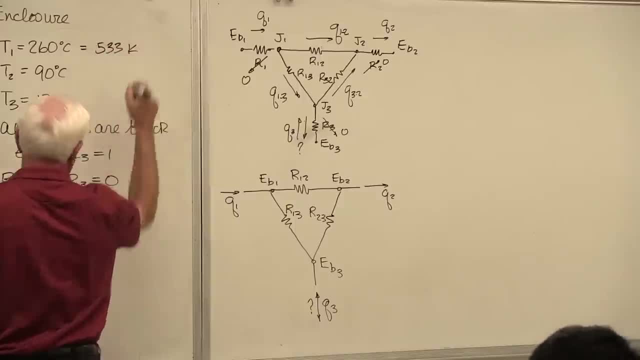 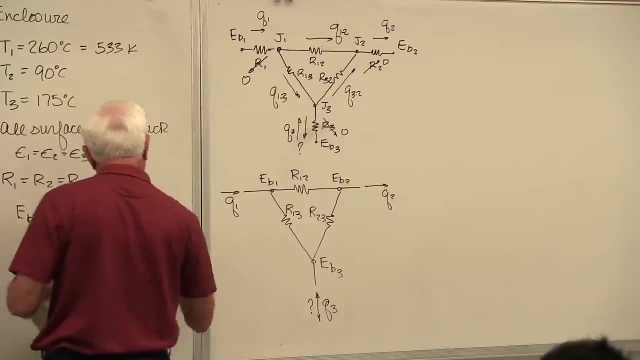 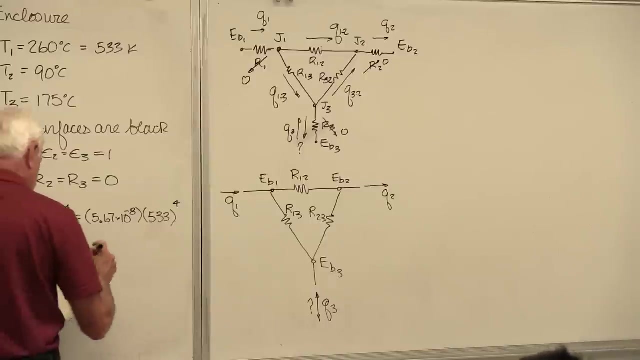 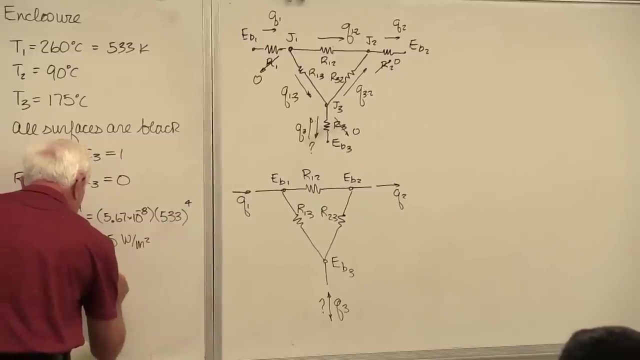 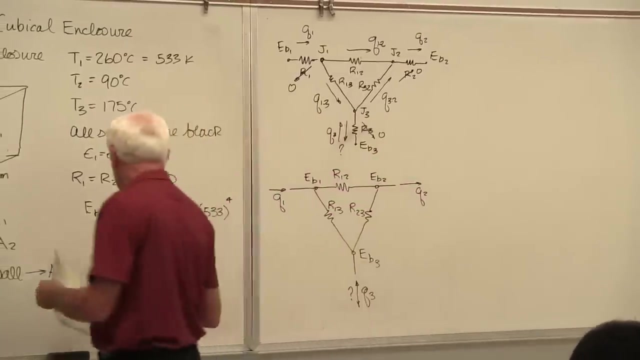 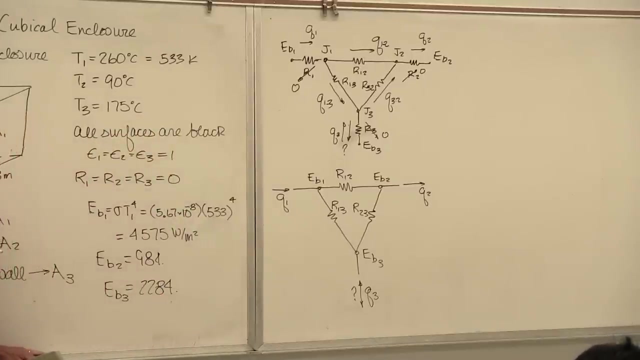 everywhere. 533K Times, 5, 33 to the fourth. EB1, EB1, 45, 75.. EB2, it's known EB3, it's known 2284.. When you're doing these calculations, you can kind of take a shortcut, if it helps. 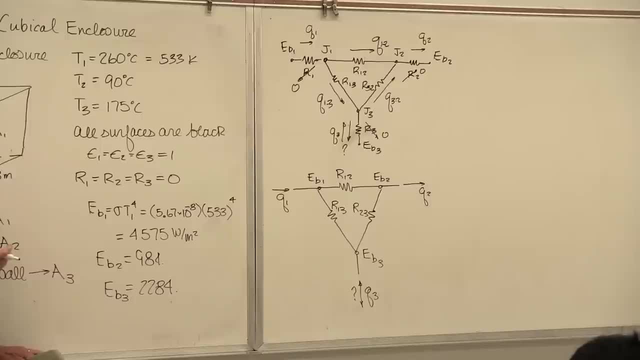 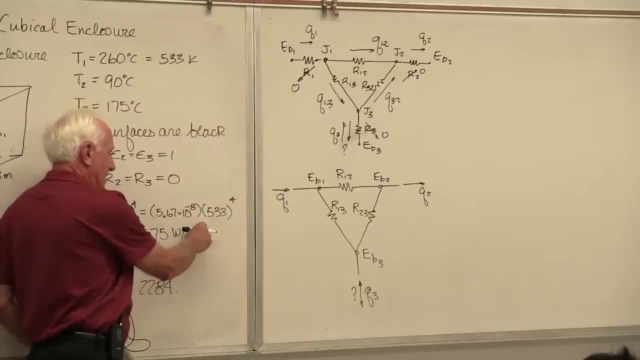 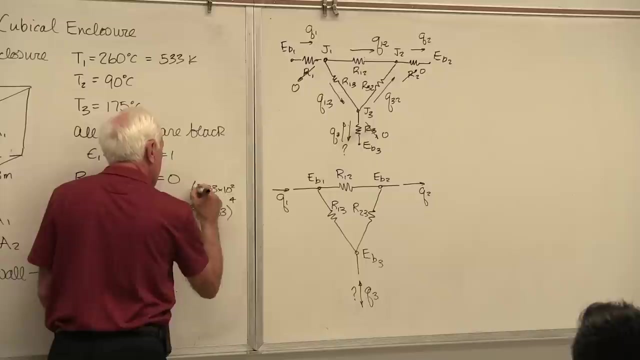 It doesn't save a lot of time, but sometimes it saves you making some silly keyboard errors. If you're doing this calculation right here- the easy way out, since these guys are always in the hundreds As you add degrees C and 273, what you do is you make this 5.33 times 10, squared raised. 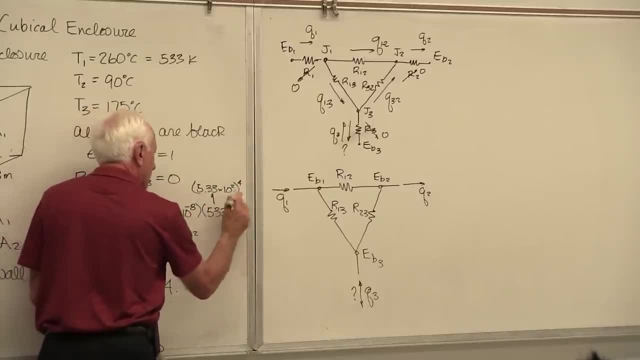 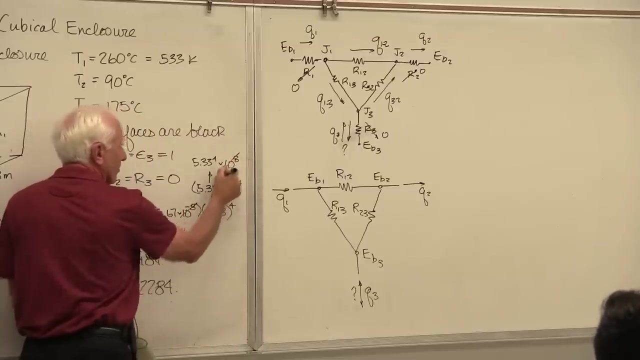 to the fourth. Then you make that 5.33 to the fourth times 10, squared, raised to the fourth, and lo and behold, oh, those guys go out. thank goodness I don't need to key that in, at least on my calculation. 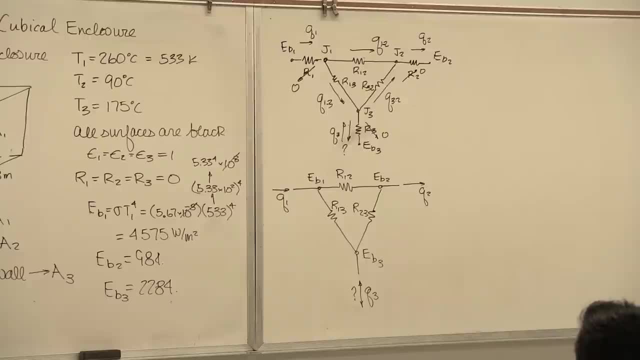 So you can avoid keying in those 10 to the eighth stuff and 10 to the minus eighth stuff. Just move the decimal point on the temperature two places to the left, knock out the 10 to the eighth, 10 to the minus eighth and now raise 5.33 to the fourth power. 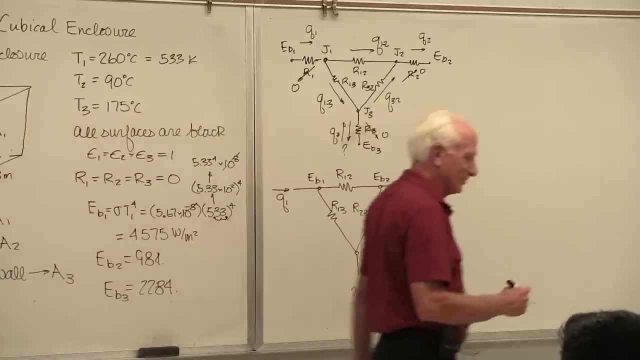 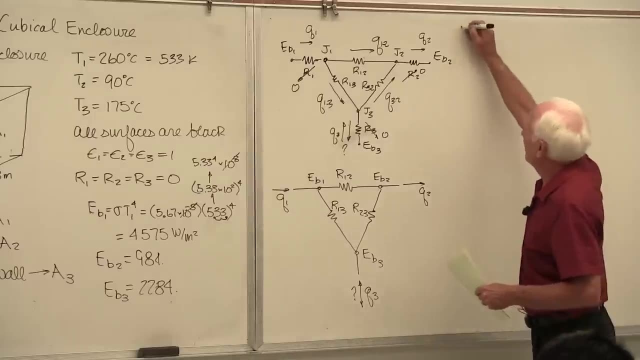 It just saves some calculations in a stressful situation like an exam, where you might key the wrong thing in and then, all of a sudden, your answers go crazy. All right, So there we are. All right, Let's call these things what they are. 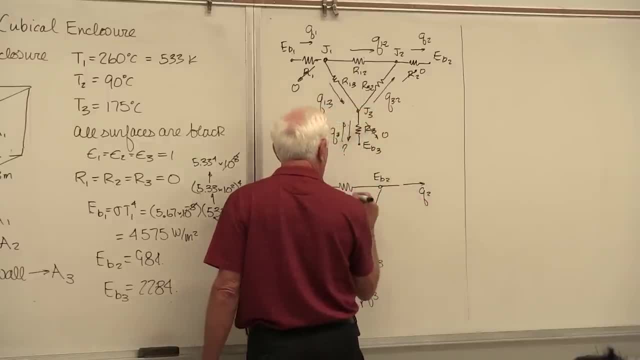 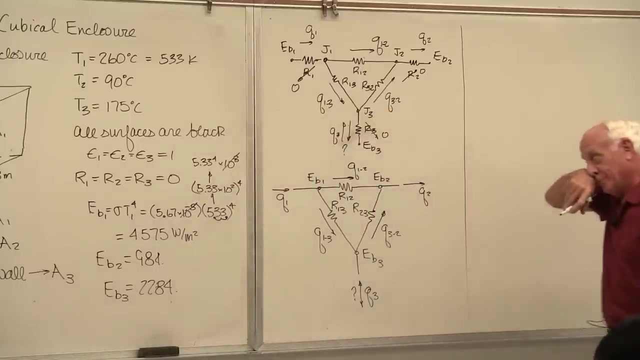 I'm going to move R12 inside here: Q1-2,, Q1-3,, Q3-2.. All right, Let's find Q1., Q1-2.. Q3-2., Q3-2.. Q3-2. 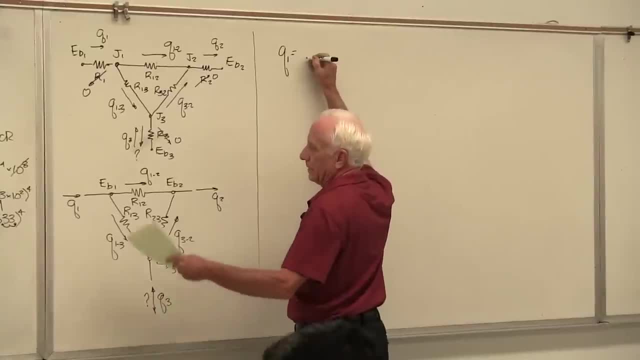 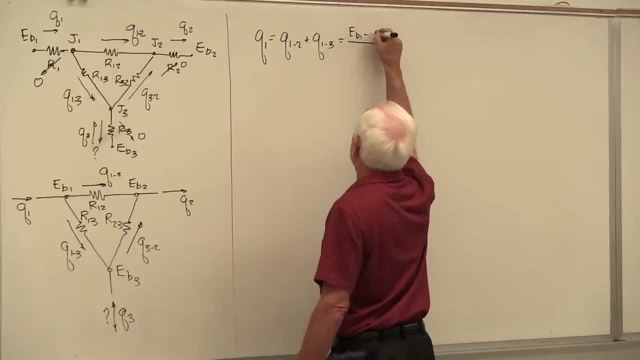 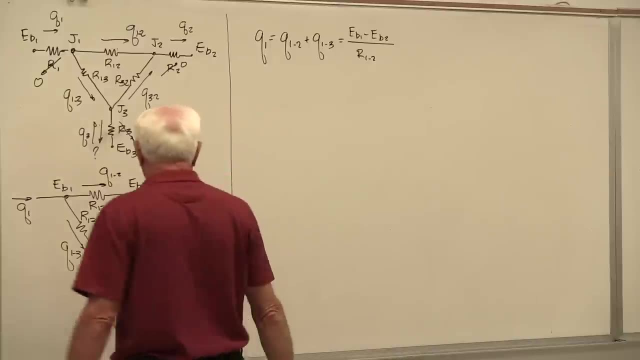 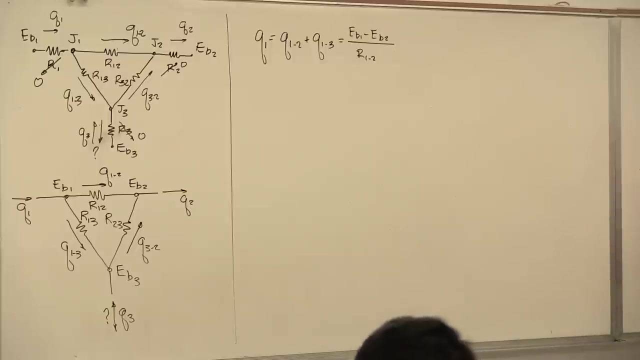 Q1-2, EB1 minus EB2 divided by R12.. Okay, Now I need the R's, Okay, Okay. So next step: I'm stuck here until I find I'll put them both on here, plus EB1, minus EB3 divided by. 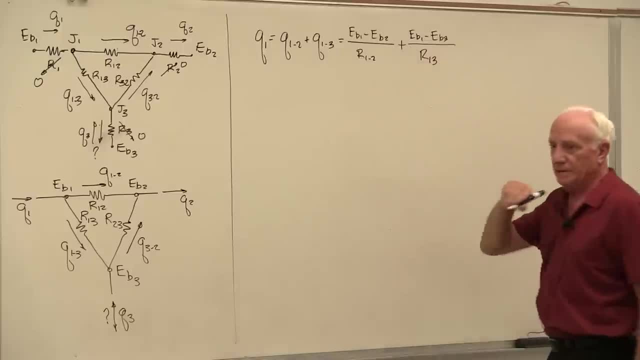 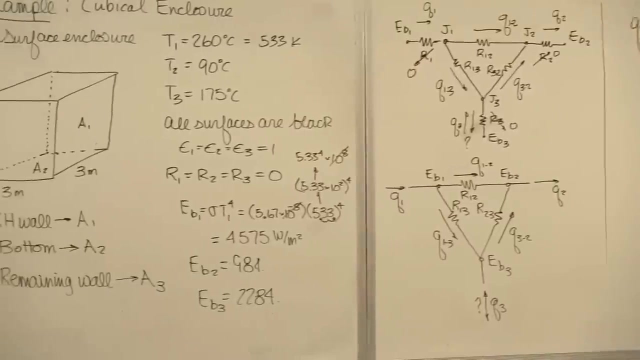 R13.. Okay, So I'm going to find the R's. I think I need all that board space over there, so I'll put the R's over here from figure 13-6.. Okay, All right, All right. 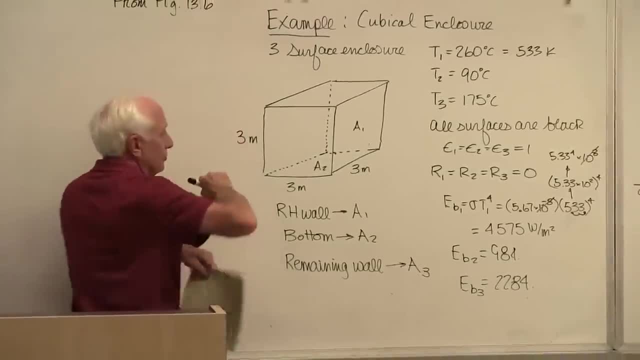 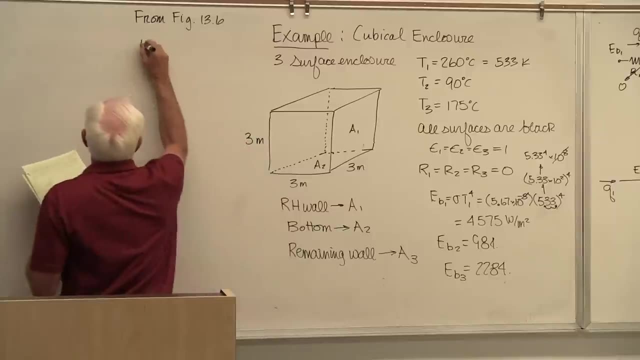 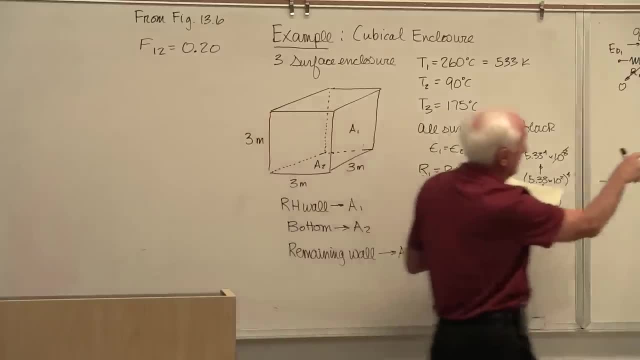 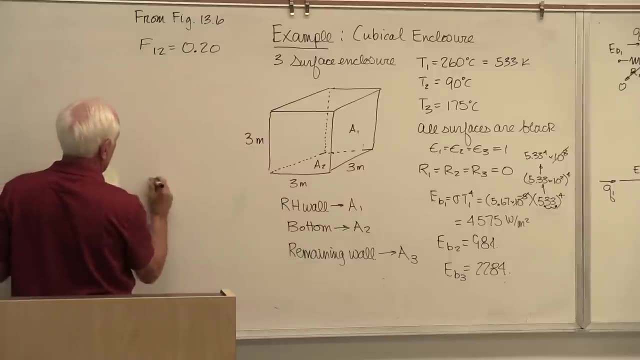 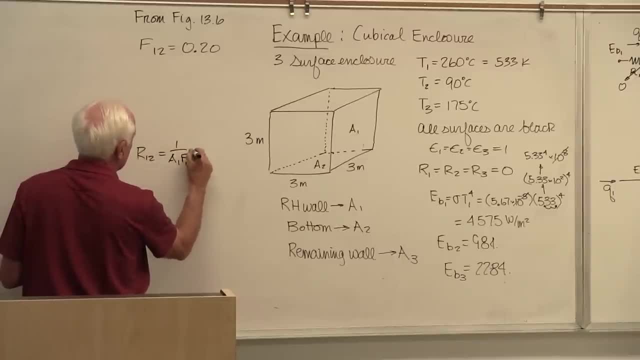 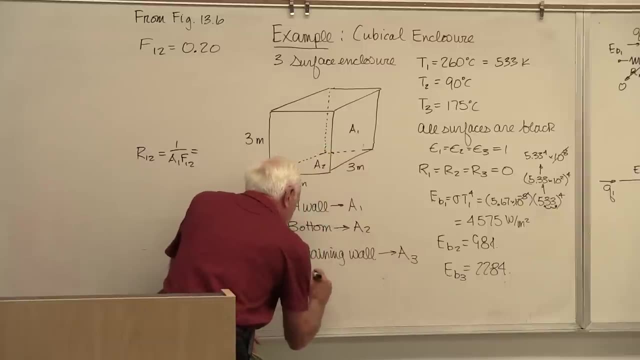 equal 1 over A1F12.. I'll put them down here: A1, equal 3 meters squared 9 square meters. A2 is the same 3 square meters, 9.. A3, there's 4 remaining. 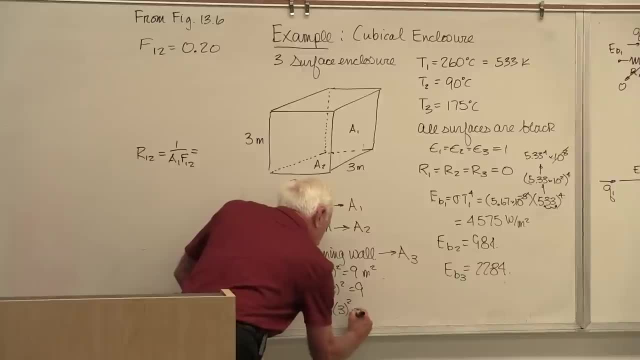 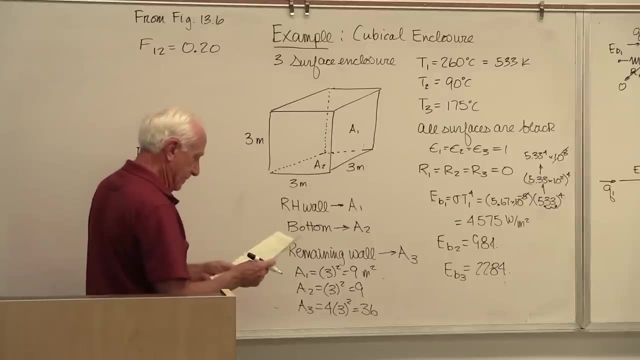 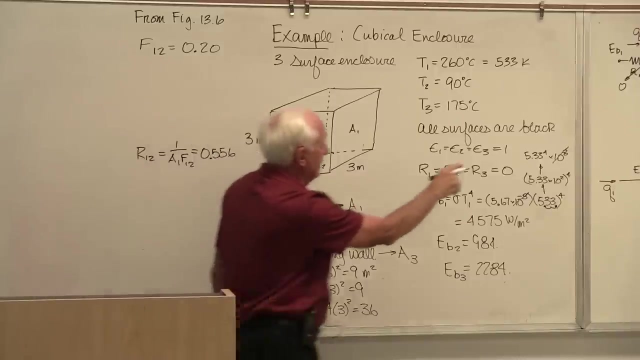 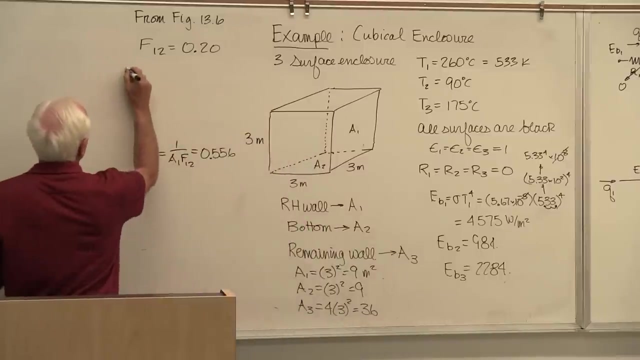 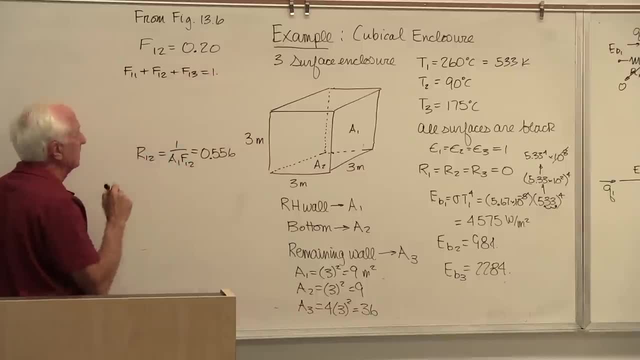 equal one. Enclosure law, energy balance. Surface one: plain surface- F11 is zero. Surface two: a plain surface- F22- is zero. Surface three is not plain. F33 is not equal to zero. F33, not zero. Okay, So F13, one minus 0.2, zero, 0.3, 0.5,. 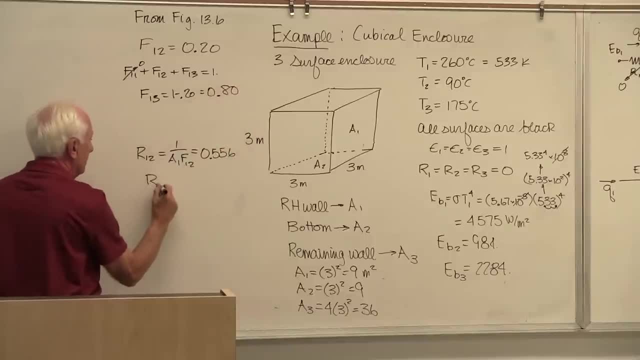 0.80 R131 over A1 F13, put it in there, 0.139.. By symmetry looks to me like F13 is the same as F23.. Of course it is. F13 is the same as F23.. It's a cube, symmetrical three by three. 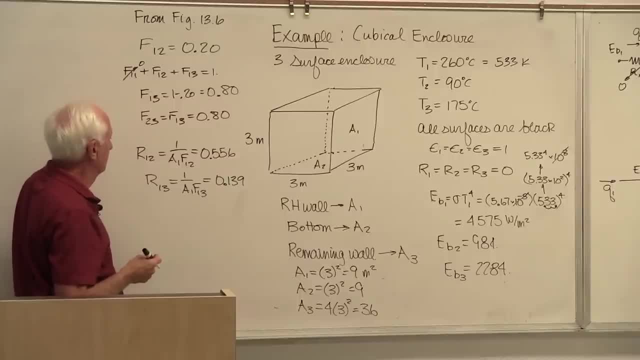 by three. all the sides are equal, So of course it's the same Conclusion. Oh, then that must mean R23 is the same as R13.. Yeah, it is. So now I've got a little bit more time, I've got them all. I've got R12,, R13, and R23.. Don't forget that. if I want to well. 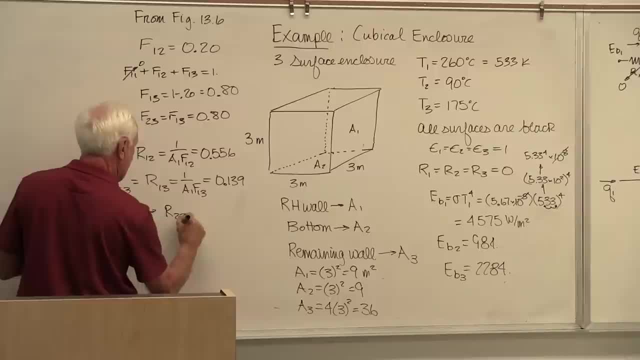 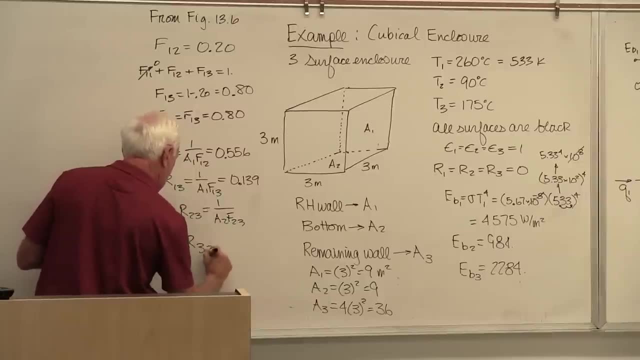 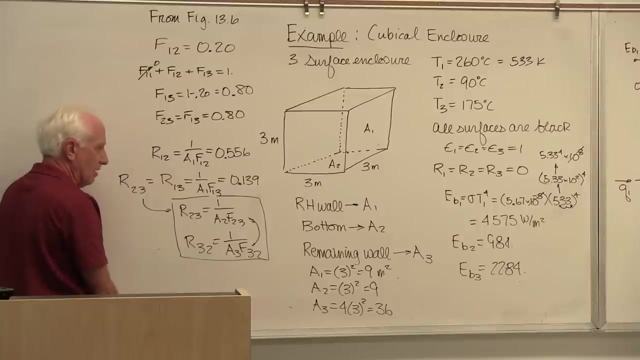 I'll write down R23.. Don't forget reciprocity A2, F23 equal A3F32.. Conclusion: It doesn't matter the order of the subscripts, Because of reciprocity, R23 equals R32.. R21 equals R12.. R12 equals R13.. 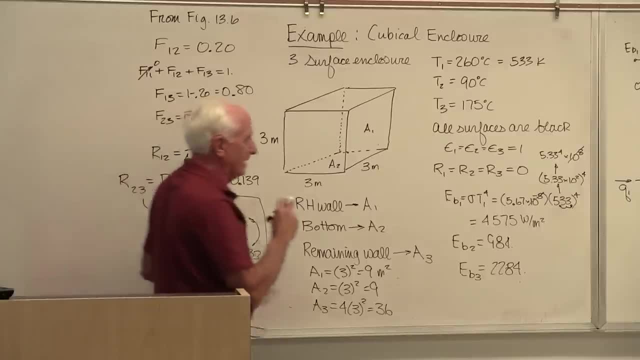 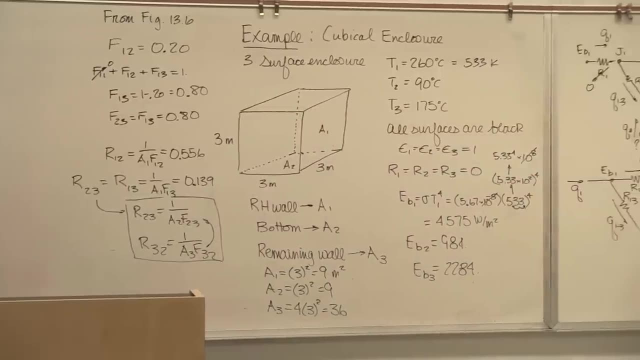 3 equal R 3 1. it doesn't matter. you say, you know how can you call that Q 3 2 and that R 2 3. it doesn't matter if you don't like that, call it R 3 2, it's the. 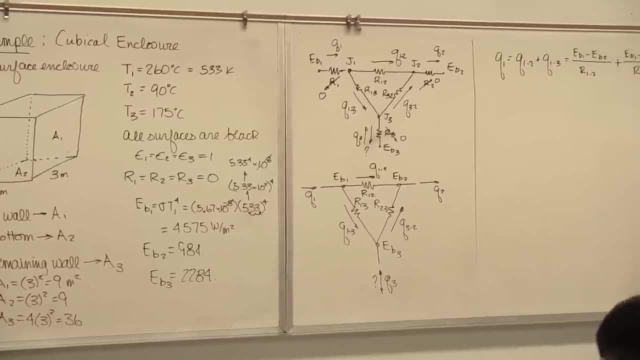 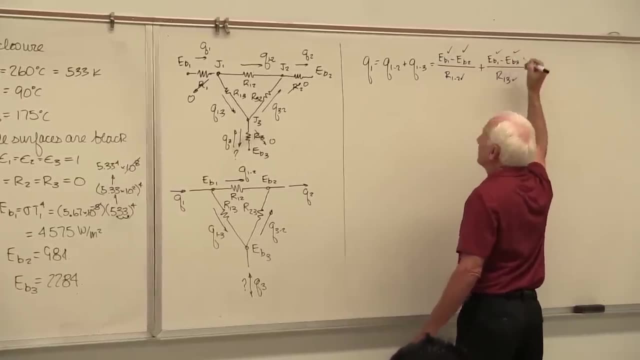 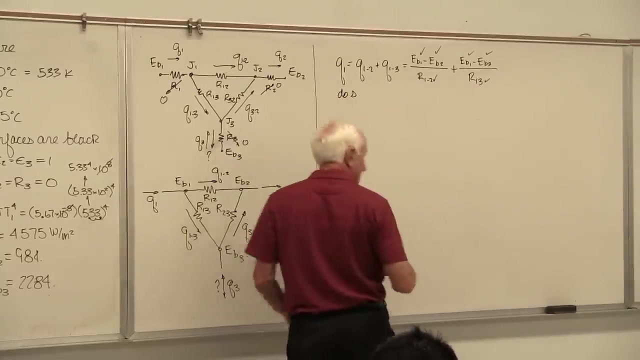 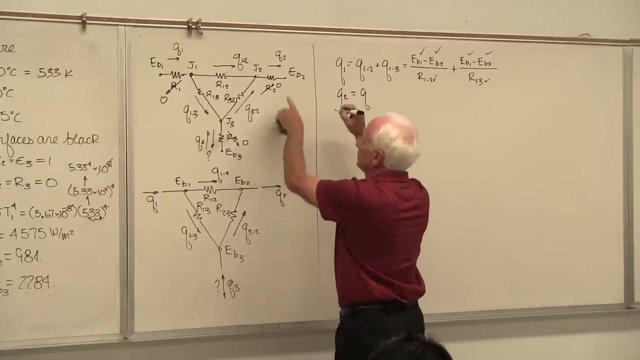 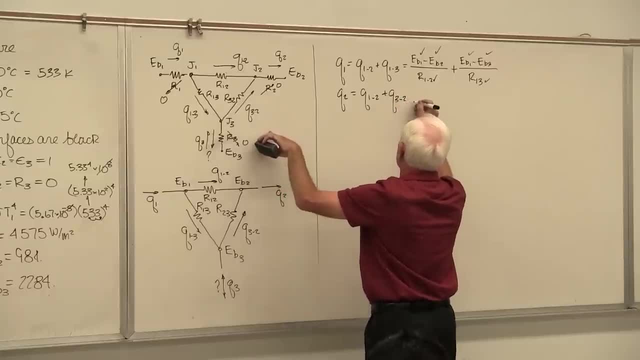 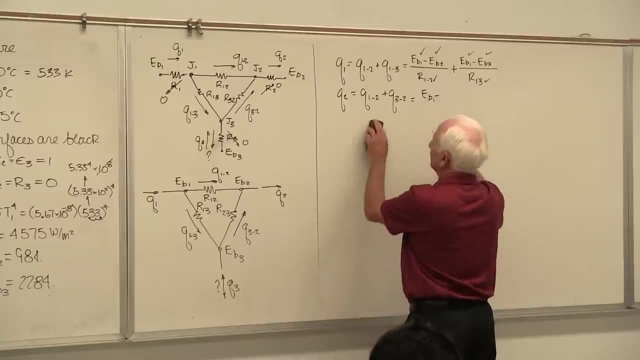 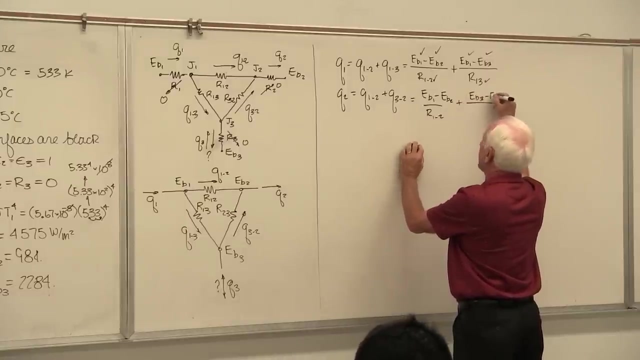 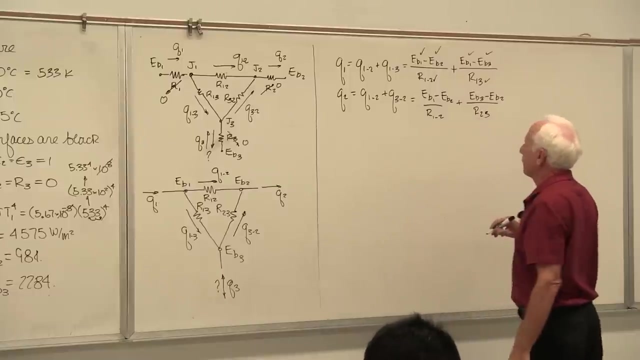 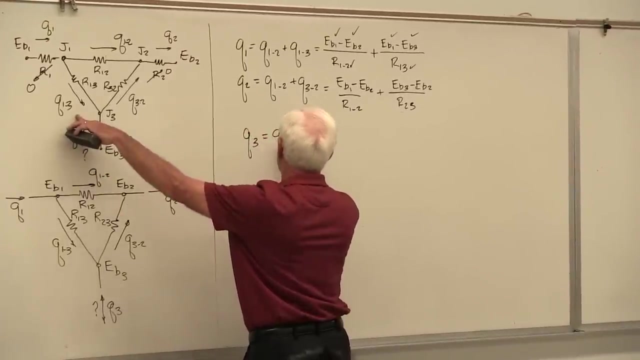 comes in: Q 3: 2: okay. e B 1 minus 2: 0. yeah, one, that one, two, two got it. okay. the last one, Q 3. what comes in: Q 1: 3. what goes out, goes out minus sign. Q 3, 2. 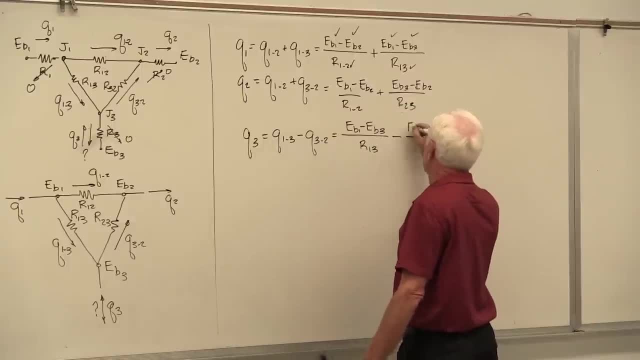 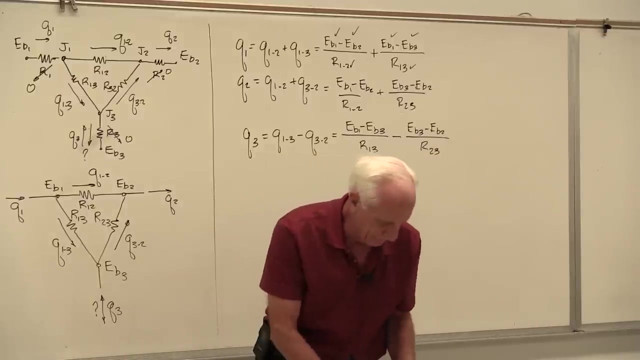 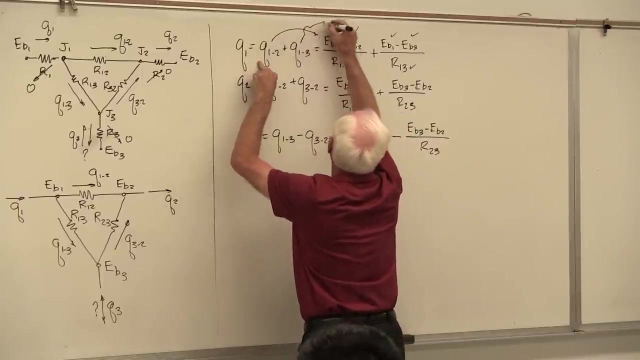 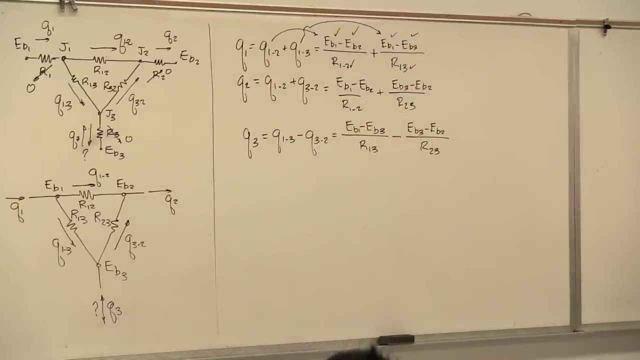 minus. so there, how many different cues are there? there, there's six, six different cues. you want to find them? there they are, they're all right there. here's Q 1, 2, here's Q 1, 3, here's Q 1, and so on and so forth. you can find all six Q. now to 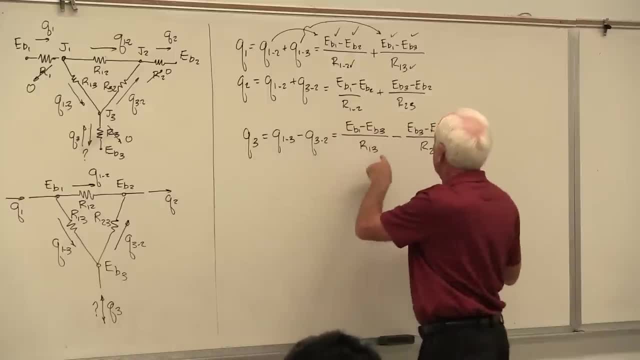 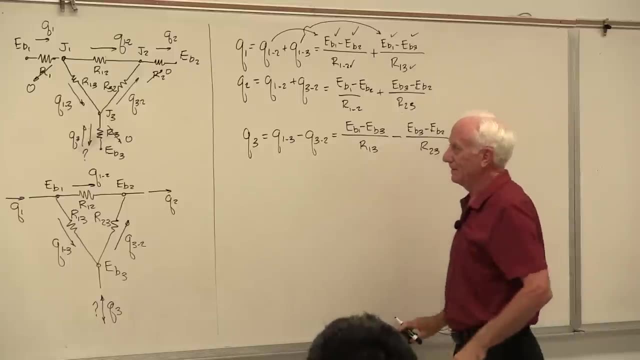 see which way the heats flowing down here. look at this thing right here, this calculation: if Q 3 is negative, you're gonna get minus. so there are three Q's negative. you guessed wrong, okay, Okay, because this equation right here will tell me which. 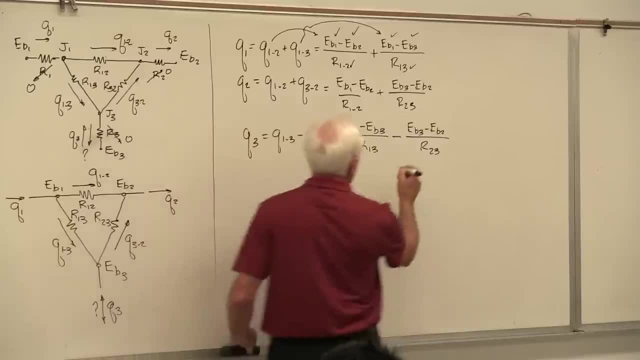 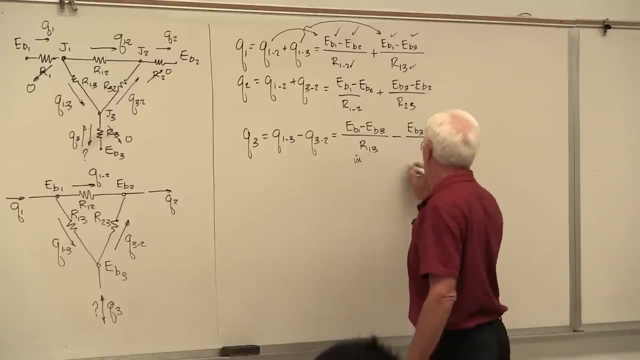 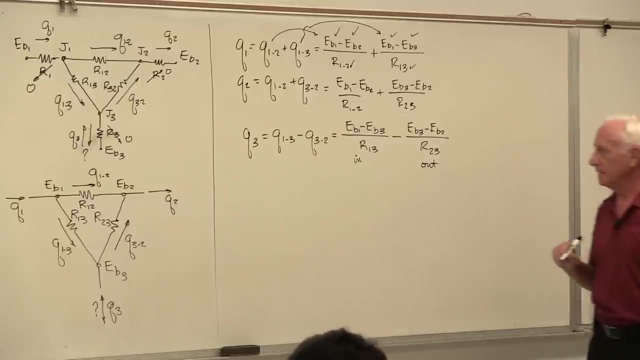 way this Q is positive or negative. If this number here is big, compare that number, it's a negative sign. What is this? This is what's coming in. What is this? It's going out, okay. So that's how you tell which way. Q3 is Okay if 5 watts comes in and 3 watts goes out. 2. 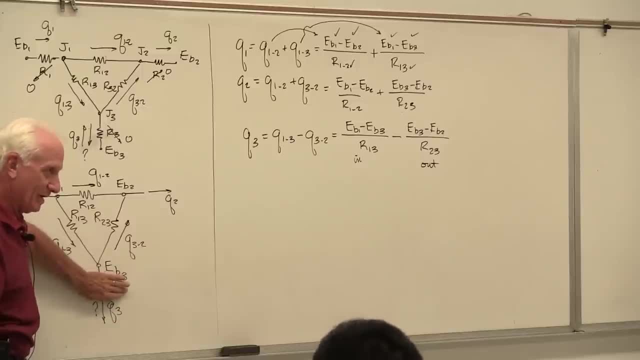 watts have to go down That way, that way. So once you find Q1, 3,, Q3, 2, that's the game you play. This comes in, that goes out, this takes care of the rest. That makes it. 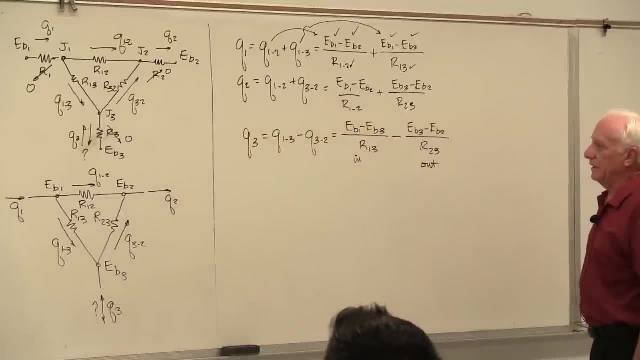 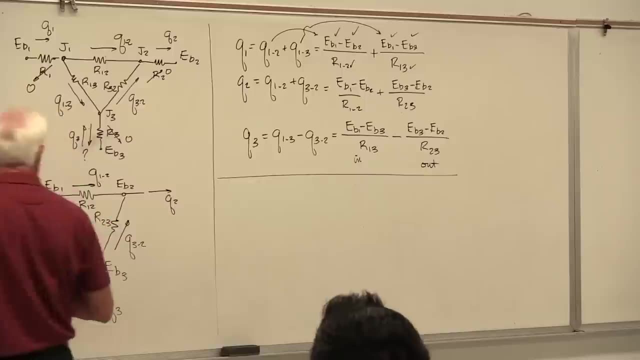 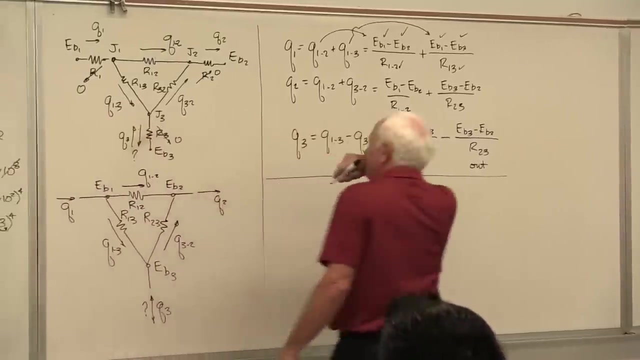 equal sign. Okay, Okay, black surfaces- all right. So now we've got black surfaces. Obviously, in the real world there's not too many problems where all the surfaces are black. Generally they're not black, So our next step is non-black surfaces. Okay, no more of that. equal to 1.. 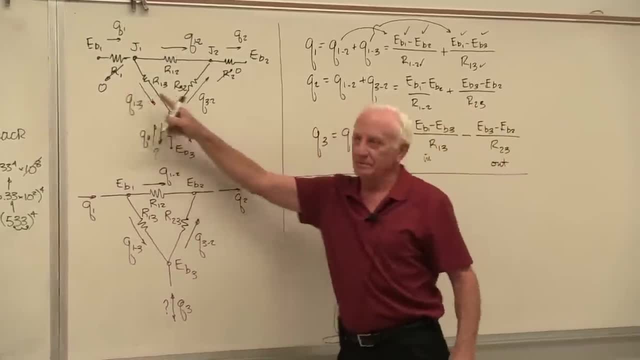 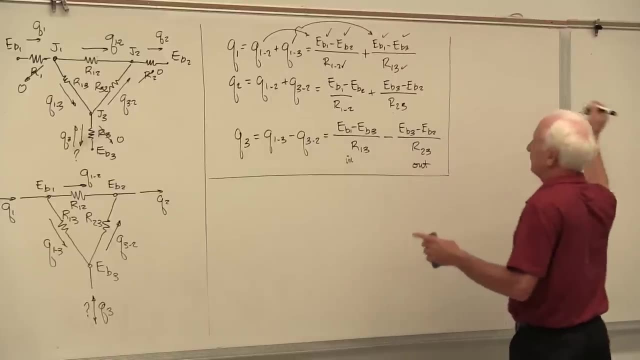 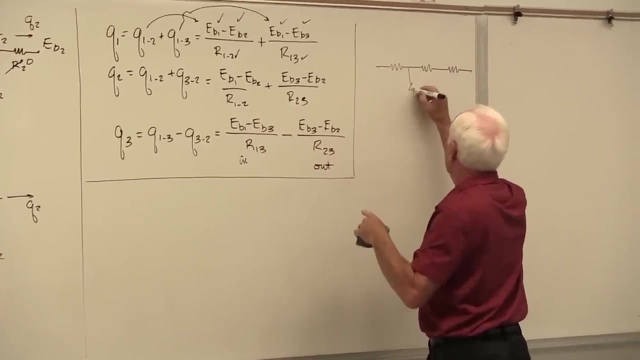 Okay, Don't put them equal to 0.. I'll put the picture here. No, I'll do work over there. All right, so now we have again same thing: 250 positive 0. Except now there are not 0.. 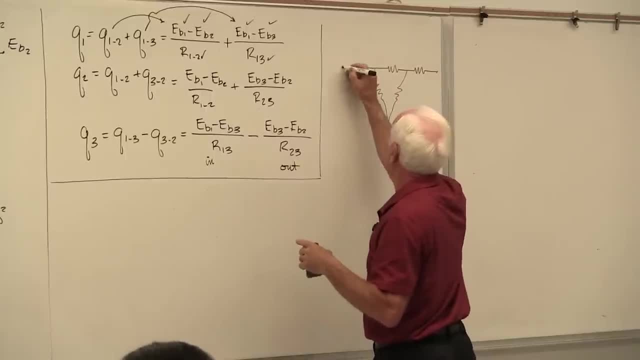 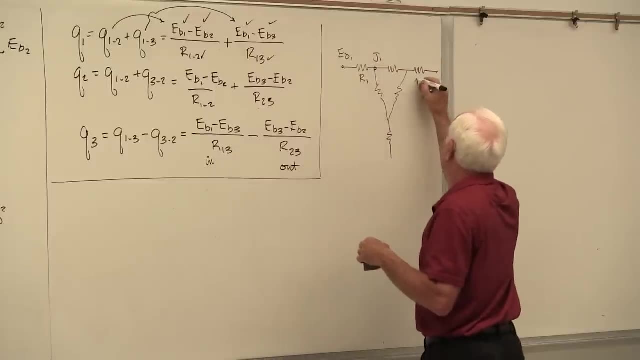 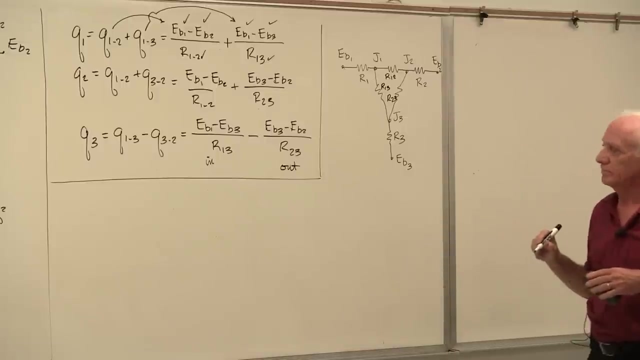 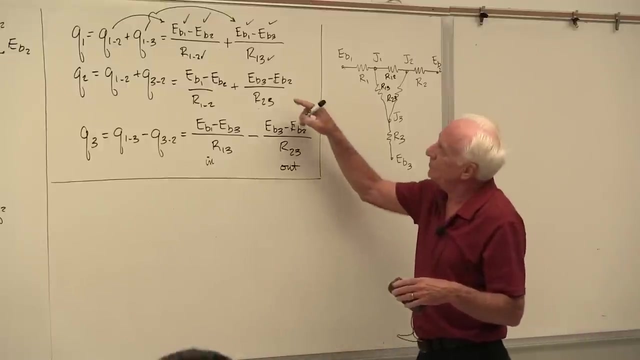 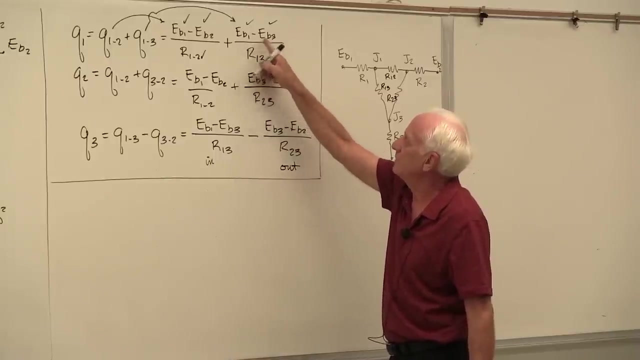 Thank you. All right, Did you get this Good? Thank you. You know, you might say, when you wrote this down here: EB1 minus EB3 divided by R13, okay, the 1 comes first, the 3.. 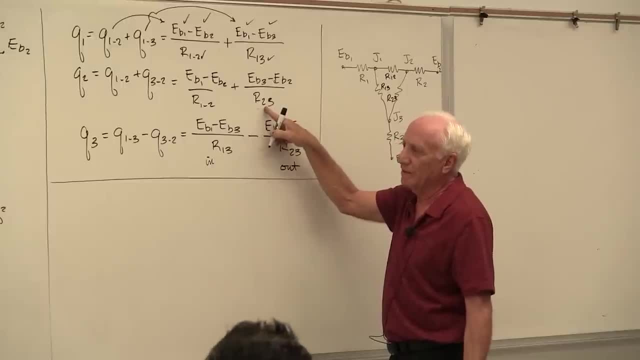 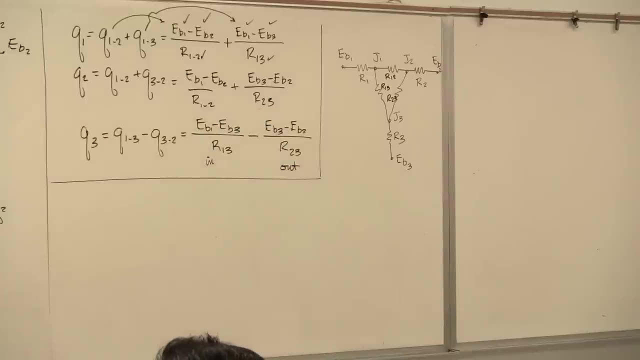 Why didn't you make it R32?? Well, first of all because I know reciprocity. R32 is R23.. Which one do I want to find Back over here? do I want to try and find first R32 or R31?? 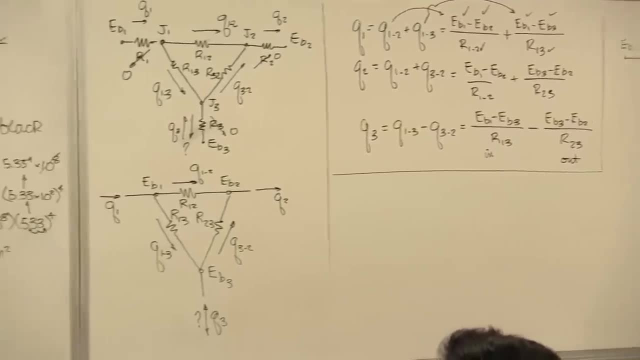 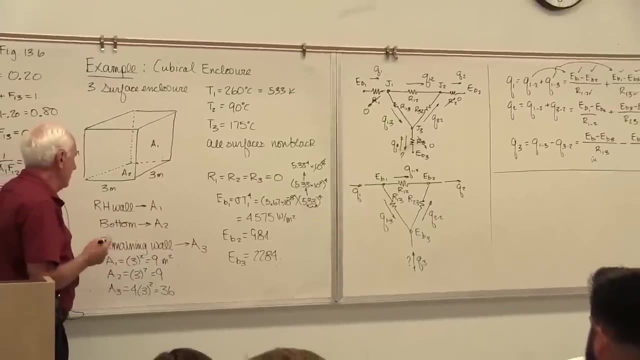 Oh my gosh. no, I don't want to find R31.. First I want to find R. from the small surface to the big surface, R13.. So I find R13 first. There, it is right there, R13.. 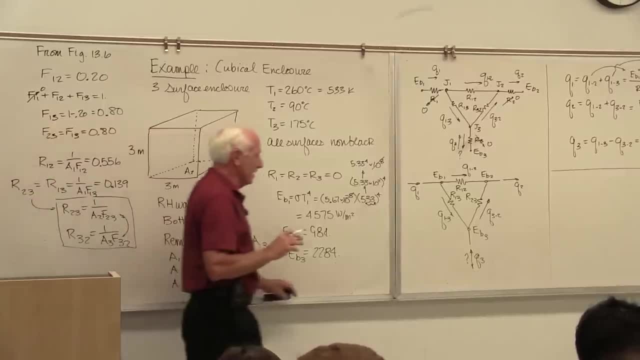 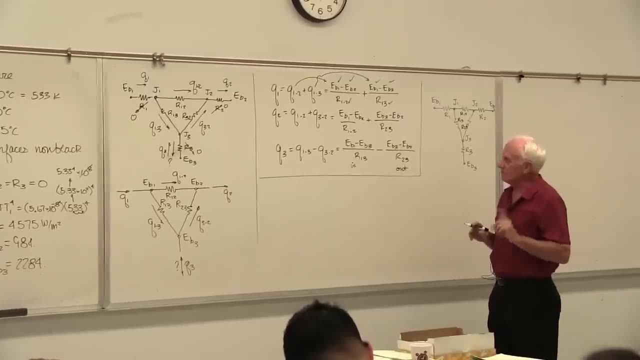 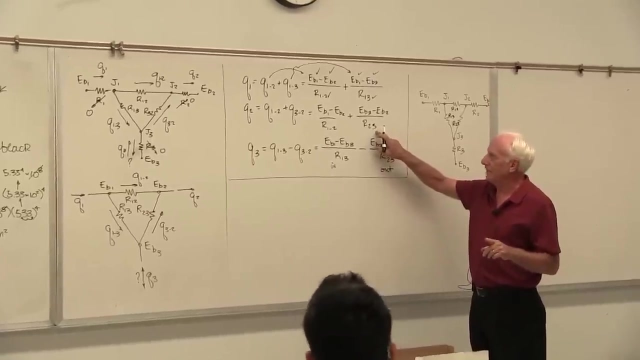 I don't want to find R31. So my conclusion is: you've got a choice to make to find these R's, the two subscripts, Take the easy way out. Sometimes one is easier than the other one to find. Maybe F23 is easier to find. 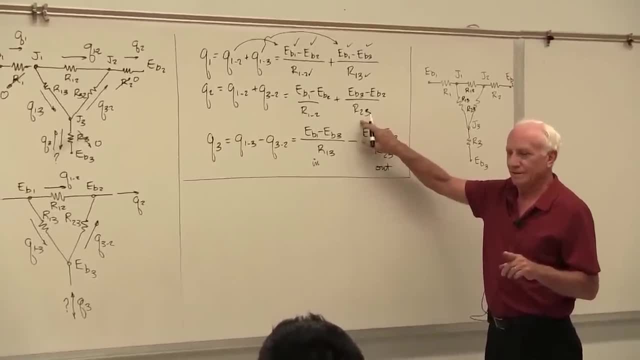 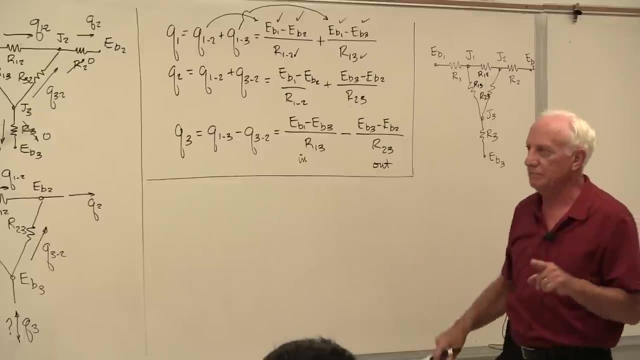 Maybe F32. Then use the R23. Take the easy way out sometimes. Look at them. There's two possibilities to find the view factors. Flip the subscripts, See which one's easier to get, And you'll see in homework that that works out sometimes that way. 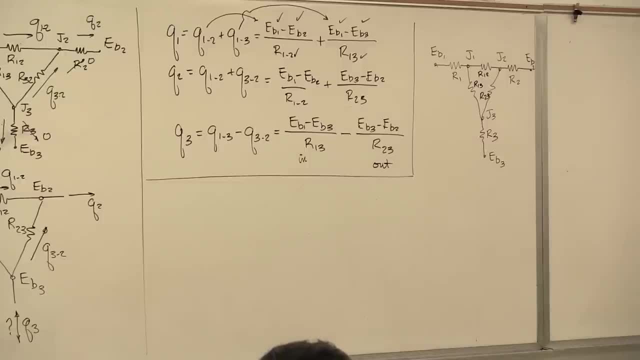 There's a hard way. There's an easy way. On a timed exam, there's two ways to do it, sometimes easy and hard. You want the easy way out, the less time-consuming way out. Okay, now Put the resistors in. 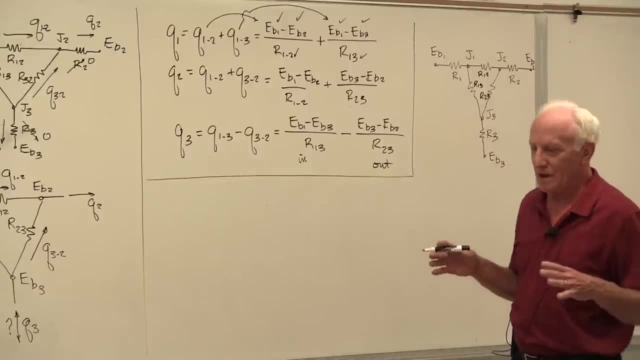 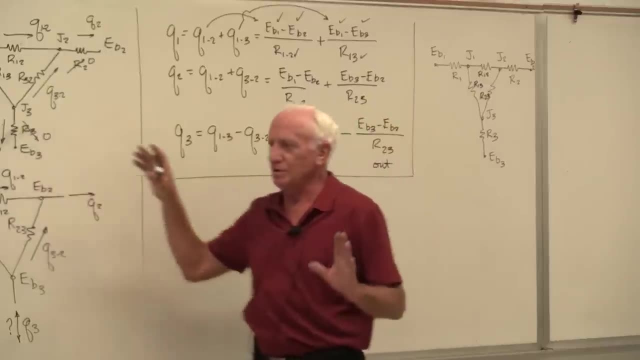 Pretend I don't know which way the heat flows, because for more complicated problems I'm not going to know which way the heat flows. There I used my intuition for the direction of the arrows. Let's assume you don't use your intuition here and you just want to solve for the Q's. 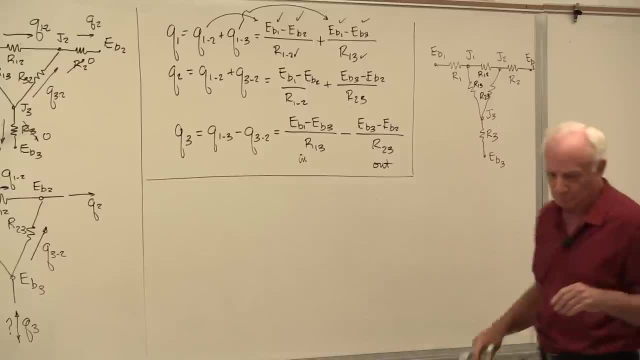 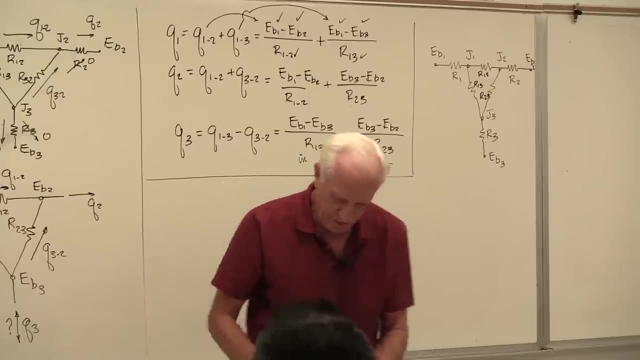 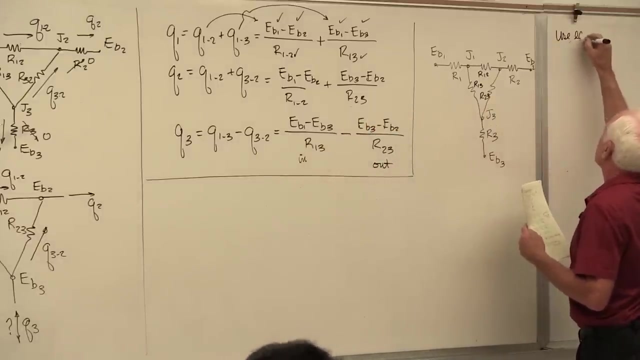 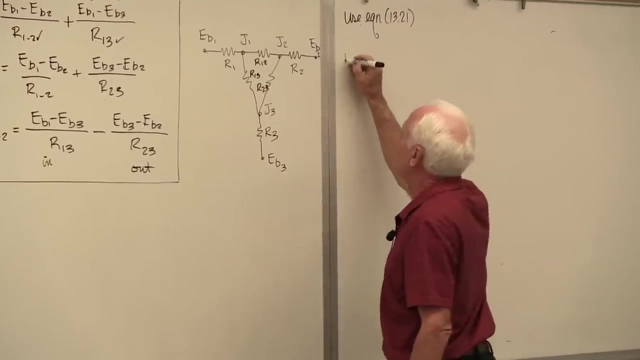 I don't know which way the Q's are going. So here's what you do: You go to equation 1321.. And let's give the answer to that question. If I go to the bottom of the� In the book And I'll kind of I'm going to write it for node one, node J1.. 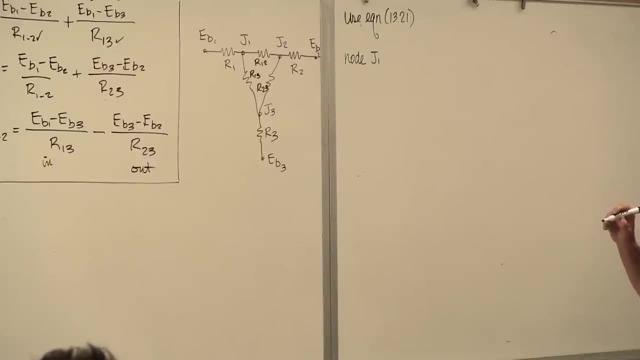 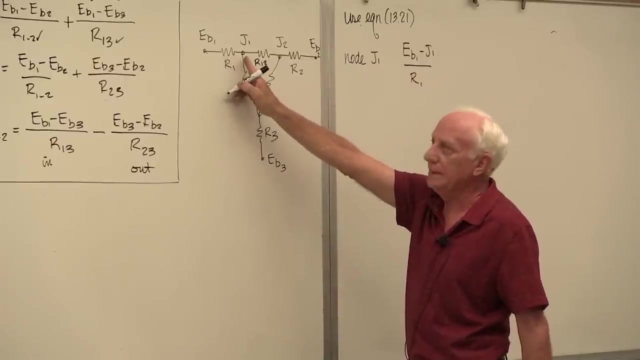 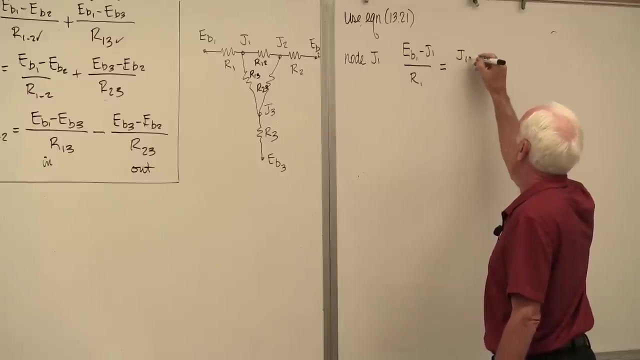 This is what it says: The heat that comes in to node J1 from the surface one goes out to nodes J2 and J3.. minus J1 divided by R1, that's Q1, equal the heat that goes out to J2 and J3.. Okay, I'll. 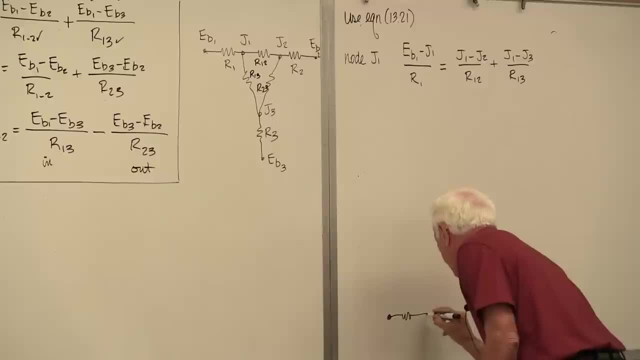 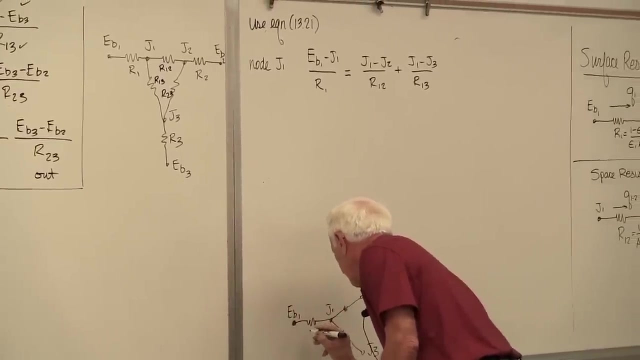 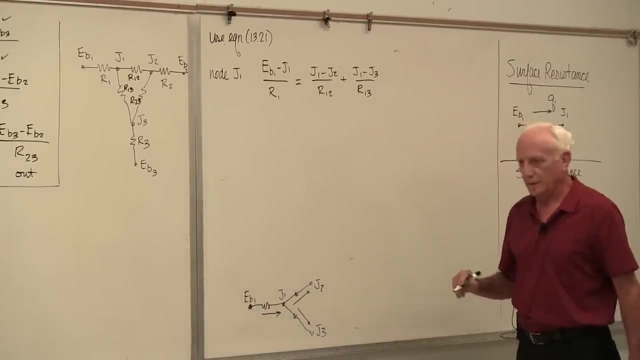 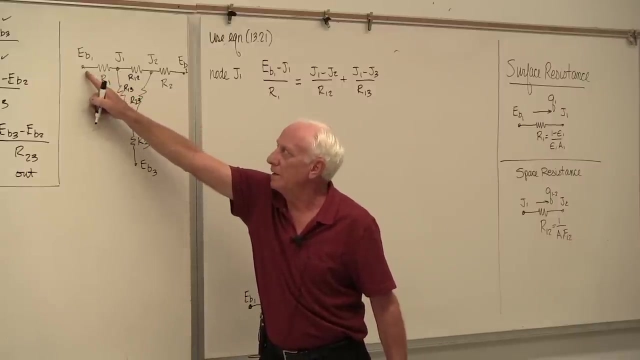 draw a little picture down here to show that. So there's the picture. The heat that comes in to no J3. J3 from the surface 1 goes out, some to surface 2, some to surface 3.. Are those directions? 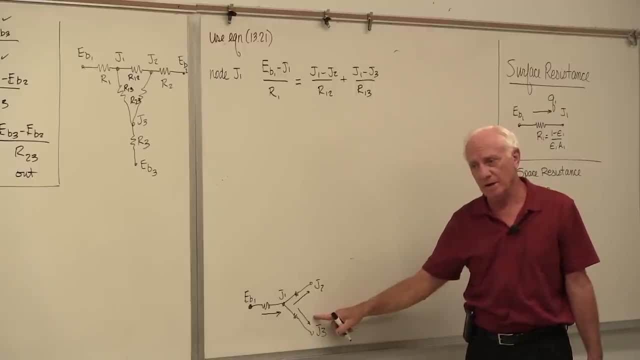 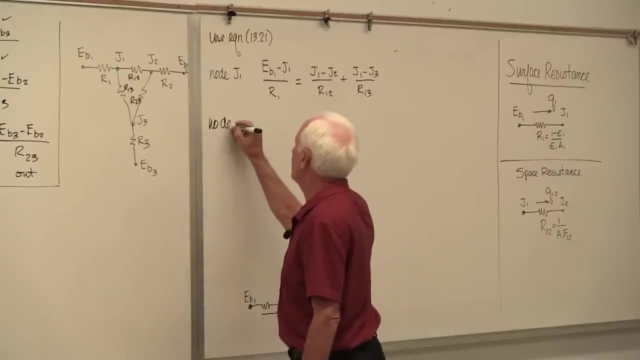 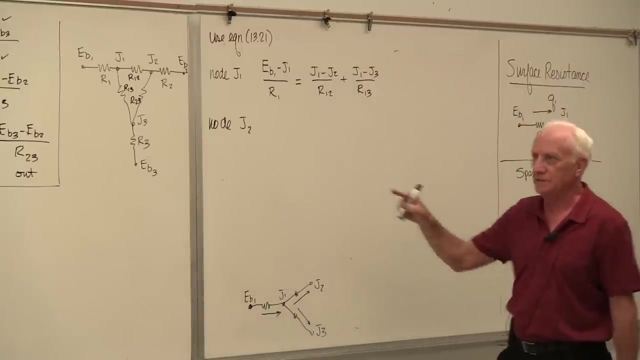 right? I don't know. I'll find out when I'm done if they're right or not, But for right now that's what you say. Now you write the next equation for node J2.. Here's what you say: The heat that comes in to node J2 from the surface that's up here, some, goes to. 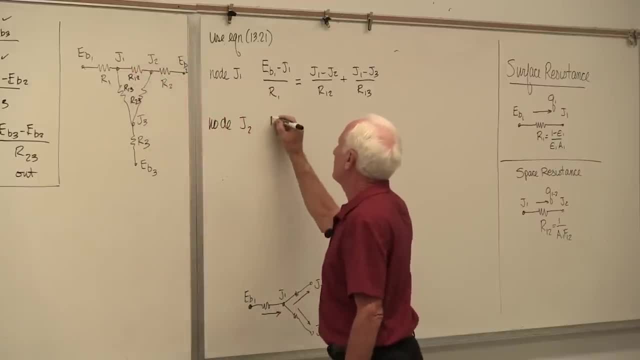 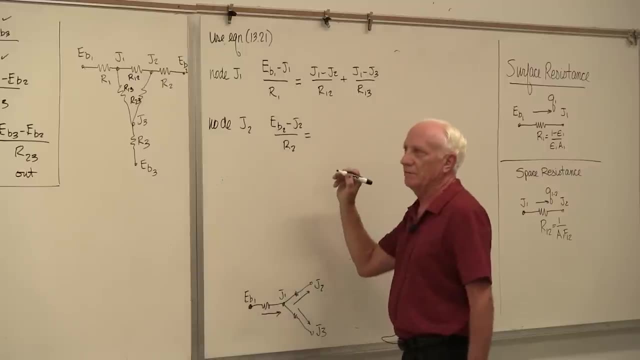 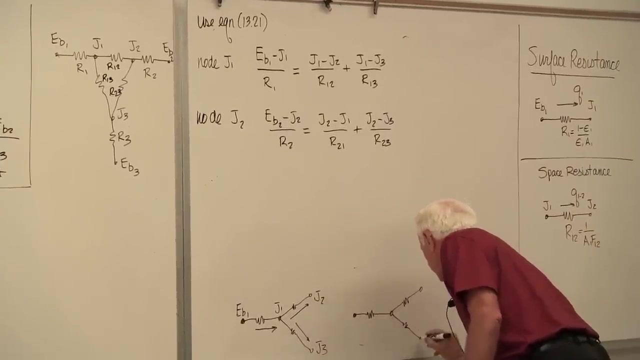 J1 and some goes to J3. Okay, EB2 minus J2 divided by R2 equals some goes to node 1, some goes to node 3.. Okay, I'll draw the picture down here. What comes in from surface 1, A1, goes out either to. 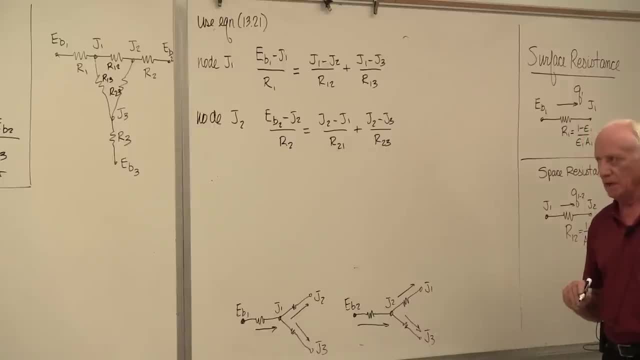 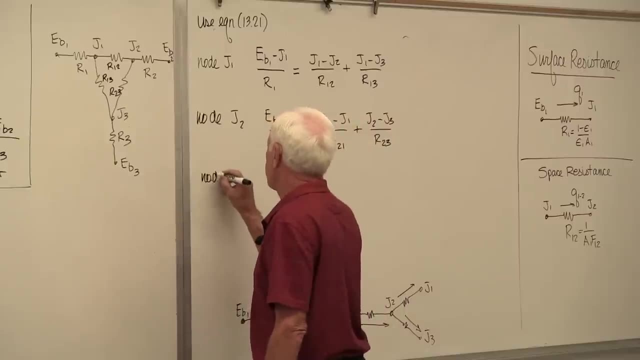 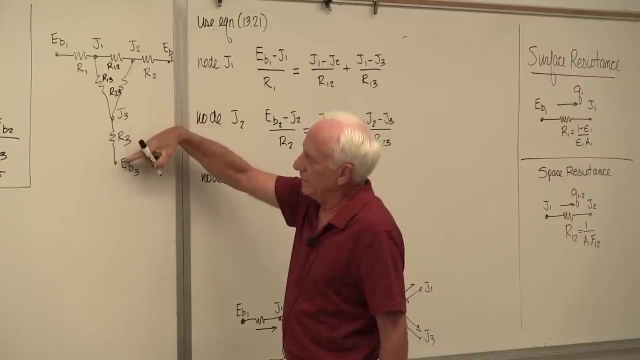 3 and to 1. that way That goes with that picture. Now I do know that. Okay, I'll draw the picture down here. Now I do know J3. Node J3. The heat that comes in to node J3 from surface 3 goes out to 1 and 2.. Okay, 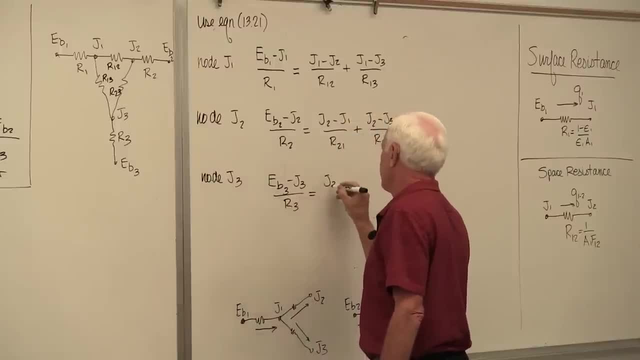 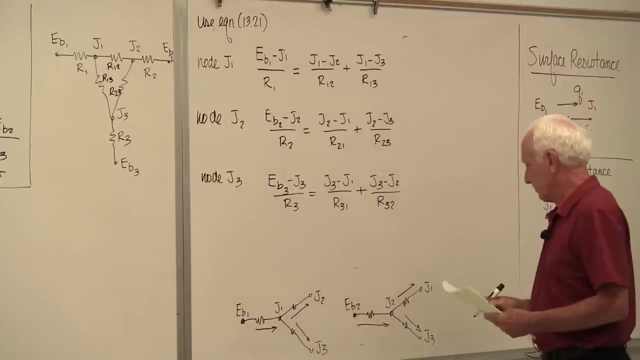 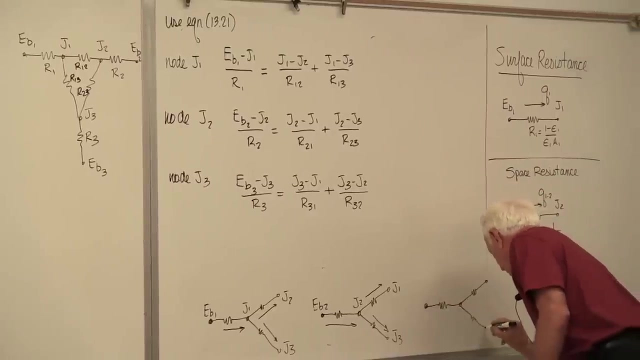 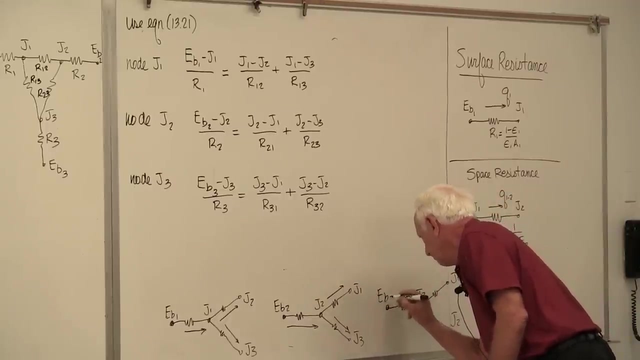 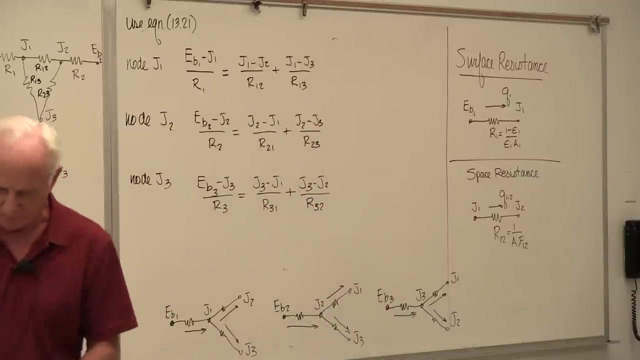 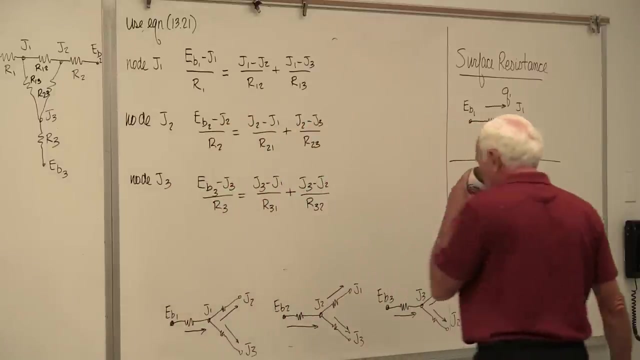 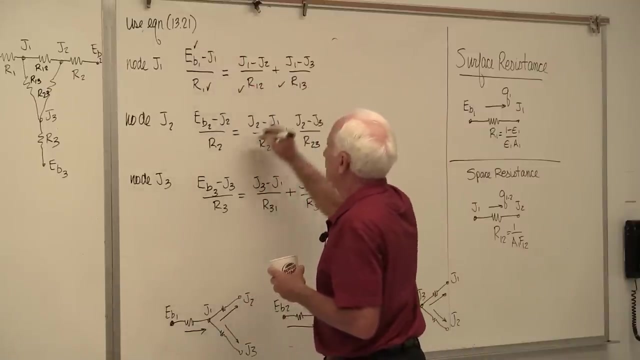 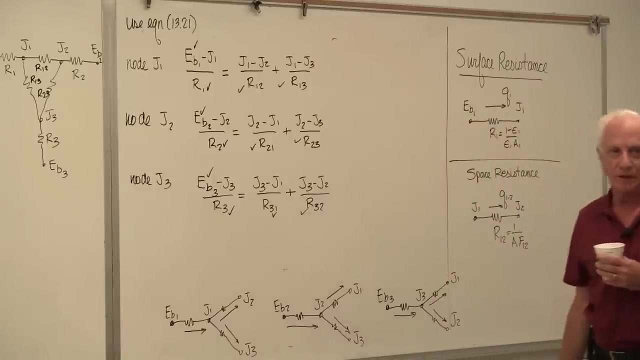 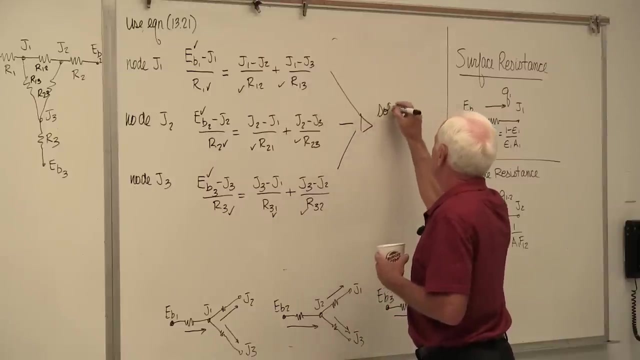 To 1 and 2.. Okay, Here's a picture. Put a checkmark by everything. you know What's left, Solve for it. Okay, J1,, J2, and J3.. Very similar to your next computer problem in class. 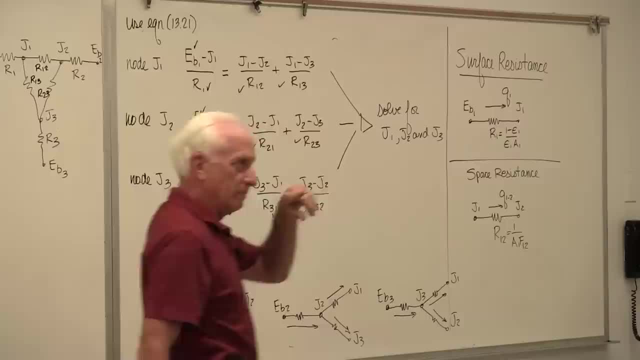 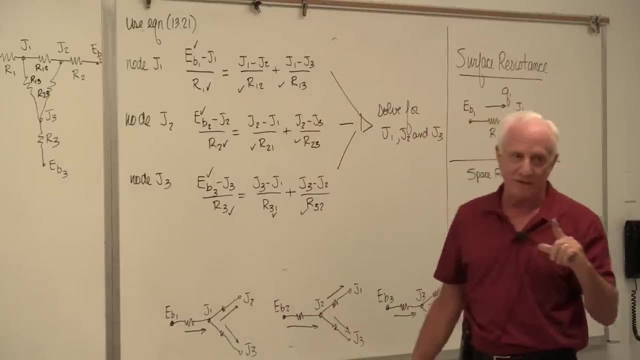 It's going to be a six surface enclosure like this room. There's going to be possibly six different temperatures of the walls. Each wall has a different temperature. You'll write. You won't know which way the heat goes from where to where. 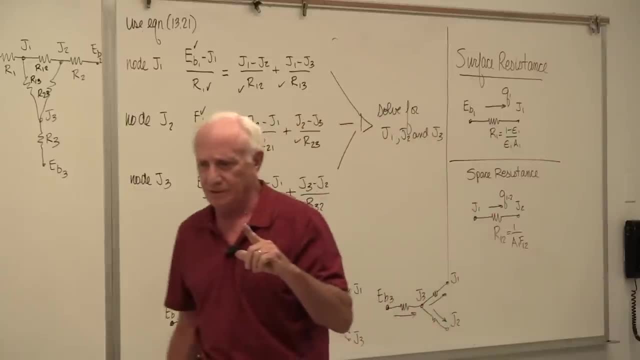 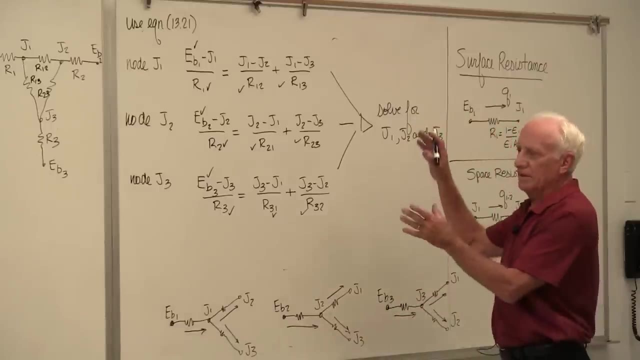 You can't guess it? Don't try and guess. Oh, I think the heat goes from that wall to that wall. No, it's not that easy. You can't do it that way. Don't even try and guess. Play the mathematical game. 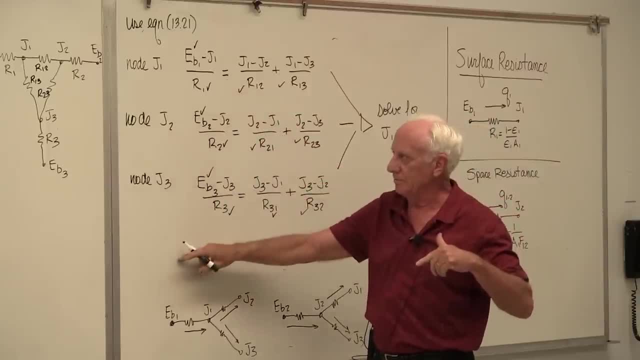 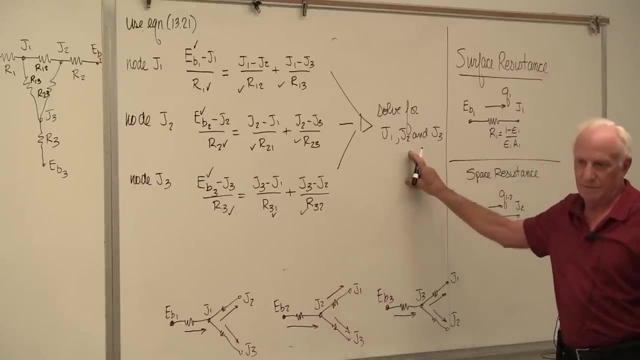 For every node. if there's six surfaces in this room, there's six different nodes, There'll be six different Js. You'll solve them whatever method- Excel, MATLAB, TI89, whatever it might be- and get the six Js. 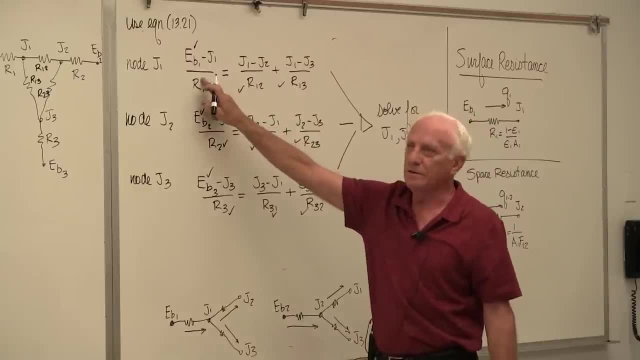 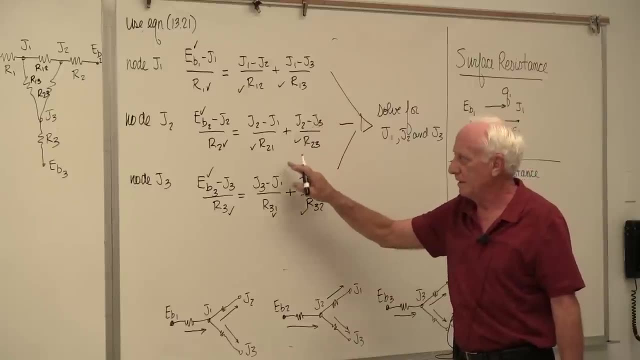 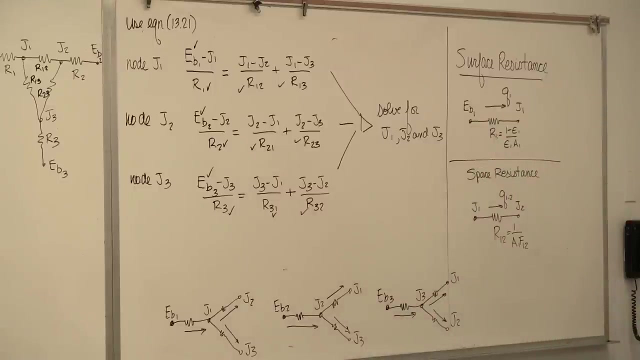 But you got them. If somebody says what's Q1?? There it is. What's Q2, 3?? There it is. What's Q1, 3?? There it is. So once you know all the Js, you can find any of the Qs in the problem. 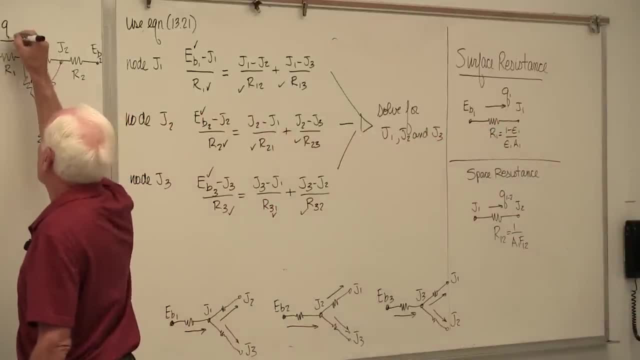 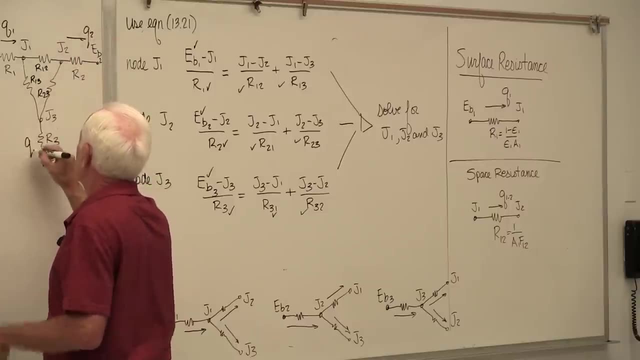 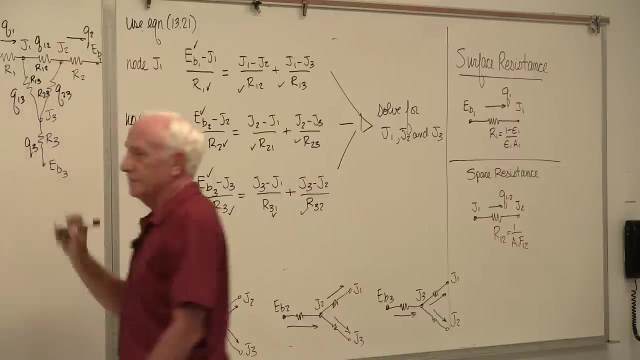 And how many are there again: Q1,, Q2,. I don't know the directions. you'll find out. It depends on Q3,, Q1, 3, Q1, 2, Q2, 3.. There's six of them. 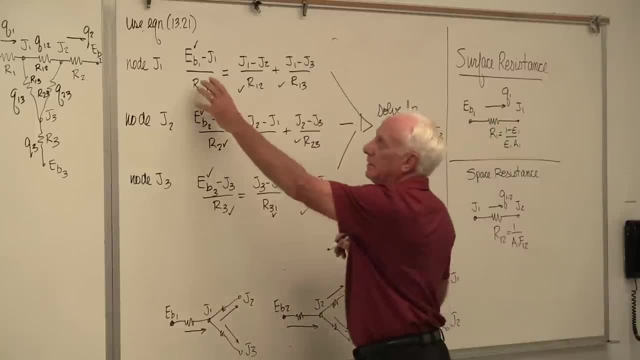 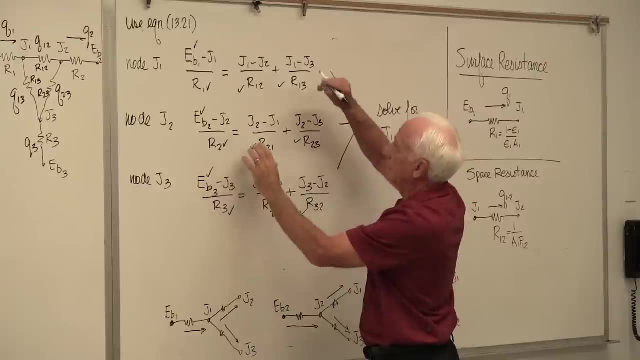 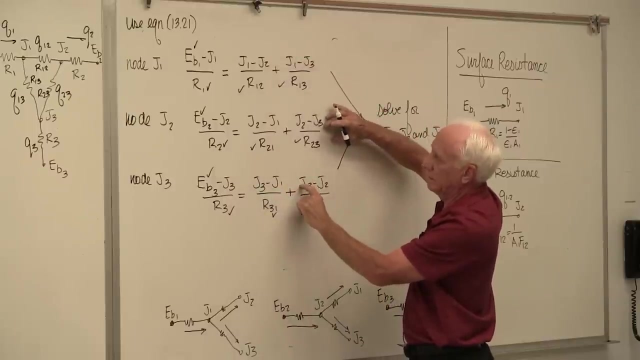 Six of them. You can find them Here's Q1.. Here's Q2.. Here's Q3.. Here's Q1, 2.. Here's Q2, 3.. Here's Q3.. Here's Q3, 1, or Q1, 3.. 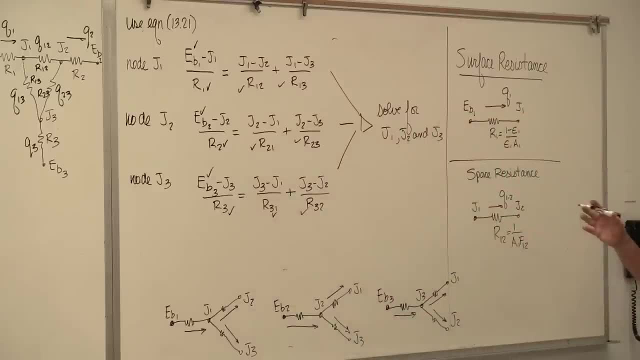 There they are, all the Qs. That's what you want to find typically in a thermal analysis: all the Qs. Okay, So the easy one. all the surfaces are black. Look at the picture, By the way. by the way, just so you know, are there any Js? 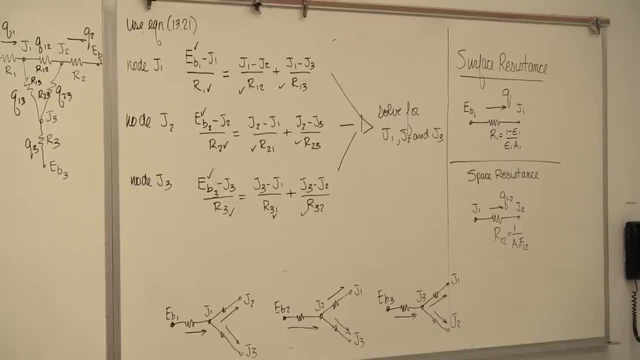 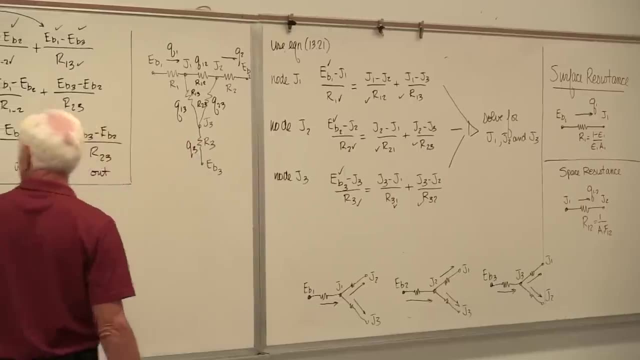 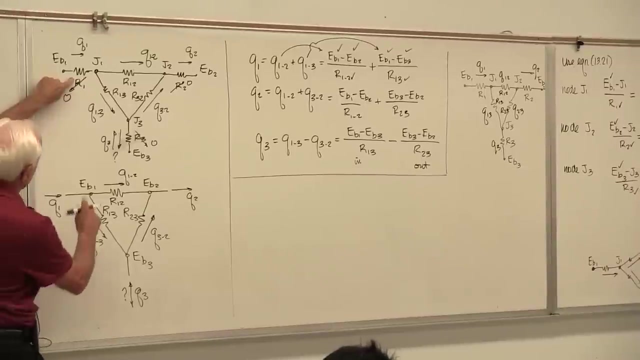 No, there's no Js. When they're not black, are there Js? Oh, yes, They'll be the Js. now the radiosities, They're the unknowns. Okay, Over here, all black, no Js. By the way, when I got rid of that resistor, why did I replace that J1 at that node with? 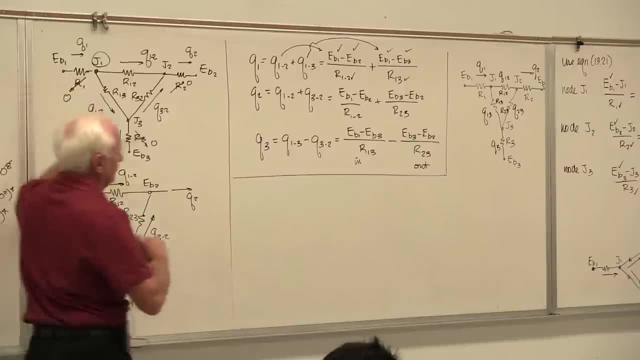 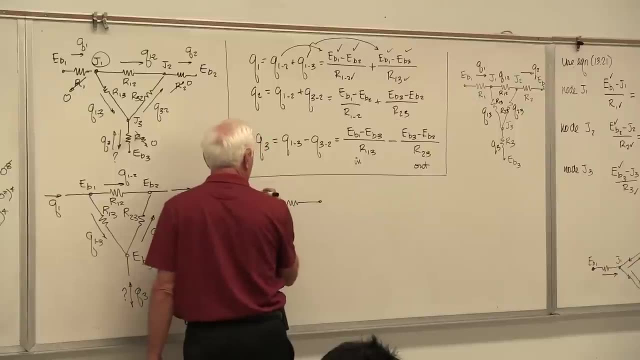 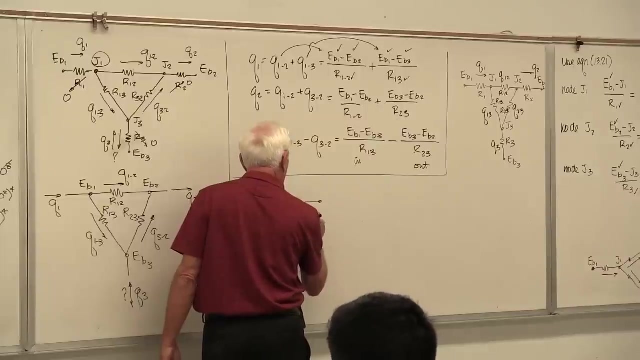 EB1?? Sometimes that confuses people. Well, let's go back and ask you a trick question from simple circuit theory: V1 equal 10 volts. The resistance here equals 10 volts. V2 equal 50 ohms. This is V2.. 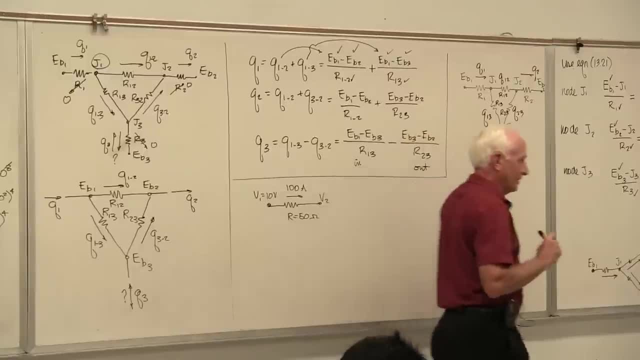 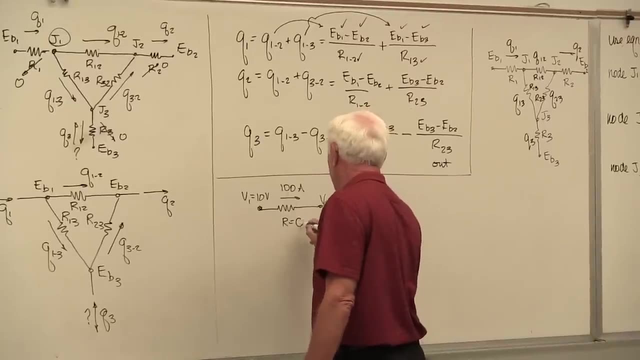 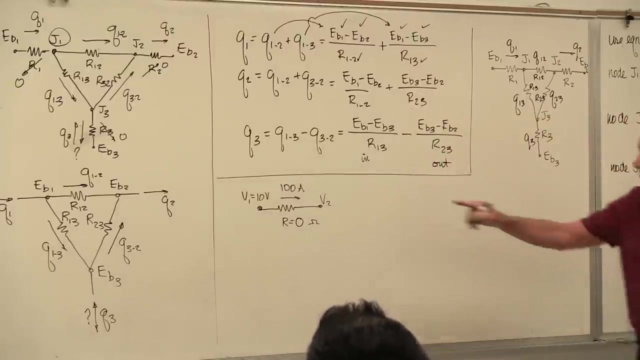 This is 100 amps And somebody tries to trick you and they say, oops, pardon me here, This resistance right here is zero, not 50.. Okay, What is V2?? Now look here, This is like V1.. 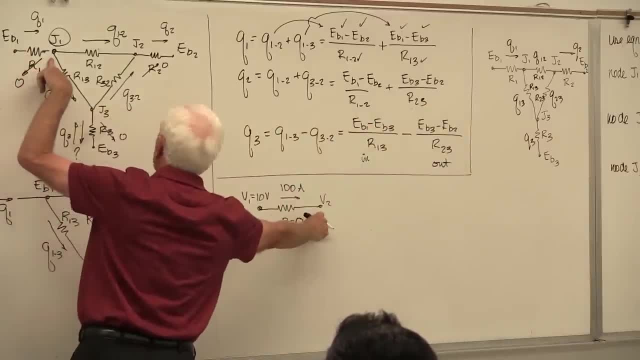 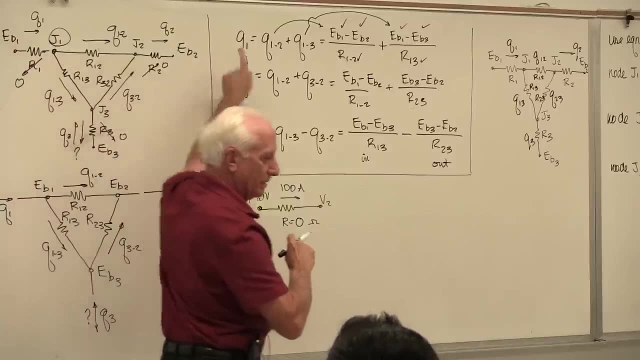 I know it. This is like J1.. I don't know it. The resistance is zero. Yep, Is there a heat flow? Q1?? Of course there is, It's right there. So somebody says: what's V2?? 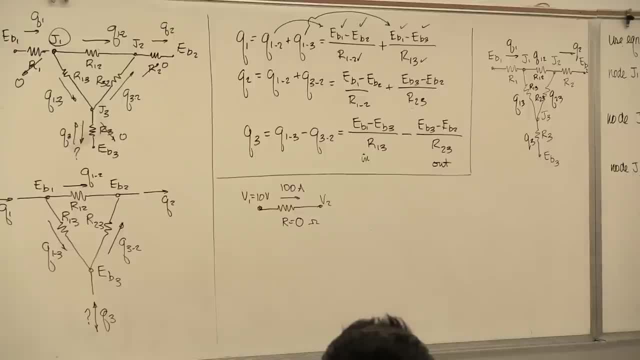 You say: hey, come on, Don't try and kid me. V2 is 10 volts. What else can it be? What else can it be? It's got to be 10 volts. There's no losses. Resistance is losses. 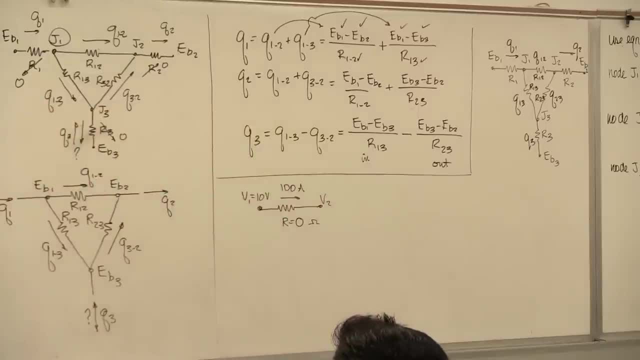 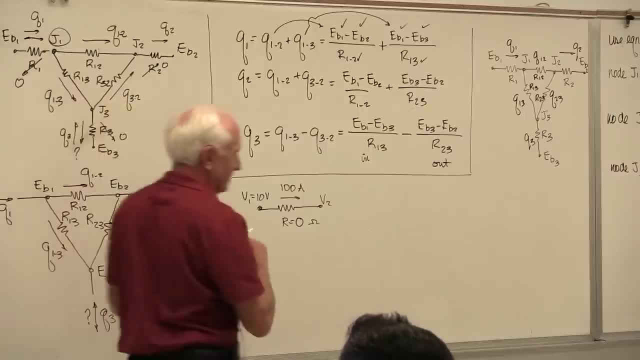 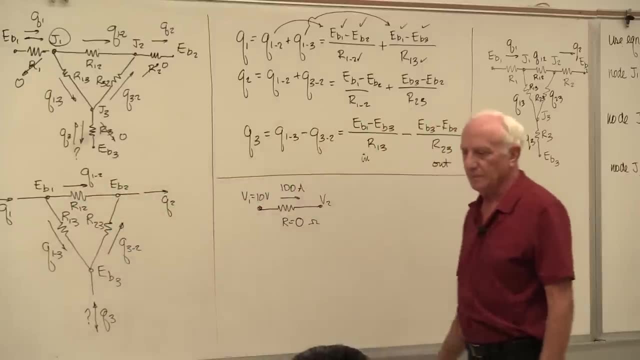 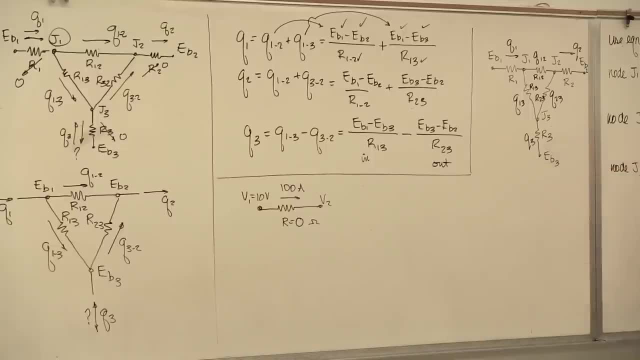 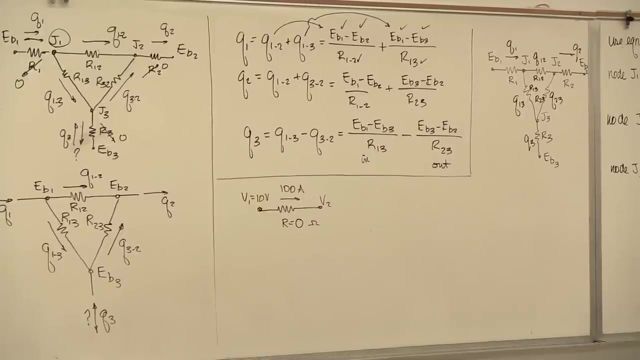 Now comes a tougher problem Here. it is: How do you do it Mathematically this way? Okay, So we've worked two problems so far. Now the third problem: Same picture, Everything's the same, except now I say: you know what? 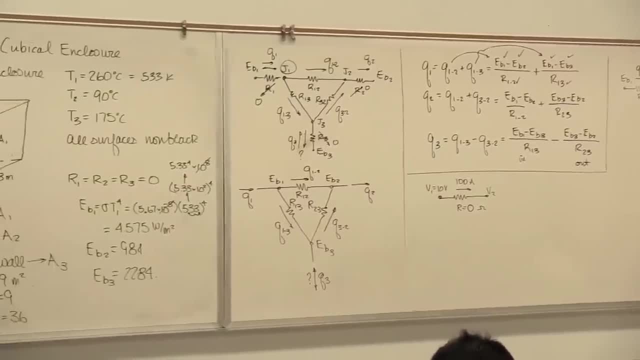 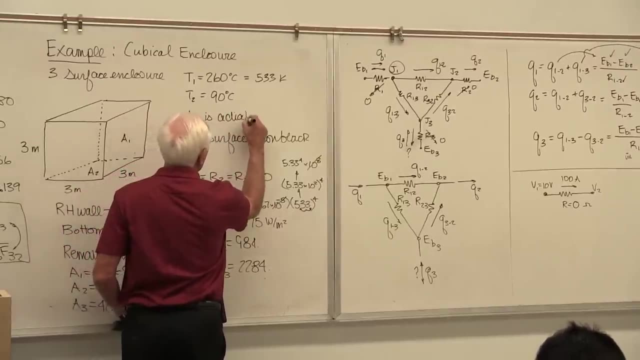 Let's say, 1 is still 260.. Surface 2 is still 90. But now surface 3 is adiabatic, perfectly insulated adiabatic. What does that mean? Well, I know, what adiabatic means. 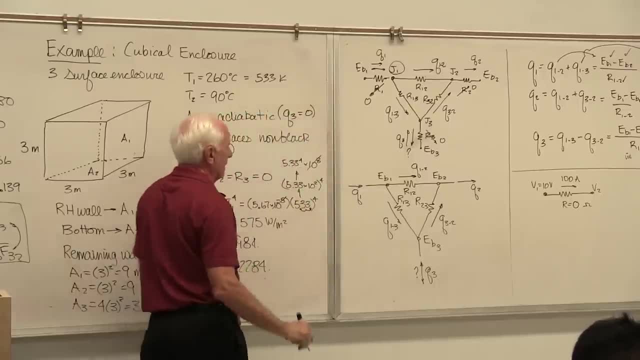 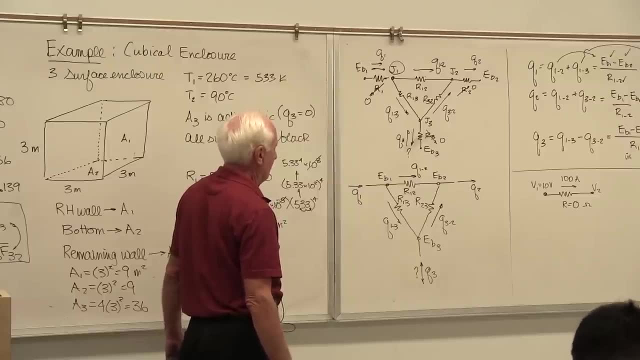 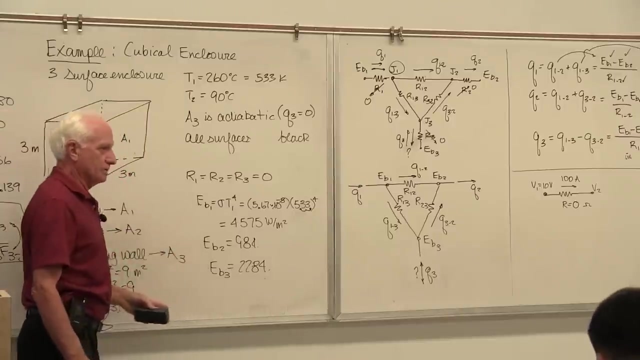 It means Q3 is zero adiabatic. Let's assume that they're all black. Okay, All surface is black. Did the EBs change? Of course not. Did the resistances change of R12,, R13, and R23?? 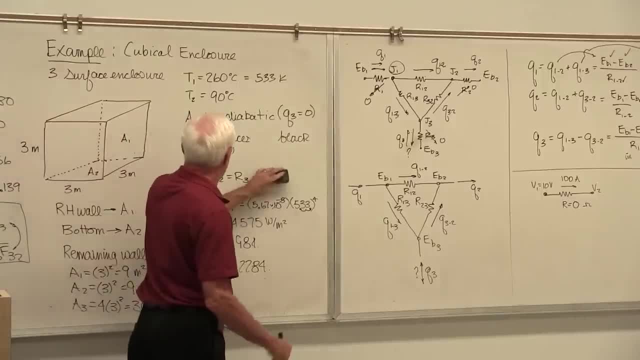 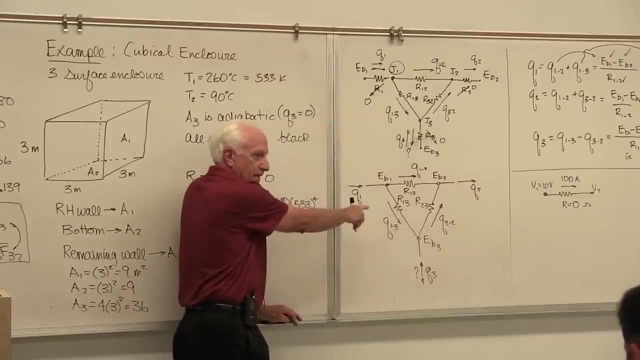 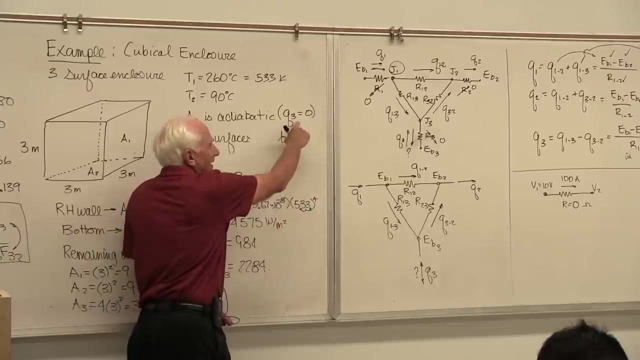 No, Are these guys all zero now? Yeah, They're all black, Okay, Zero, Okay, Here's my picture. now There's my picture. Same picture, you see, Same picture, except for one very important thing: He's zero. 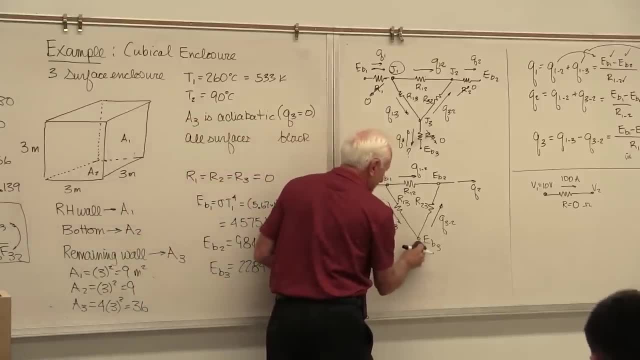 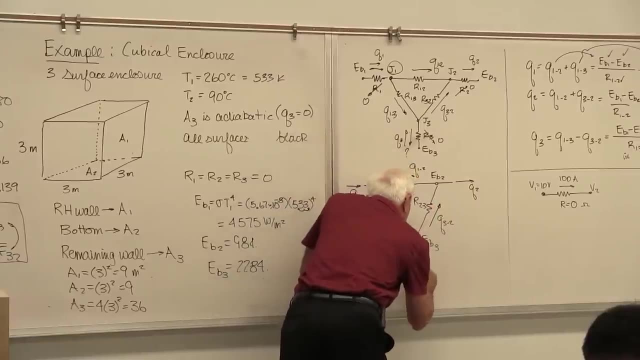 No, He flows that way. So guess what happens When Q13 comes down here. it's equal to Q32.. Okay, Here's a new picture. This is what I say to myself. I say: you know what? Here's how the heat flows. 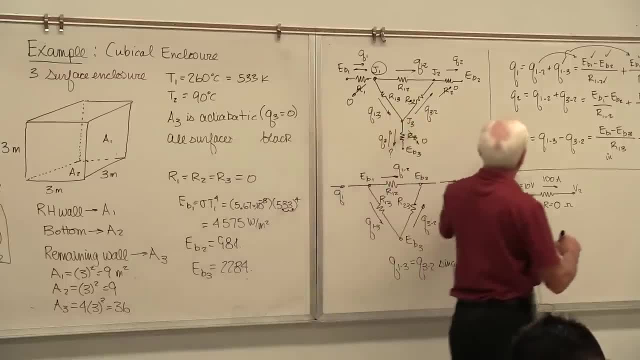 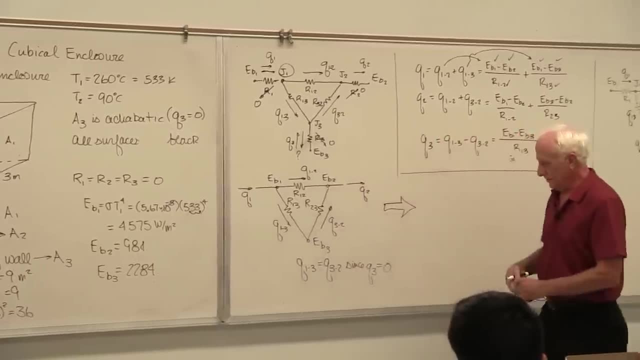 It comes in Q1.. It divides. Some goes down, Some goes straight across. Here comes my fingertips: Uh-oh, Back together. Here comes my fingertips: Uh-oh, Back together, Uh-oh, Back together, Uh-oh. 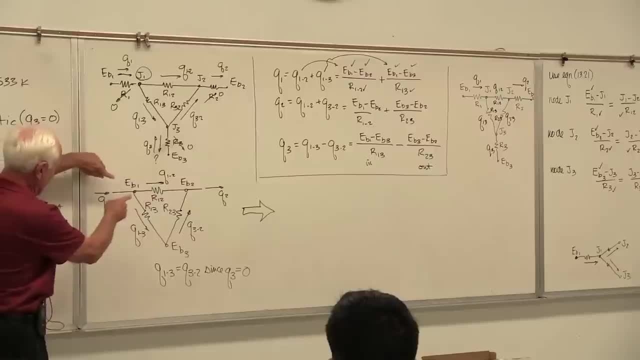 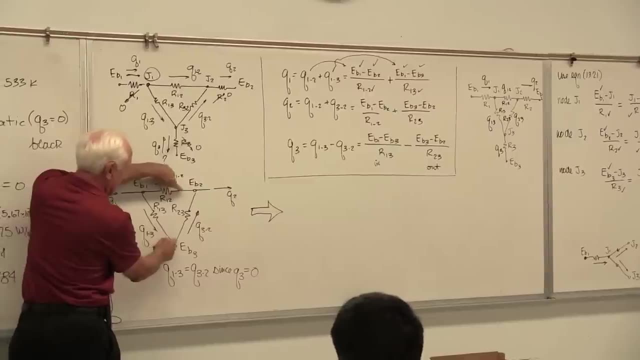 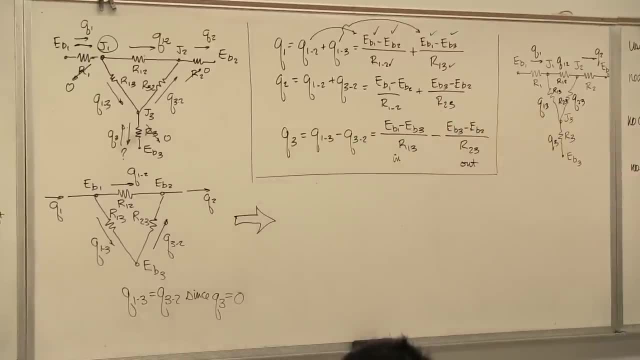 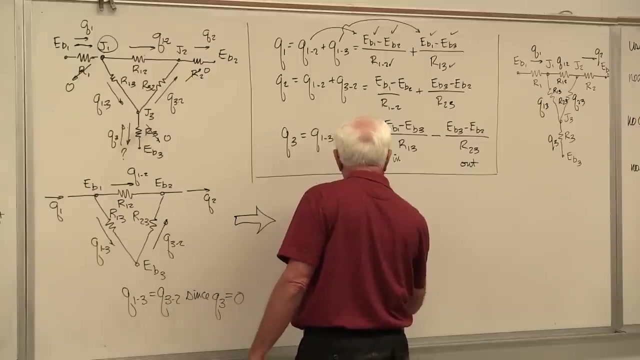 Parallel, parallel. When you do this, they come here, they split, They come back here and go out. That's parallel circuit. All right. So now we have a parallel circuit. Comes in like this: Some goes this way, Some goes this way. 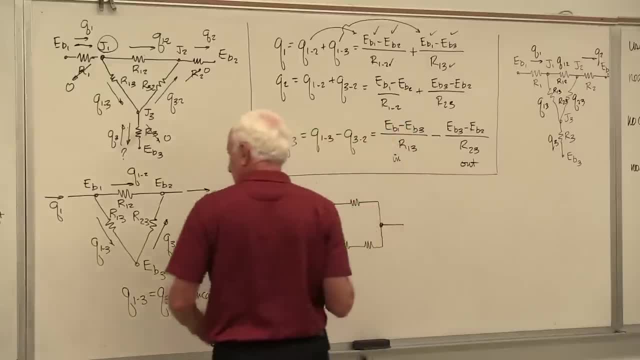 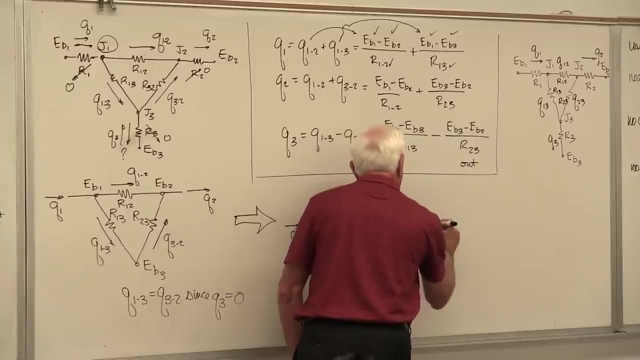 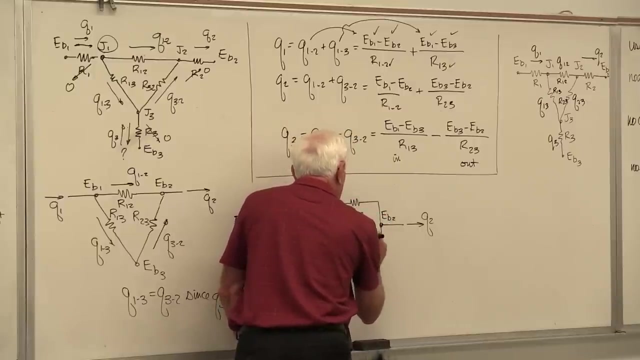 And then it goes back out. Here's the nodes E, B1, H. All right, This is Q1,, this is EB2,, this is Q2,, this is R12,, this is R13,, this is R23,, this is. 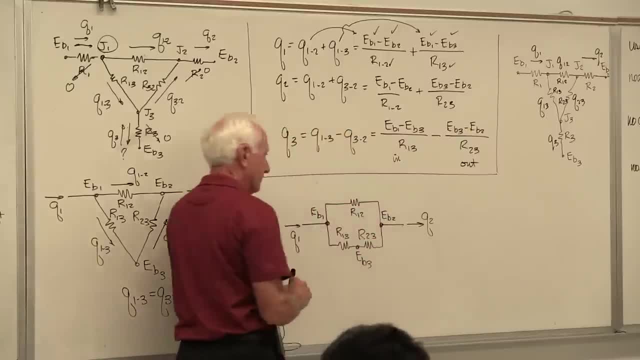 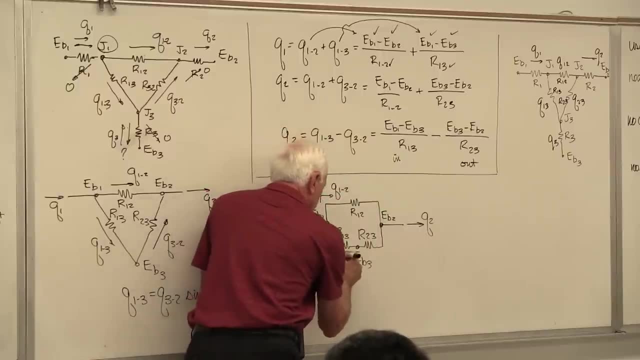 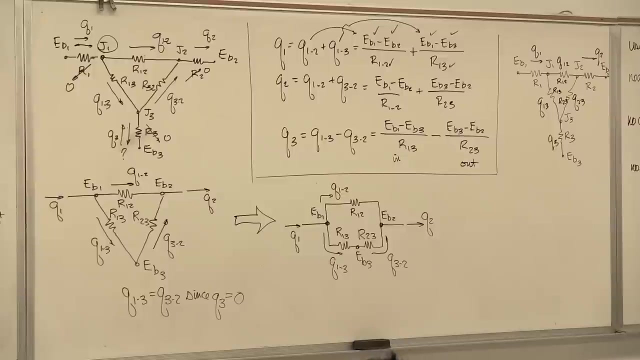 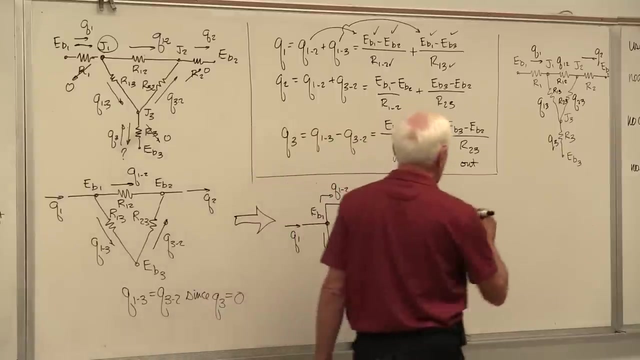 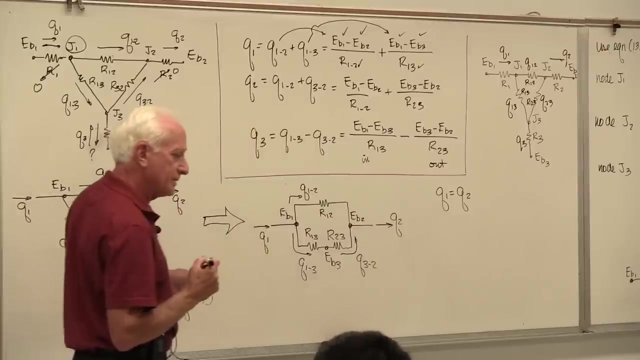 EB3.. This is Q12, this is Q13, this is Q32.. So there's the simple thermal resistance model that you want to work with. It's a parallel circuit? If it is, I can tell right away that Q1 equals Q2.. What comes in must go out, because it can't get out three. it's. 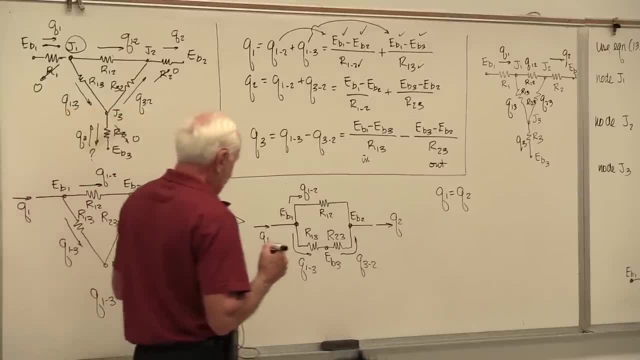 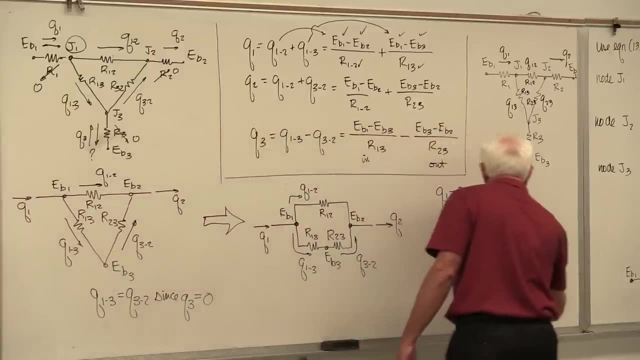 adiabatic. Okay, parallel circuit. you want to find Q1. All right, Q1 equals EB1, the big value minus EB2, the low value Divided by R equivalent. R equivalent for what A parallel circuit? Multiply the two. 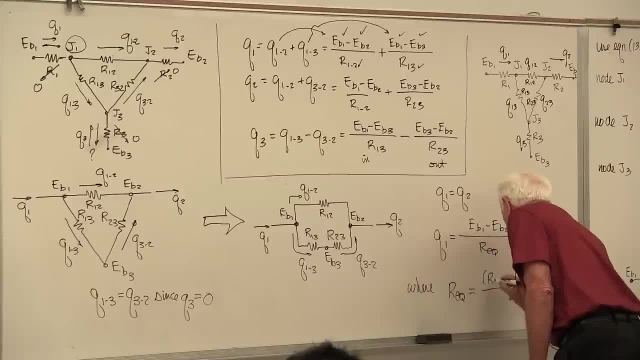 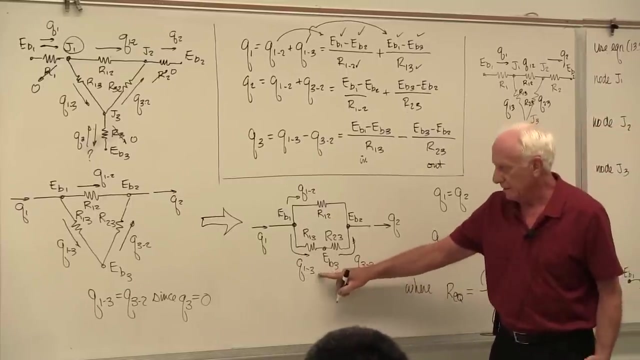 branch resistances together, Divided by the sum of all the resistances in the two branches. Okay, Got it. I know every value there. I can find Q1,. I can find Q2.. If you want to find Q13,, 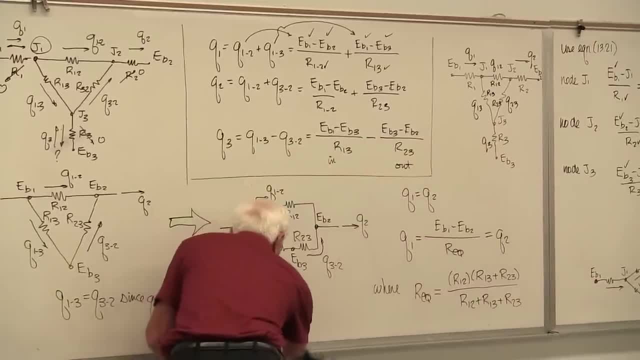 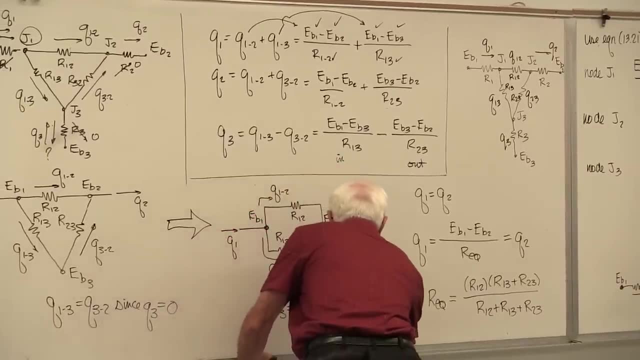 it's equal to. I'll put it down here: Q13 is the same as Q32.. That's equal to EB1, minus EB3 divided by R13.. I know EB1,, I know EB3,, I know R13.. I got it. That's Q13.. I can find. 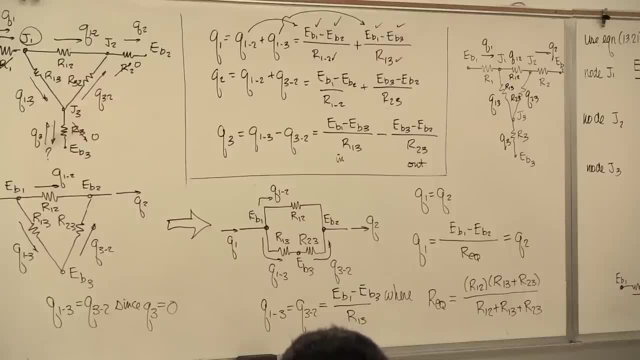 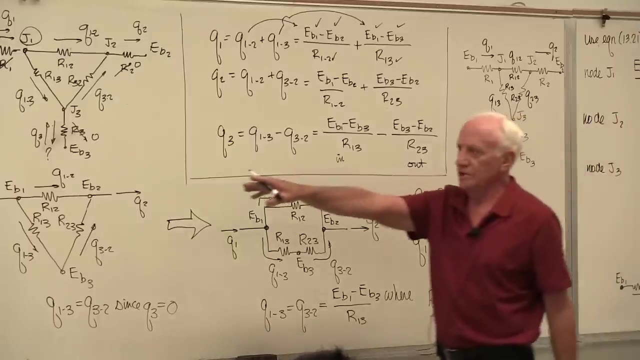 any Q term You want me to. There are six of them: Q1, Q2, Q3.. Q12,, Q13, Q23.. I can find all six. Do I see a J anywhere? Nope, Why not? The surfaces are all black. J is not. 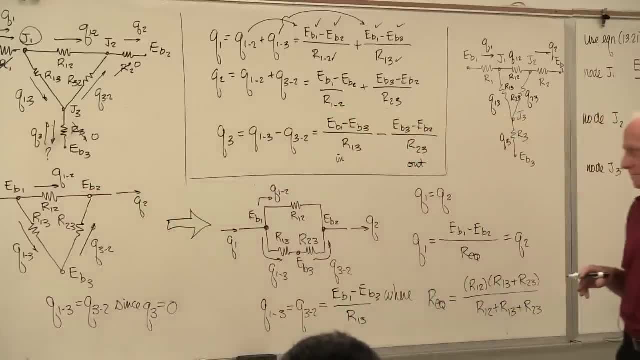 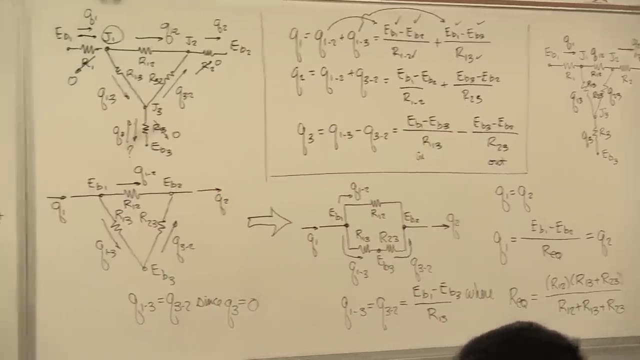 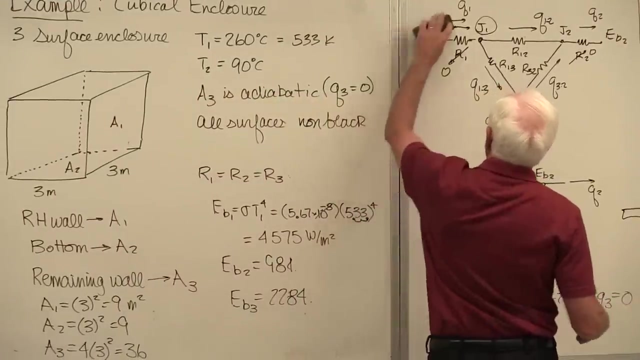 going to come in this problem. We've worked three problems now. Now comes the fourth one. You know what's left. All right. This was when all the surfaces were black. Now all the surfaces are non-black. None of the resistances are zero. Leave them all in there, All right. 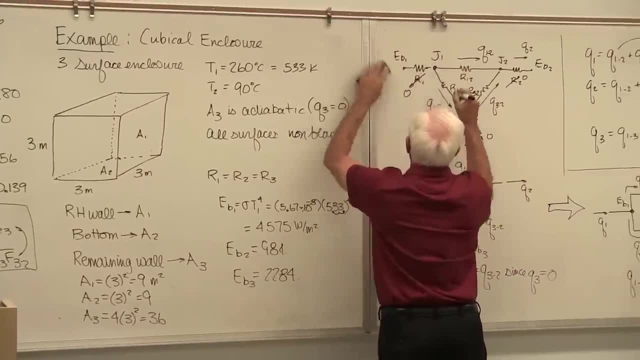 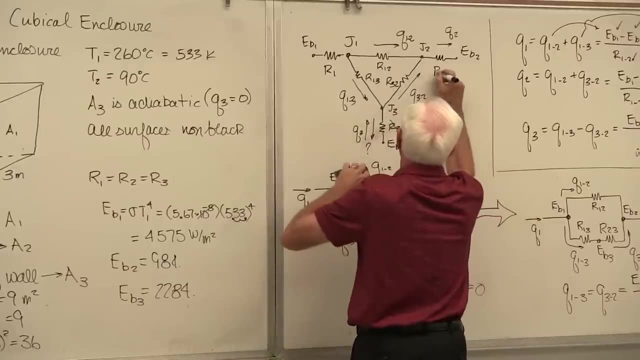 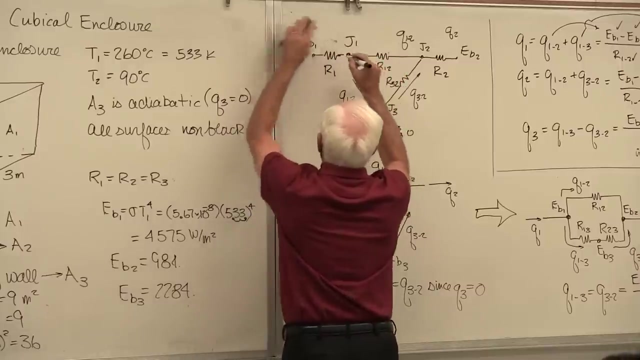 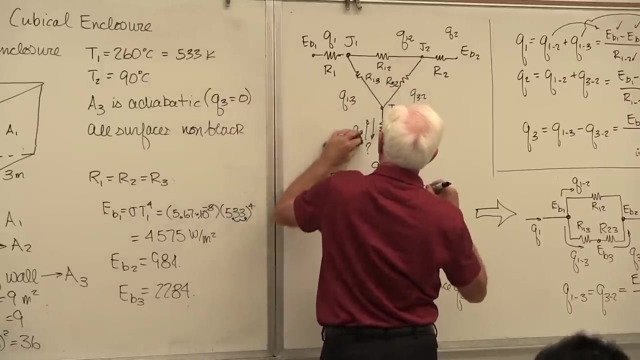 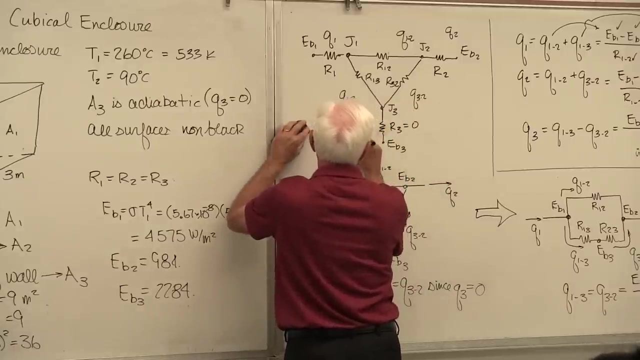 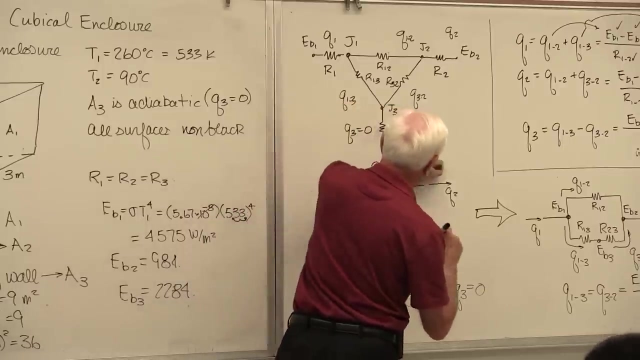 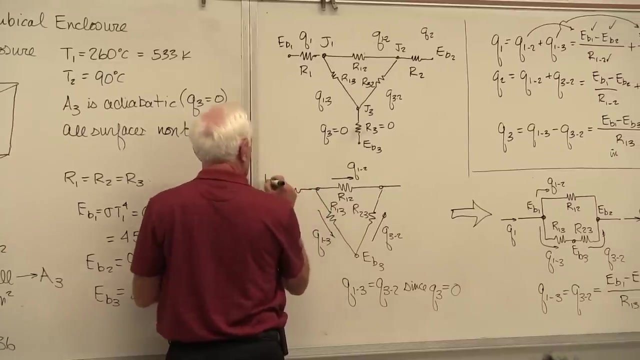 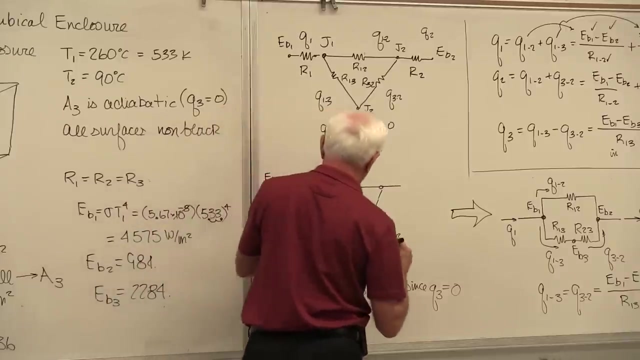 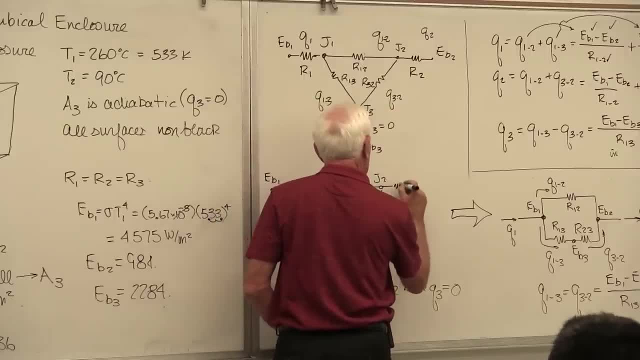 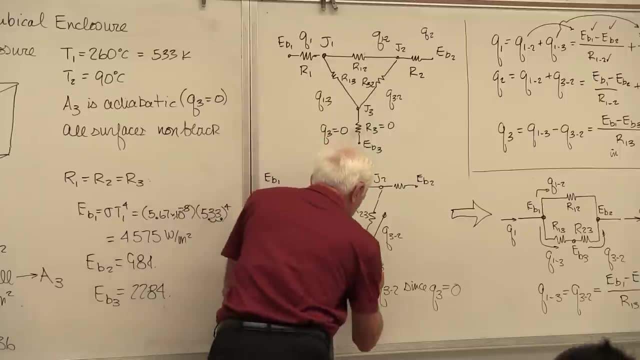 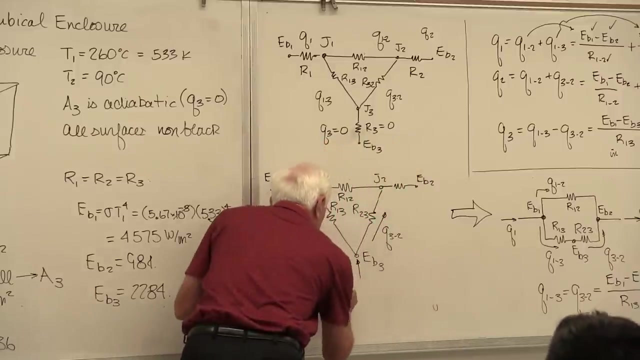 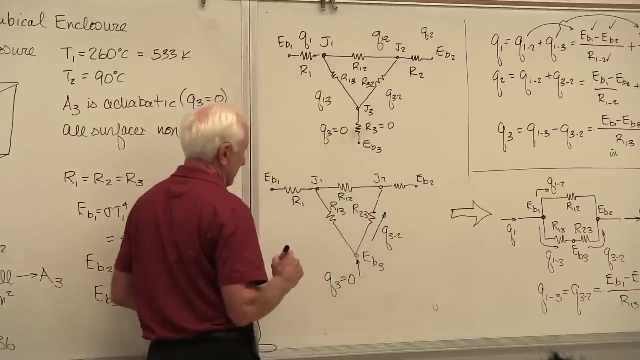 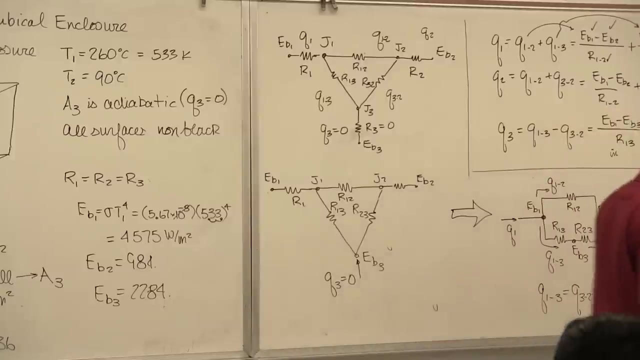 Okay, Okay. Okay, there's the picture. now. Assume I don't know which way those cues are going up. We're going to again assume we don't know which way the cues go In this simple problem like this. we pretty much do, but we're going to play the game. 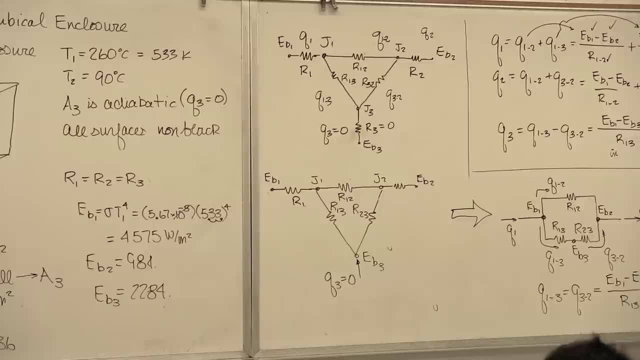 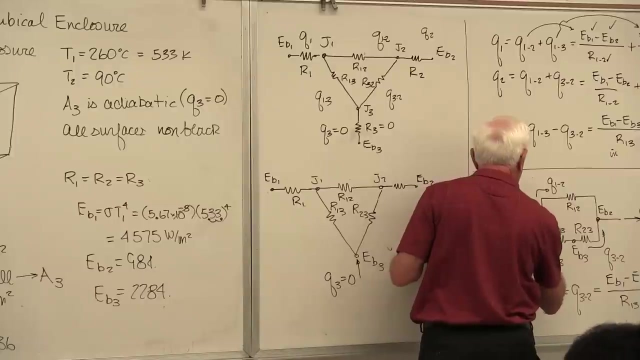 of using the equations 13,, 21, and pretend we don't know which way the cues go. okay, If you want to do it by this method, you can. All you do is you put a resistor here, R1.. 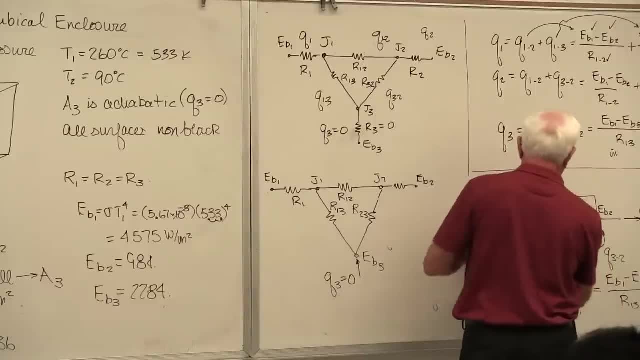 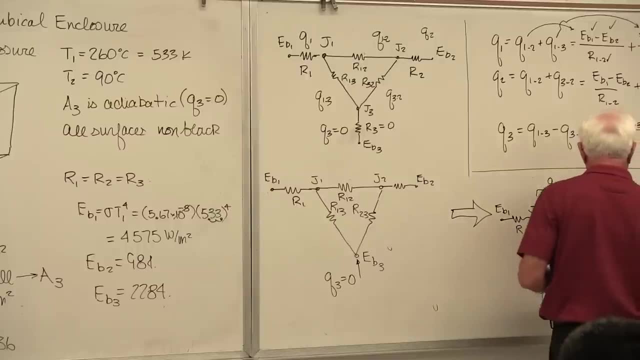 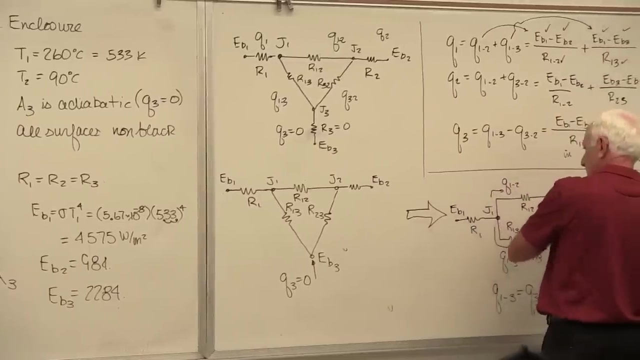 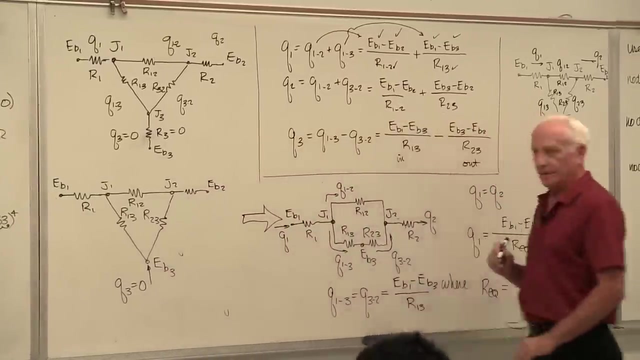 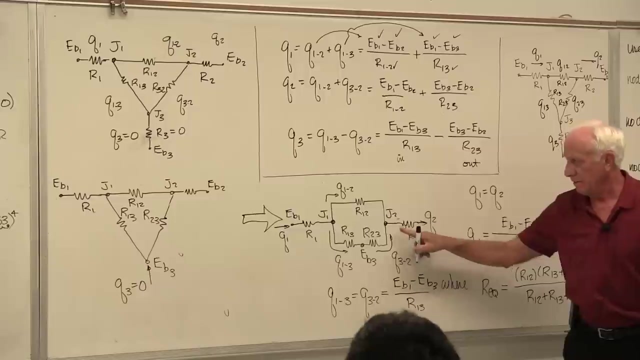 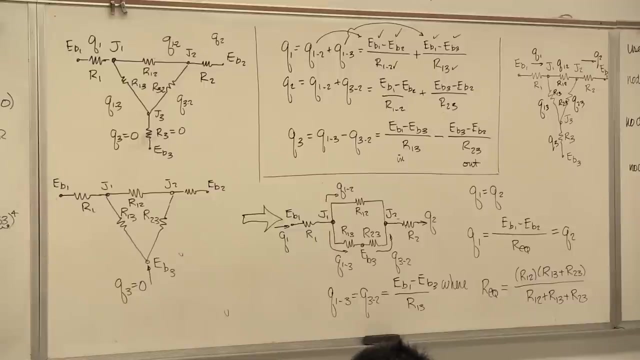 EB1, J1, J2, R2, Q2.. Now it becomes a series parallel circuit. Series Parallel circuit. Simple to solve, Not a problem. Do it very easily. But we're going to show you how you can also use the equations besides looking at solving. 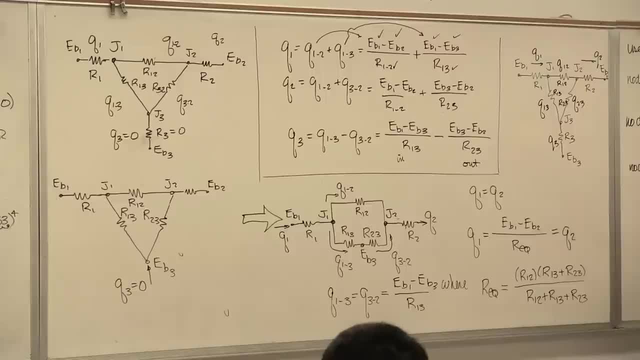 it with the graphical picture of what's going on the thermal resistance network. Okay, But you can do it by looking at this simple picture here and doing a series parallel circuit. You know, all you've got is two more resistors here. 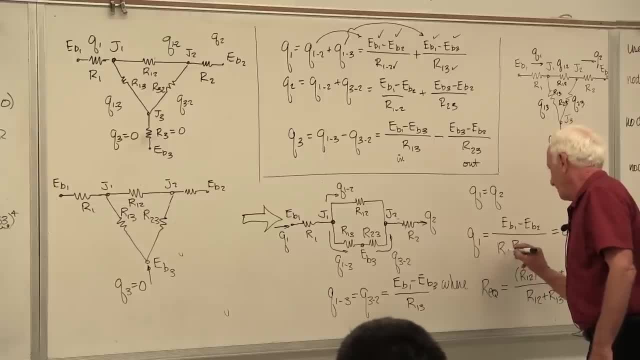 We'll go ahead and do it: R1 plus this plus R2.. There's the answer right now. That's all you do. Very simple, Series parallel. Okay, But when you do this kind of problem for your computer problem For homework, there's going to be six surfaces. 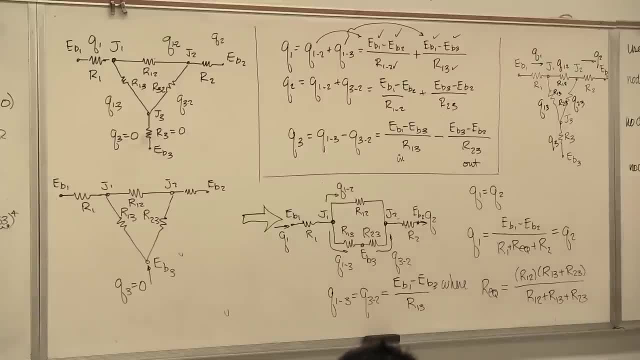 You don't want to do it this way. No, It's a bear, You know. Don't do it this way. You're going to do it this way and have equations to solve For what unknowns The J's. Where are the J's? 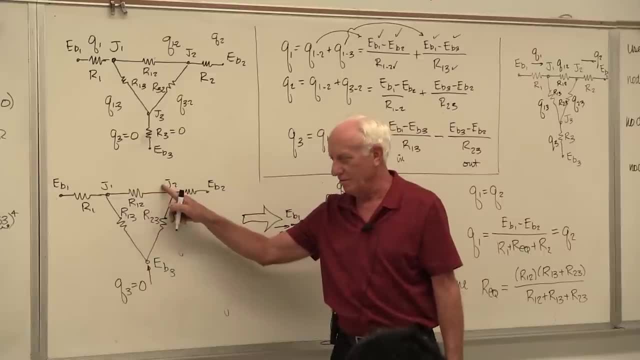 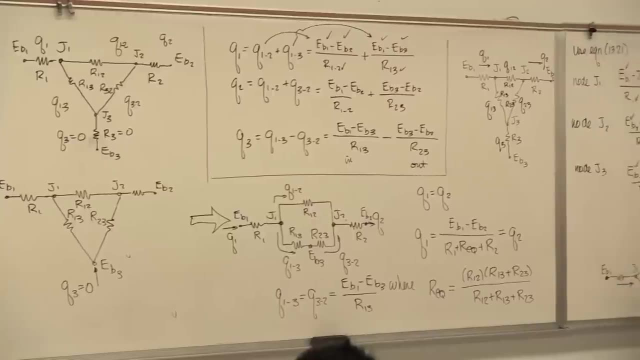 There they are: J1, J2.. Do I know them? No, All right, Node J1.. Here's the rule again: When you write the nodal equation, what comes into the node J1 from the surface is EB1 minus. 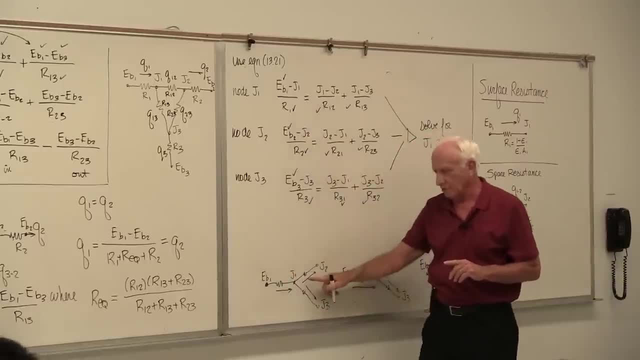 J1 divided by R1.. There Equals what goes out J1 minus J2 divided by R1, 2.. Yeah, Plus what goes out J1 minus J3 divided by R1, 3.. There Got it. 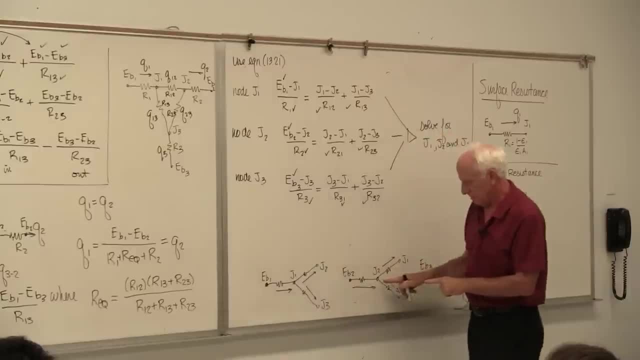 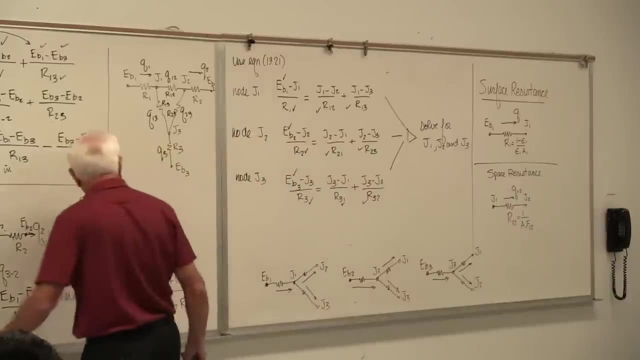 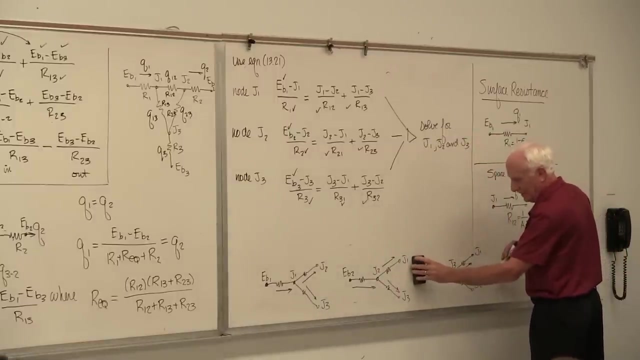 That checks Node J2.. Here it is Same thing. This equals this plus this. We've done it before. Now here comes a change. Node 3 no longer looks like this. Uh-uh, Node 3 has something that looks like this: 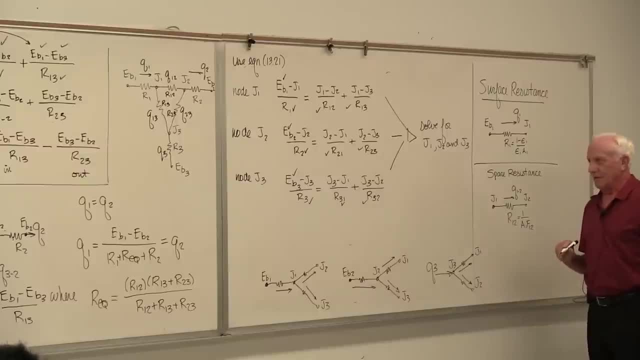 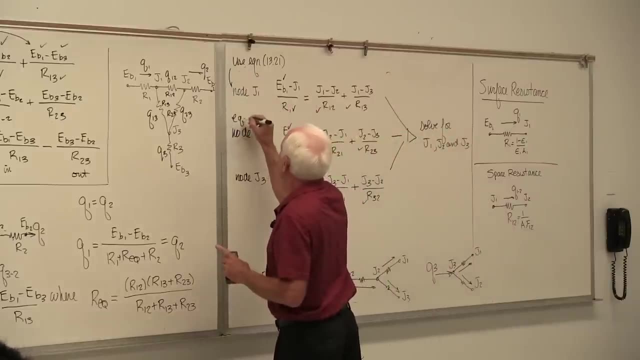 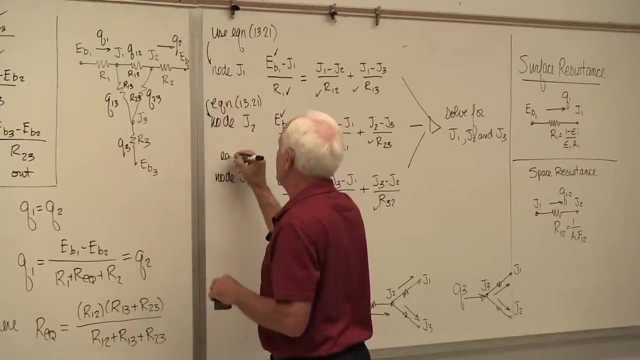 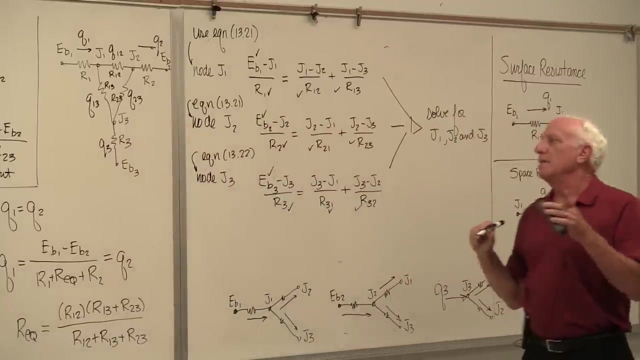 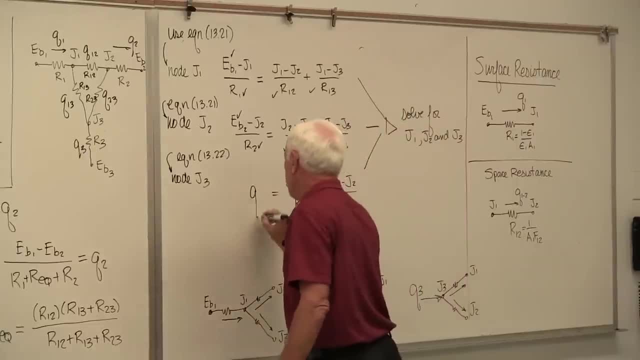 1322.. You don't use this anymore. You do this. If a node has a specified heat flux or a heat transfer, then that's the equation you want to use. What did our problem say? Our problem said: surfaces 3 are adiabatic, which 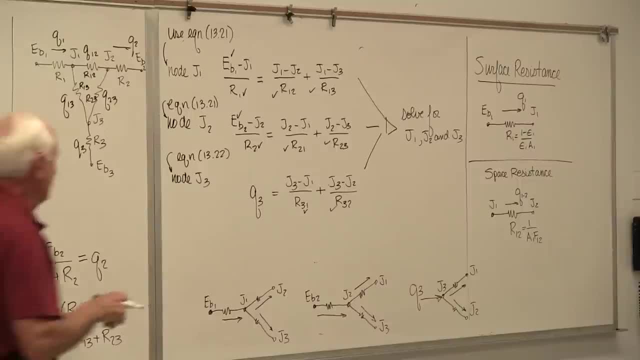 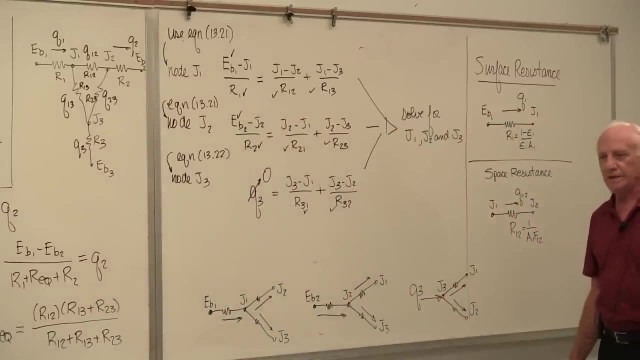 means Q3 is 0. So now we put the 0 over here. Okay, there they are Three equations, linear, simultaneous. whatever method you want to do, Solve for what? again, You don't need J3, because I know J3. How do I know J3?? Look at the picture. 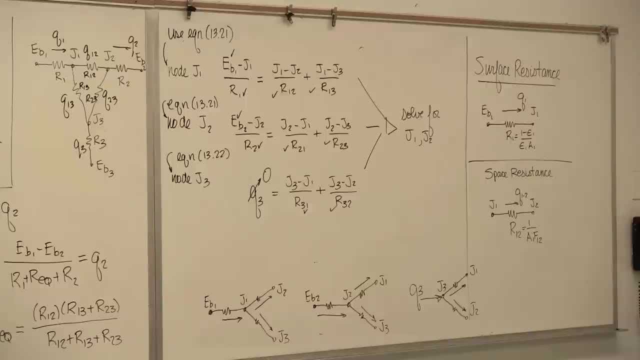 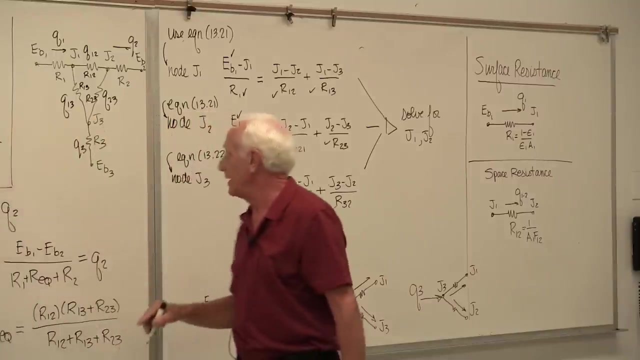 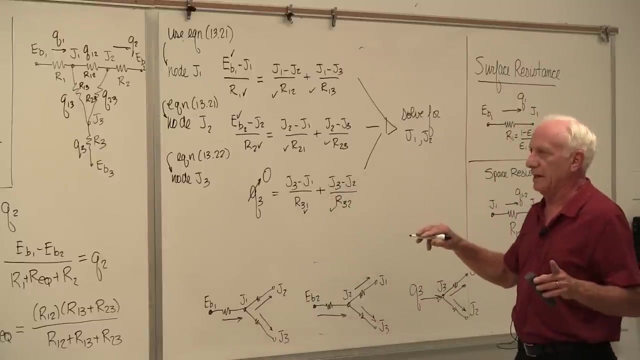 J3 equal EB3, because there is no. by the way, those are black surfaces. It was non-black, looks like that. If Q is 0, then I know that J3 equal EB3.. Okay, so I know, I know that. Okay, got them all. Now what do I do with them? All? right, how? 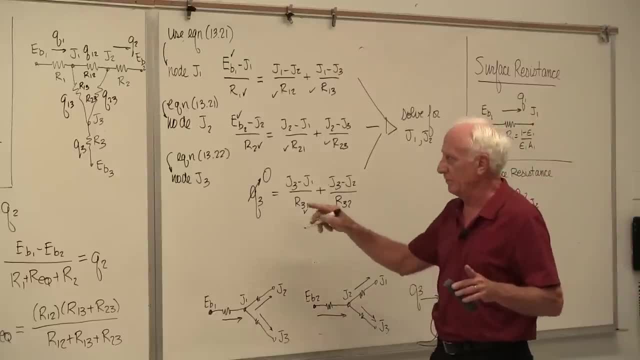 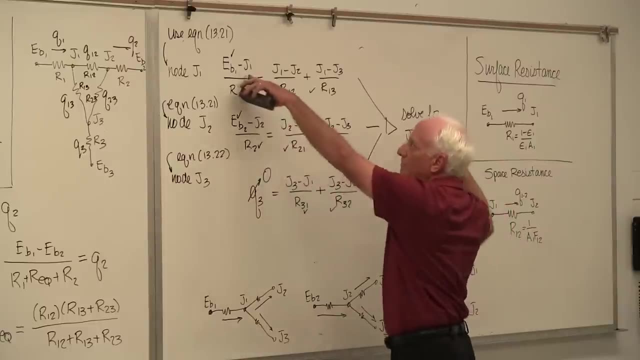 many J? how many Q's are there? There's six. Let's do the easy one first. Q3 is 0.. Okay, Okay, good, I want Q1.. There it is. I put J1 from there into there. I know R1.. I. 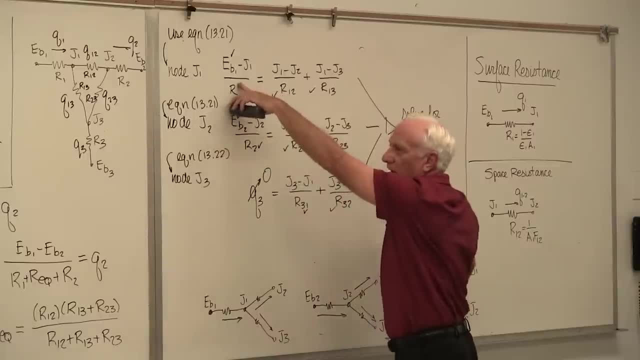 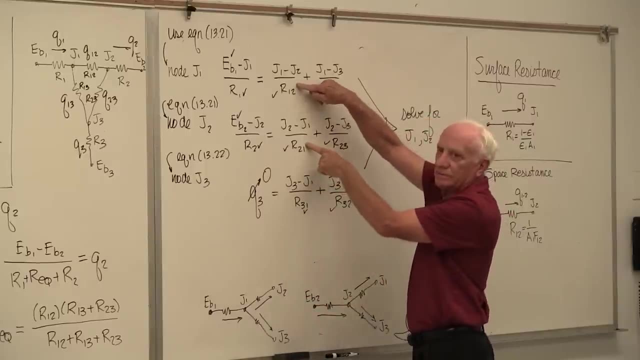 know EB1.. They're over there, I solve it. Q1.. I want Q2.. There it is. I want Q12.. Take your choice Now. watch the sign. If J1 is bigger than J2, that means he goes. 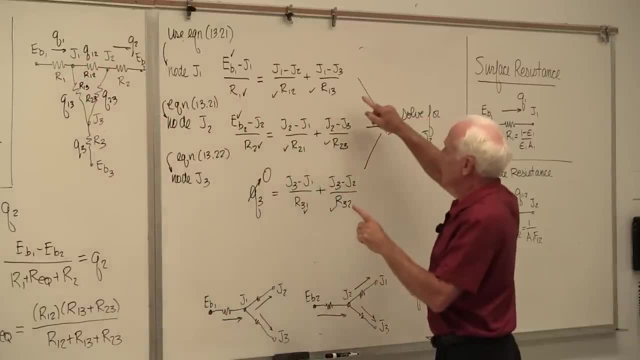 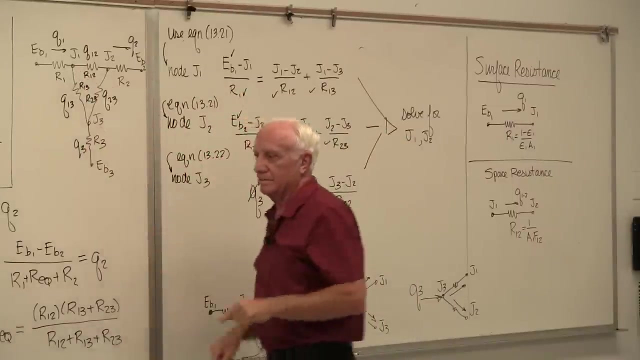 from J1 to J2.. Now J13. If, if J3 is greater than J1, J3 greater than J1, then heat flows that way. So by looking at that you can tell, comparing the J's, you can tell. now, 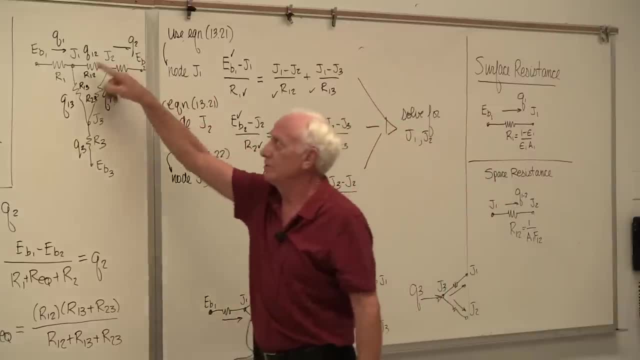 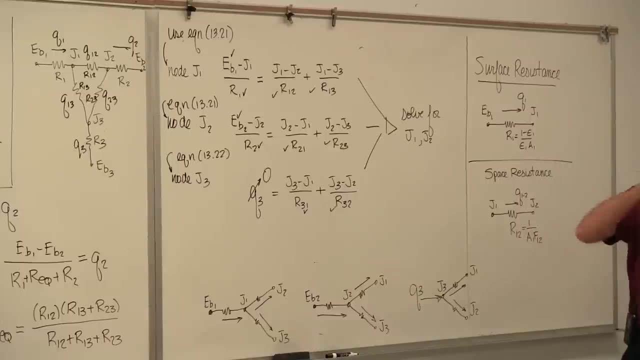 which way the heat flows. The heat flows from the high J value to the low J value, Not so important in a in a three-surface enclosure, But it's important to know about a six-surface enclosure. this room, Oh yeah, That helps dramatically, You want. 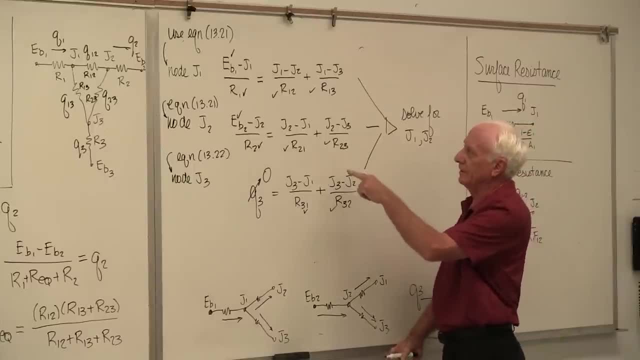 Q23.. There it is Q23.. Two, three, Right there. This is Q32.. Same thing, One sign's negative, One sign's positive. So what have you found? Six Q's Done, You're done, That's it So. 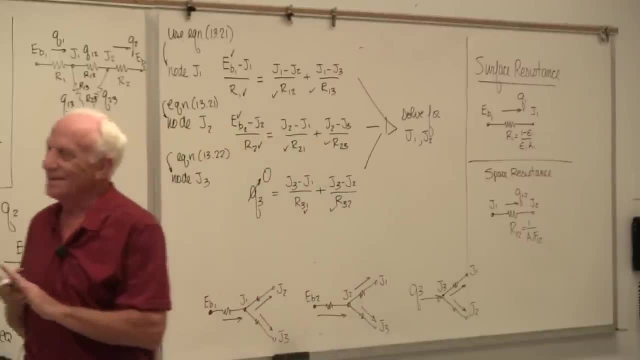 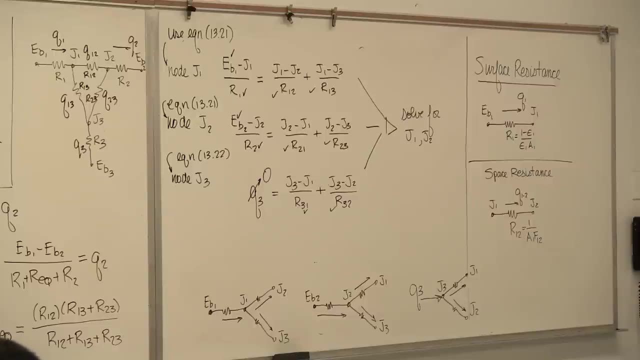 you write the equations like that. So that's our fourth problem. now Okay, First just to review. The first problem was: I know all three T's, Three temperatures: T1, T2, and T3.. All surfaces are black. I showed you how to solve it Next. 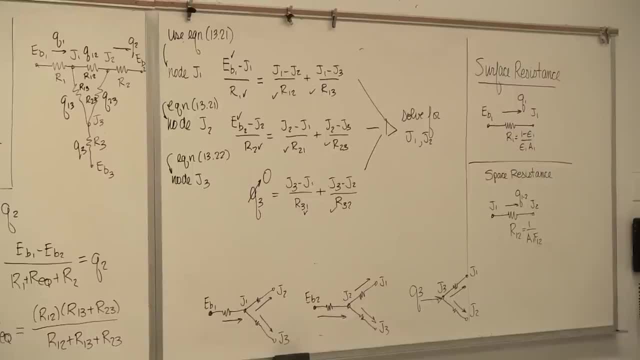 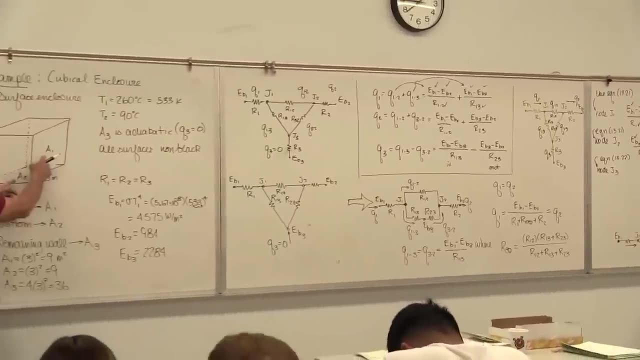 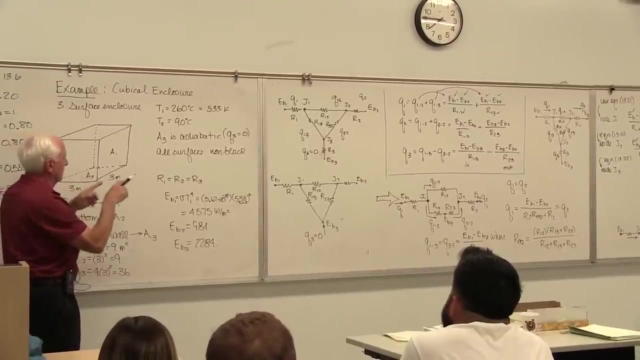 problem: Three surfaces, Three known temperatures, But they're not black. We solved it. Next thing: Two surfaces known temperature, Other surfaces adiabatic- Okay, All black, We did it. The last one: Two surface temperatures given, One surface adiabatic, Non-black. 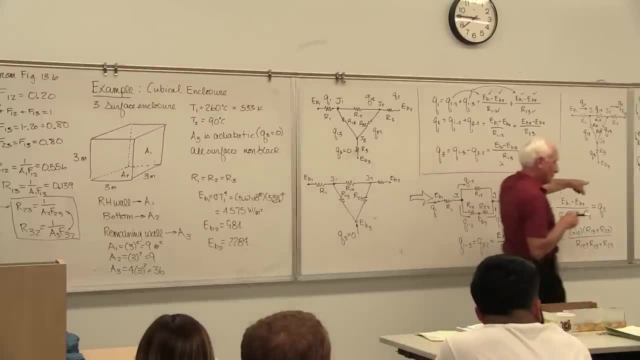 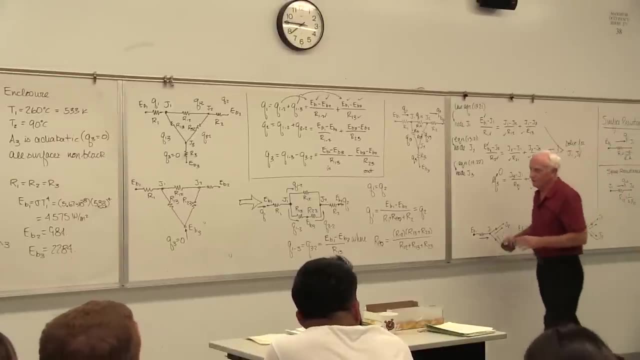 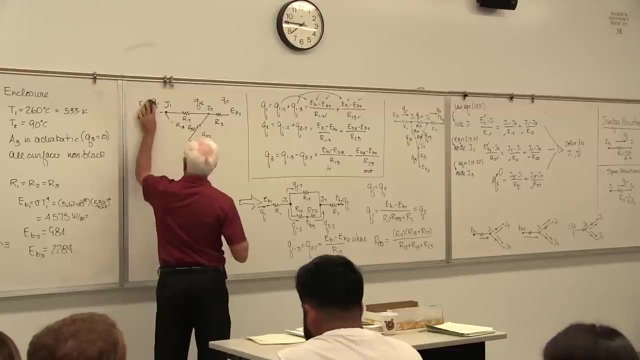 There, it is right here, And there's not much more you can do in a three surface enclosure. I just about covered everything on that. Now here's what you don't want to do. Let's take this room where there are six different surfaces. Maybe temperatures are known on a couple of 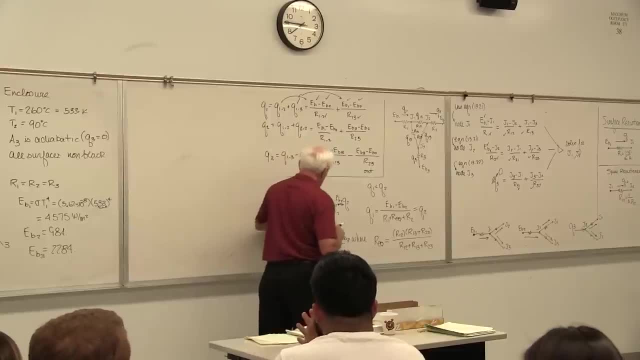 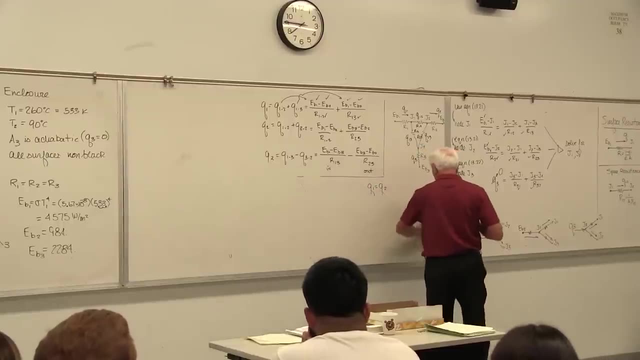 them, Many of them. Maybe Q is given, Maybe it says the heat into surface one is 1,000 watts. What does that mean? Well, that means that outside this box, outside this box, there might be some electrical heating elements on this outside surface. And then these guys. 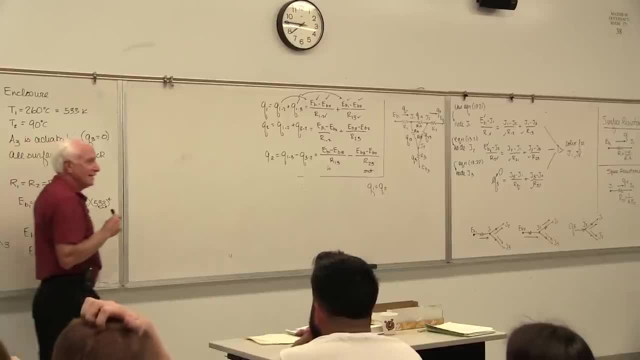 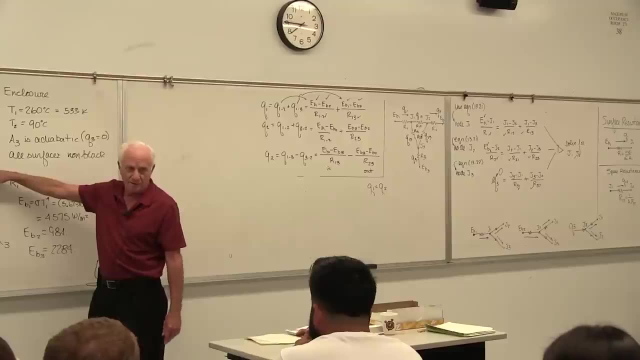 go to some kind of voltage supply and they heat the outside the box. If somebody tells you that they're heating this with electrical wires, they put out a 1,000 watts and it's insulated on the top of that. then That 1,000 watts has to go into that box. That is going. 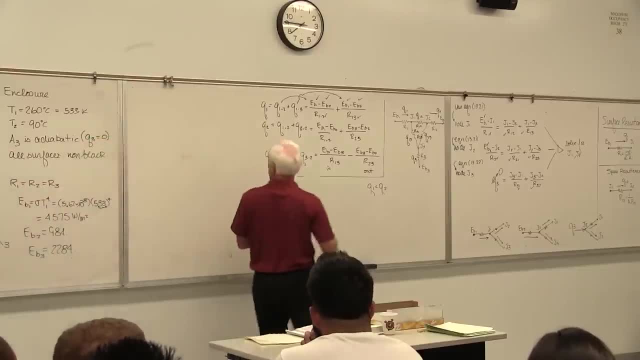 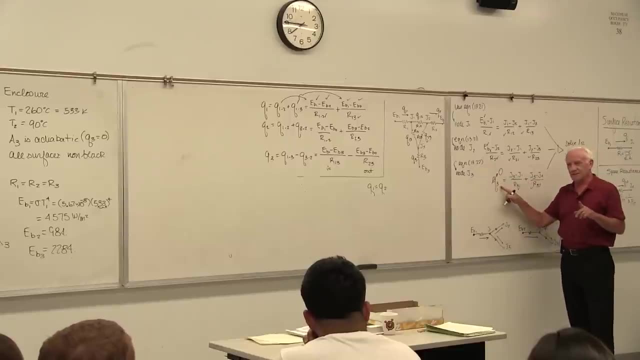 in the box, in the enclosure. Okay, That's my Q, That's my Q1.. Now I know Q1.. Q1 is 1,000. So I use equation 1322. Where I see Q1, I put 1,000. That's a known heat rate, a known 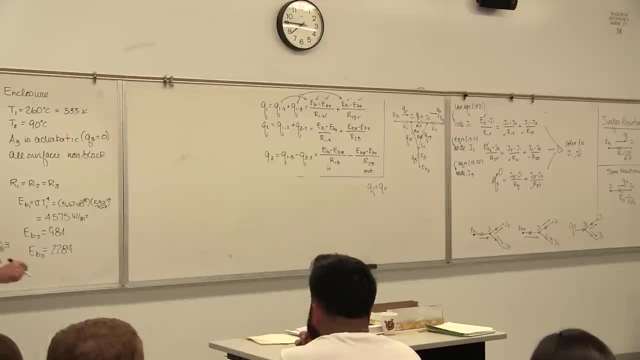 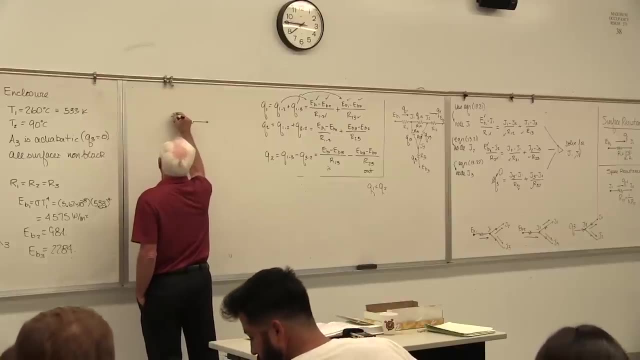 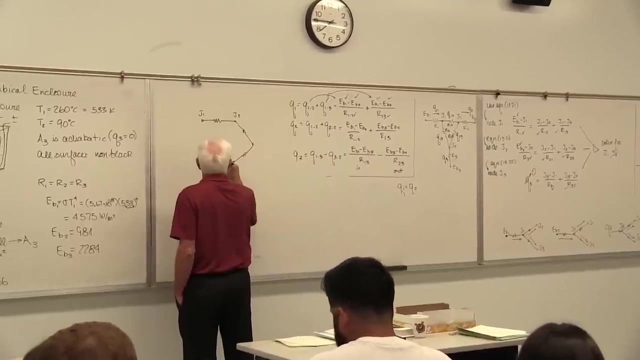 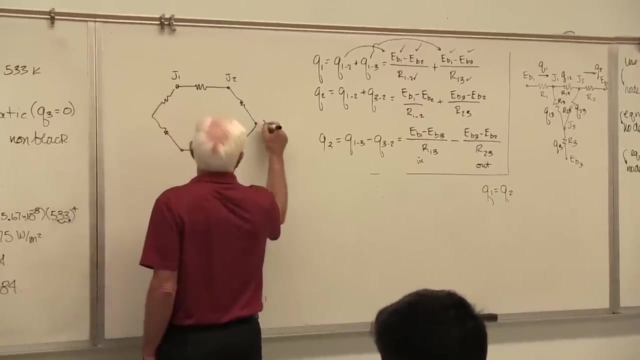 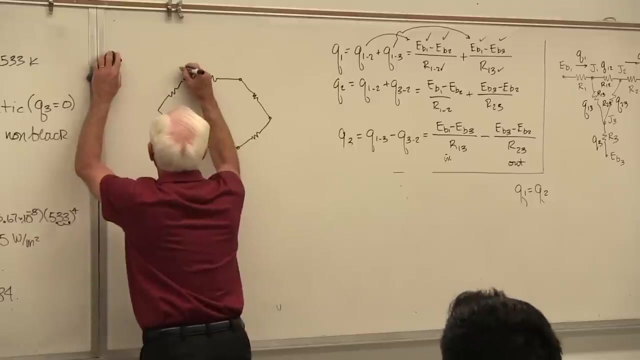 heat rate. Okay, So let's say that you're doing this room with the six, Okay, So here we have: this is J1, this is J2, J3, I better change that. This is J1, EB1, J1, this is. 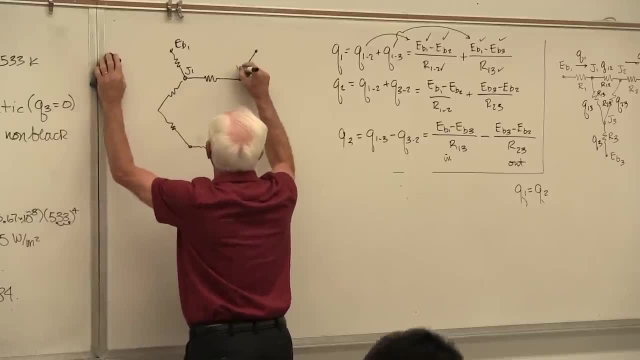 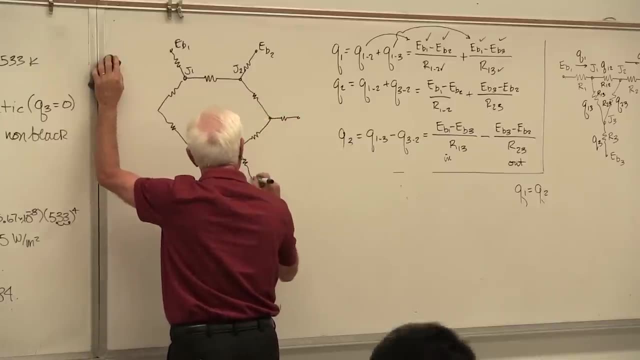 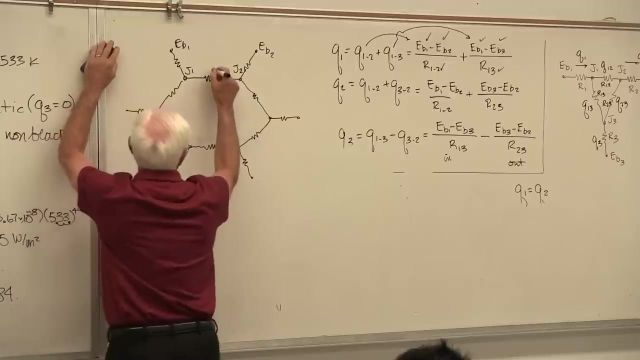 E, B2,, J2, and so on, and so on, and so on. Three, four, five, six. This is R12.. This is R16.. This is R13,, R14,, R15.. This is R21.. 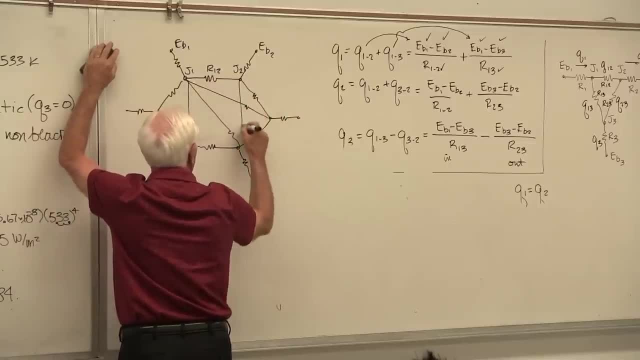 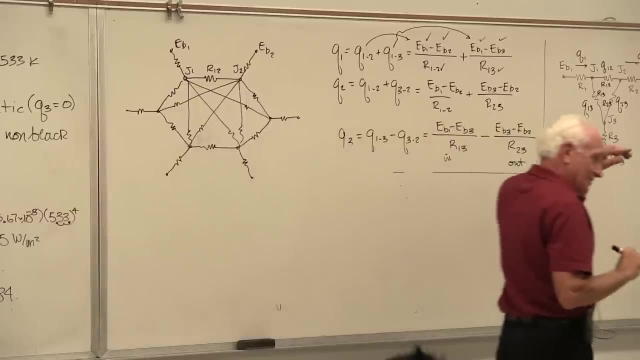 This is R23.. This is R24.. This is R25.. This is R26.. Oh, you keep going. Looks like somebody's built a plate of spaghetti on the floor. You think, oh my gosh, what's going on? 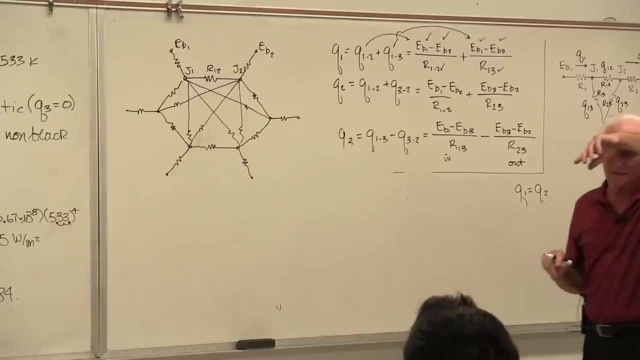 Which way is the heat flowing there? This is really confusing to me. I don't see what's going on here. You're right, which means that this approach of the equivalence, the equivalent network, doesn't work very well for more than three surfaces. 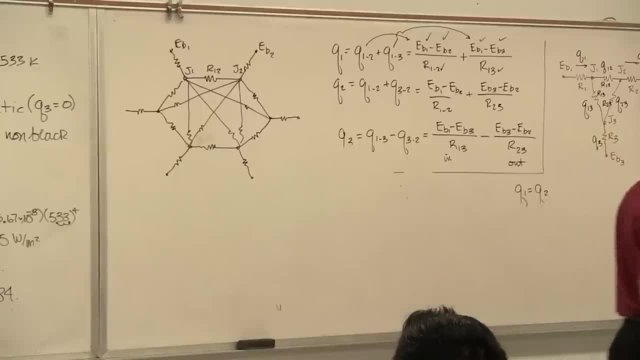 It gets too confusing. It's not worth too much. Then what do you do? Fall back on the math, because it's not going to fail you. There they are. There they are. Now you can do it. Draw a new picture. 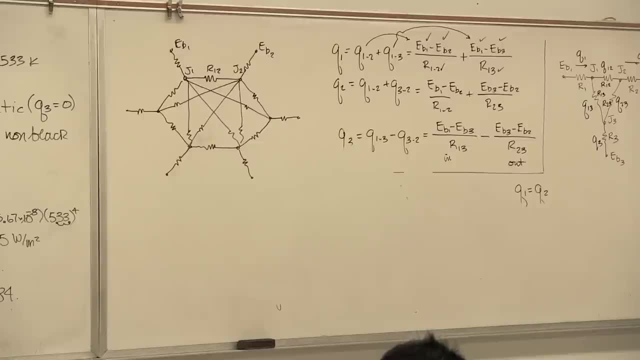 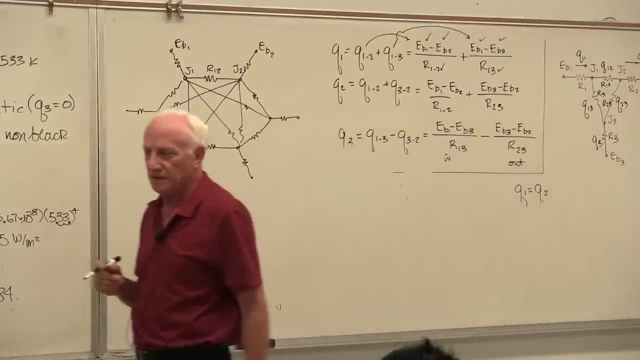 E, B1 to J1 to J2 to J3 to J4 to J5 to J6.. Bam, done deal. Write the equation, Write all six of them. Solve, Solve, Solve, Solve, Solve, Solve them simultaneously. for what? 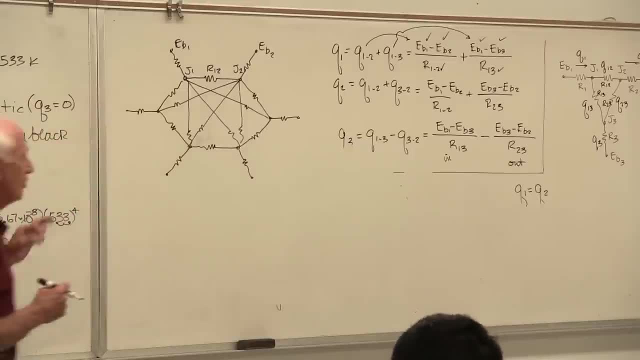 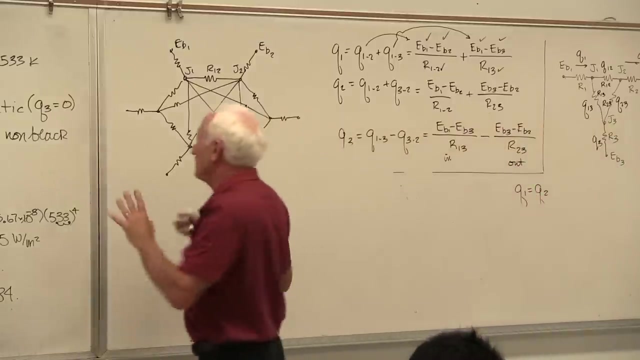 The Js. Once you get the Js, then what do you do? You put them in the Q equations. Here's Q1, Q12, Q13, Q2, Q3, Q32.. Put the Js in, Done, Okay, so we don't use these circuits. 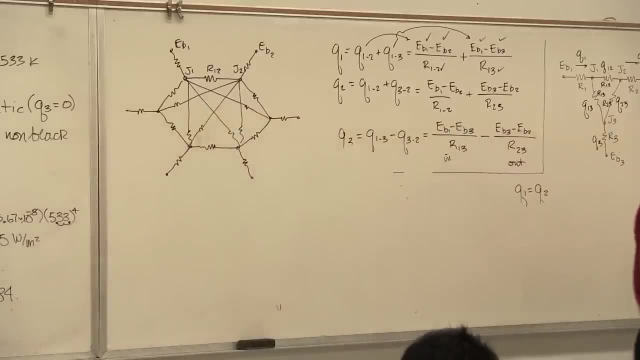 for any more than three surfaces And it's more to give you a visual graphic feel for the problem. if it helps you that way, That's all it is. It sometimes helps people to see for three surfaces how the heat might be flowing, But when you try and draw this, it's pretty much worthless.